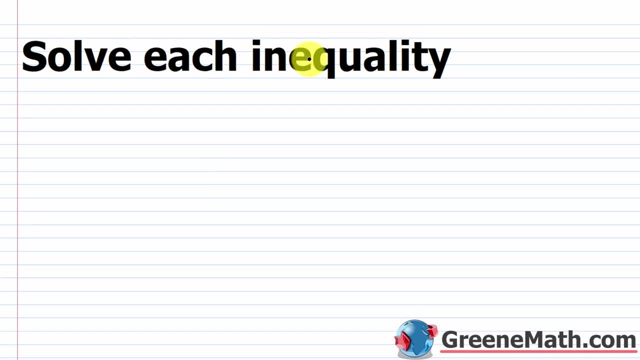 Let's take a look at our practice tests. We're told to solve each inequality And for problem one we have the square root of negative one minus six. x is greater than the square root of three x plus eight. I'm going to tell you in advance: for the problems today I'm going to use a method that is: 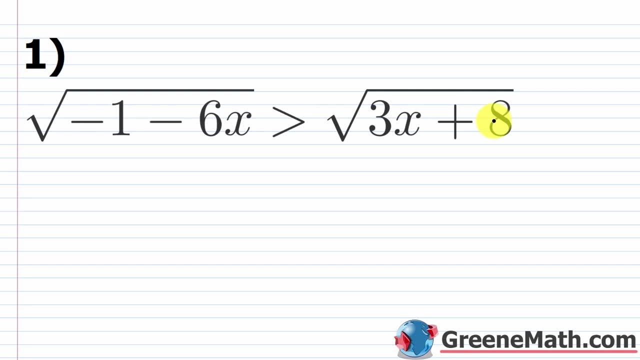 not the fastest, but it will always give you the right answer, no matter how complex the inequality is that you're working with. The idea here is that if you square both sides of an inequality, you'll sometimes get these problems, And just to give you a little insight with a simple example, 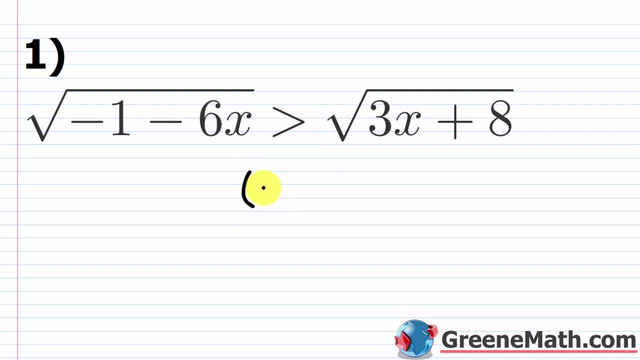 and not to go too far into it. let's just say we had something like negative five, And this is less than, let's say, two. So right now we know that this is a true statement. But what happens if I square both sides of this inequality? this left side would now be 25.. Let's keep the less than if we. 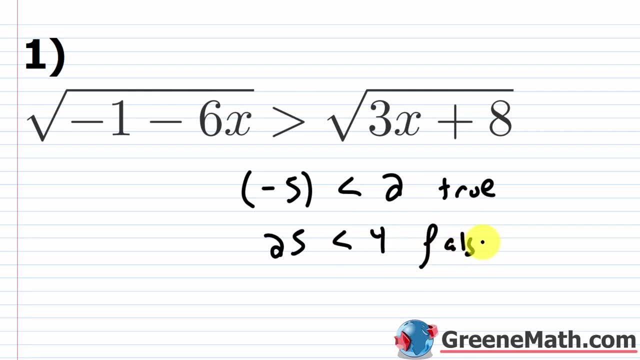 square two, we get four. Well, this is obviously a false statement now. So this is a simple example of some issues that can come up when you square both sides of an inequality. So to avoid this, what I'm going to do, 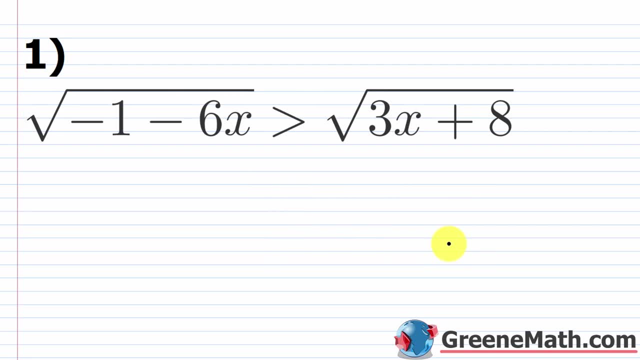 is work with the related equation and just test on each side of the solution of that. So what we'll do first is actually find our domain, because that's going to be important. And just a note here: we are working in the real number system unless otherwise instructed on your test. So when 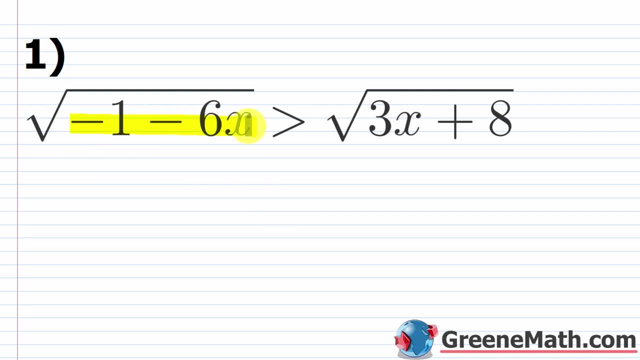 the real number system. we know that our radicand has to be non negative, so greater than or equal to zero. So you have one there and one there. So what you'd have to do is set up a compound inequality with and and say that negative one minus six x is greater than or equal to zero. 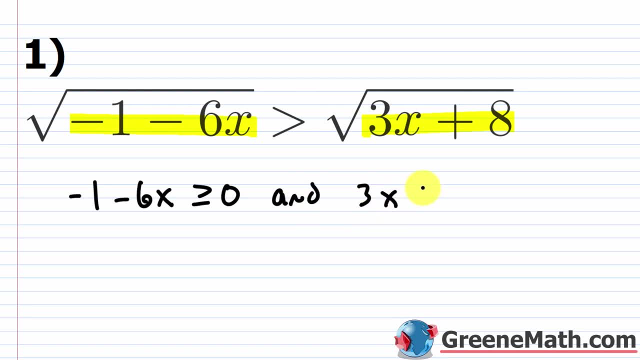 Then you're going to use your keyword and you're going to say: three x plus eight is greater than equal to zero. over here I'm just going to add one to both sides of this inequality. cancel that you'll have negative. six x is greater than or equal to positive one. Let's divided both sides of the. 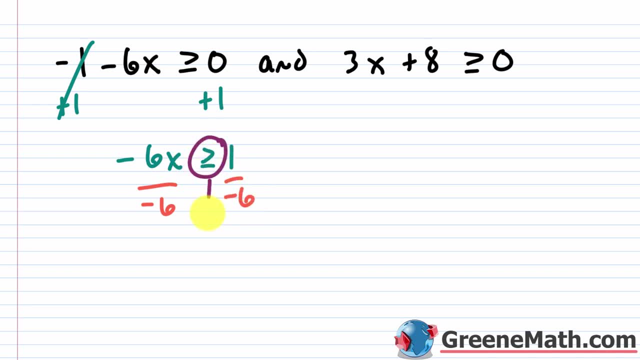 inequality by negative six. And remember, if you divide both sides of inequality by negative, you have to flip the direction of the inequality symbol. this will cancel and give me: X is less than or equal to one. divided by negative six is negative one six. Over here we're going to find the value of. 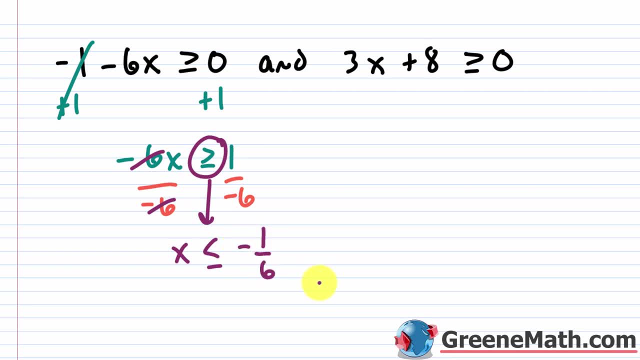 the number one equal to. There is no general way to table anything, whether that is minus one or less than or equal to. So how do you do this? So I'm going to put one over 취 sentir, which is a half of Over. here I'm going to subtract eight away from each side of the inequality. we'll cancel. 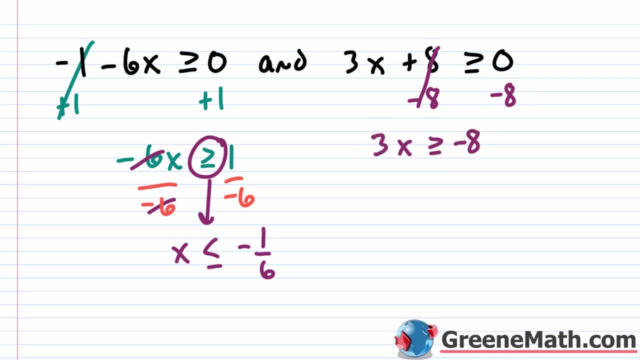 this, we'll say three, x is greater than or equal to negative eight. And then I'll just divide both sides of the inequality by three. cancel this, we'll say the keyword and here, and we'll say x is greater than or equal to negative eight thirds. 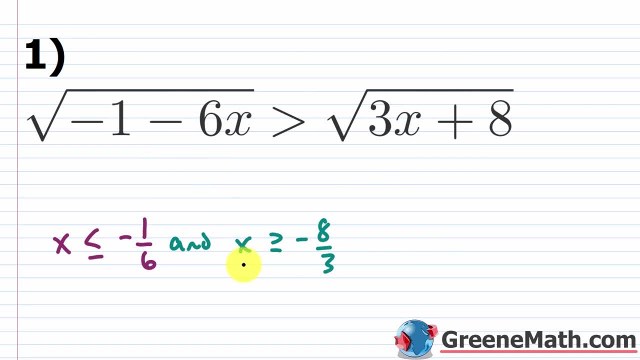 Okay, so coming back up here, if I was showing all the steps to my teacher, I would want to list the domain Again. if you're just doing this on your own, then you could just use this scratch work. you can just keep that. you know that x needs to be greater than or equal to negative eight. 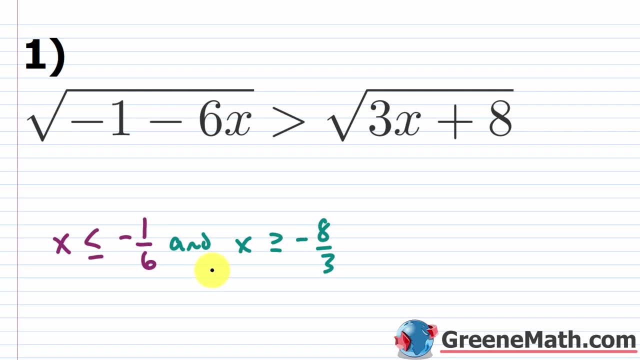 thirds, And it needs to be less than or equal to negative one six. So let's say that the domain, the domain, is the set of all x, such that again we're just going to write this as a three part inequality. So x is greater than or equal to negative eight thirds, and then less than or equal. 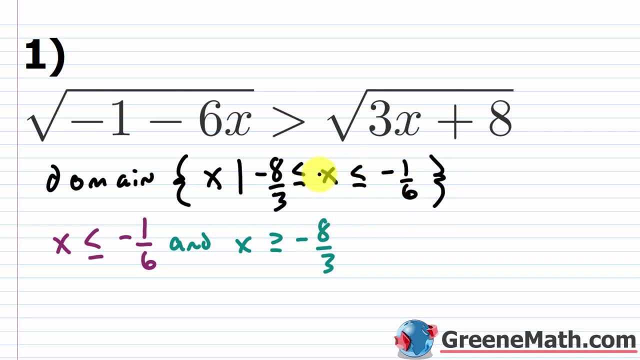 to negative one, six. So if we get a solution and it doesn't fall in this domain, we have to reject it. Okay, so that's very important. And now let's think about solving the related equation. So we have the square root. 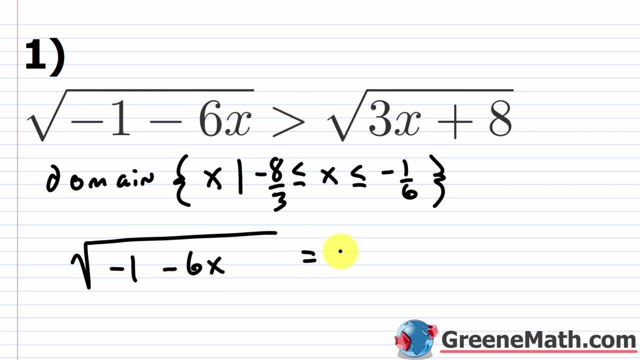 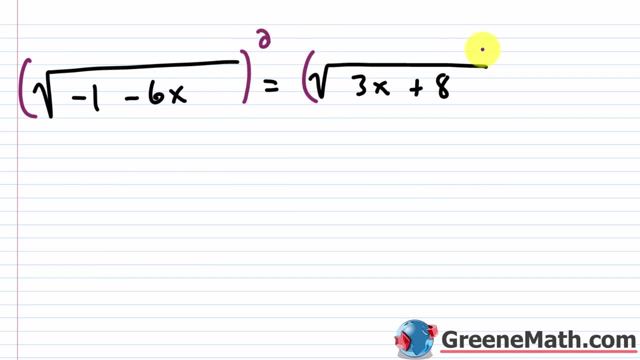 So the square root of negative one minus six x is equal to the square root of three x plus eight. For this one, since each square root is isolated, I can immediately square both sides. it gives me negative one minus six x is equal to: you're going to have three x plus eight. I'm going 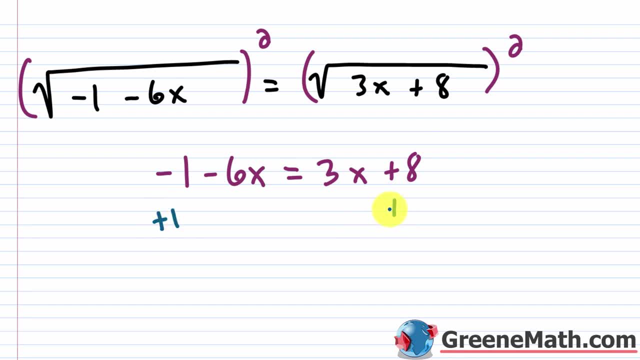 to solve this resulting equation. So let's add one to both sides of the equation here. that would cancel. Let's subtract three x away from each side of the equation. that would cancel. So negative six x minus three x. So negative six x minus three x is negative nine x and this equals eight plus one is. 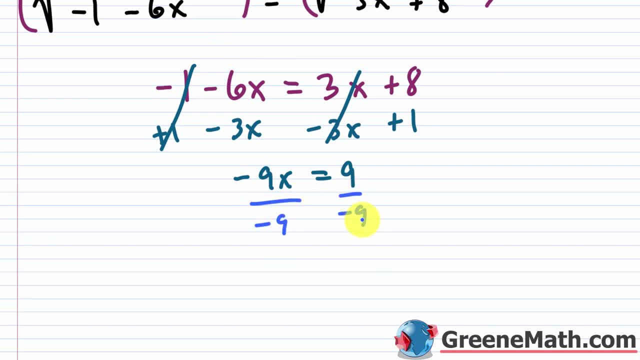 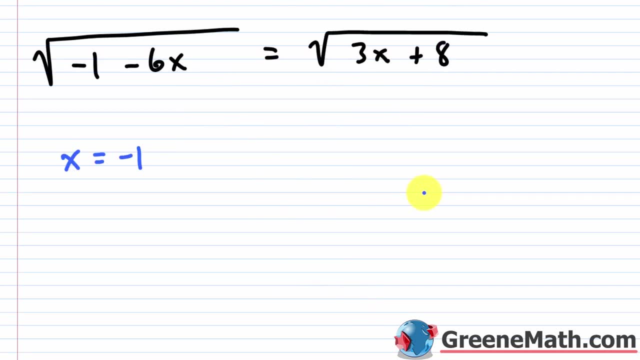 going to be nine. Okay, from here I'm going to divide both sides of the equation by negative nine. Let's cancel this. we'll say x is equal to negative one. we know that if we square both sides of an equation we have to check for extraneous solutions. 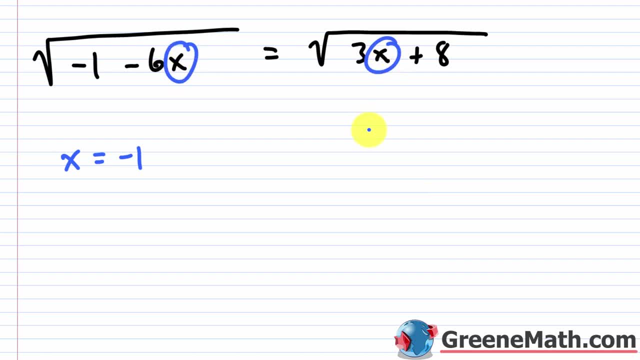 And so you would plug in a negative one here and also here. So basically you would have the square root. So negative six times negative one is six, and then six minus one would be five. So this is the square root of five. 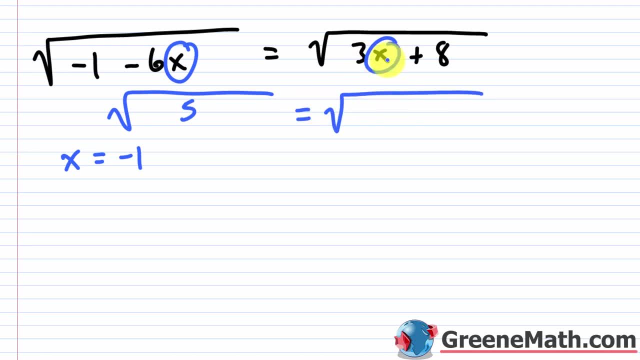 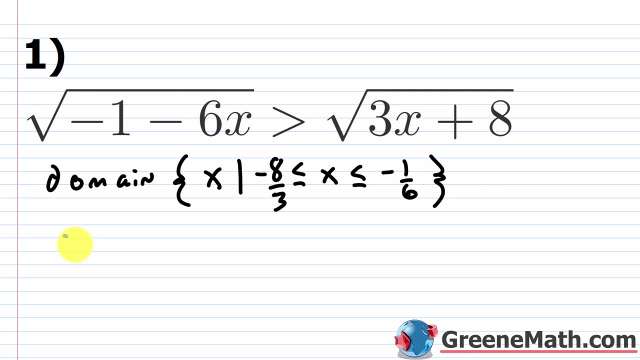 This would be equal to, over here, Three times negative one is negative three. then plus eight would be five. So you get the square root of five equals the square root of five. So this is a valid solution. So, coming back up here, I'm going to write: x is equal to negative one. 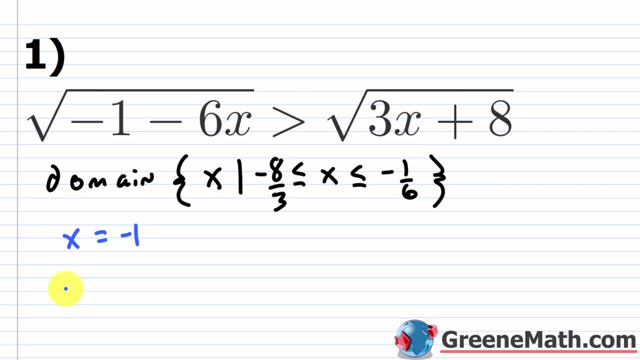 And I'm going to write this in a different way, just so it's more clear what's going on. Let's say we have the square root of negative one minus six x. I'm going to subtract this guy right here, away from each side. 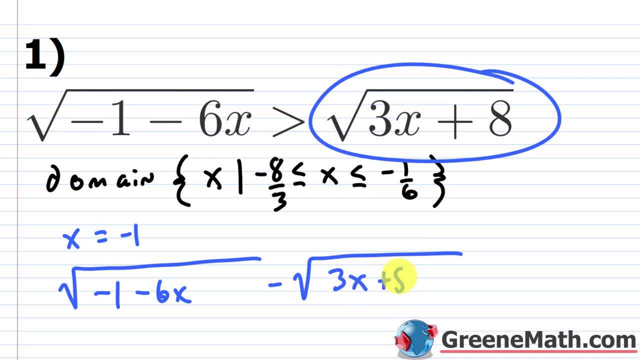 So then, minus the square root of three, x plus eight, And of course this would now be greater than zero in the inequality form. Or you could say it's equal to zero if we're working with the equation, and I'll swap this back in a moment. 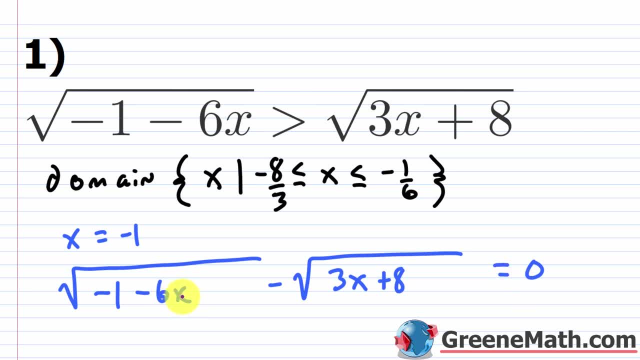 I just want you to think about what happens if you plug in a negative one. right, if we plug in a negative one for x, we know the left side is zero, so you get zero equals zero. But if you change this back to an inequality again, all I need to do is test on each side. 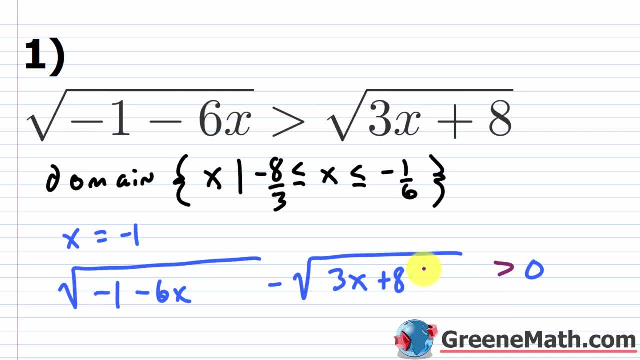 of negative one. I know negative one makes this side zero, So I just need to figure out what I need to plug in values that are greater than negative one or less than negative one. Okay, so you're going to test on each side. the curveball here is it's subject to this. 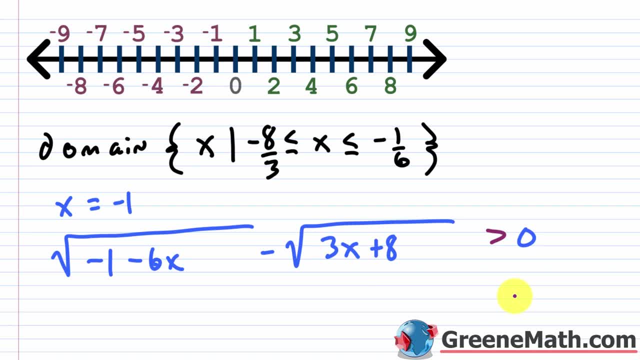 domain. I want to keep that in mind. All right, so you want to come to a number line, or you can make a table, Or again, if you're doing this on your own, you can just make some scratch work, it's. 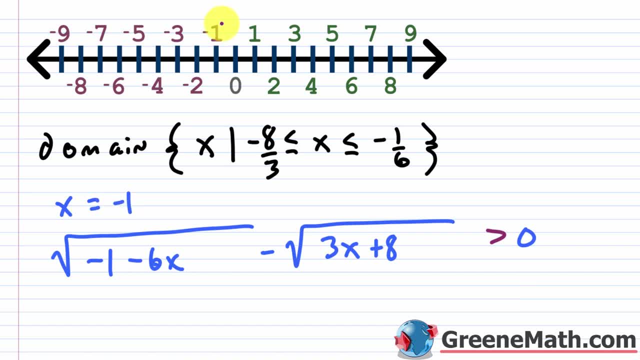 kind of up to you, But you want to think about negative one, that's going to be the boundary. So let's go ahead and put that as a little dashed line here, And then again it's subject to this domain. So if you need this, then you can put it in. 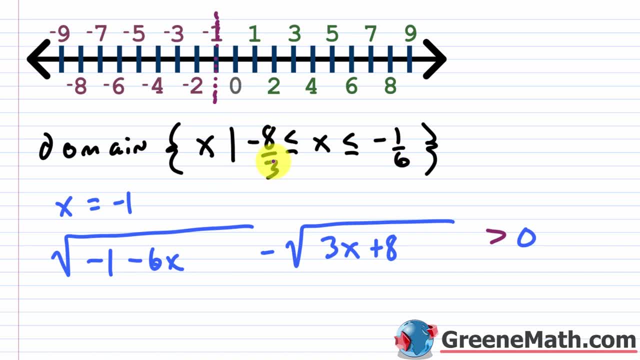 If you don't, then again it's up to you. But negative eight thirds. let's just say that's about, and I'll do some different color. Let's say that's about, right there, And I'm going to label that as negative. let me make that a little bit better. 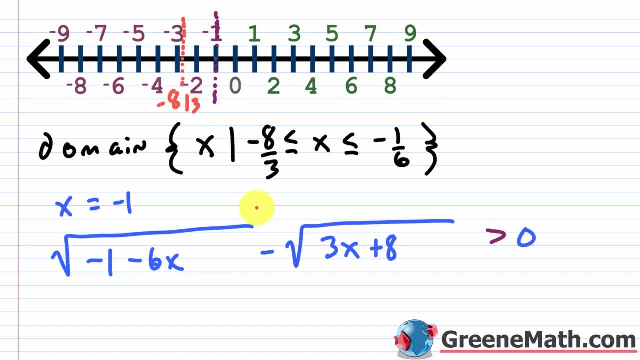 So negative eight thirds. And then the other guy is negative one six. So let's say: this is gonna be really, really tight here. Let's say, that's about right there, Let me do some different color. So I'll just put this like this: 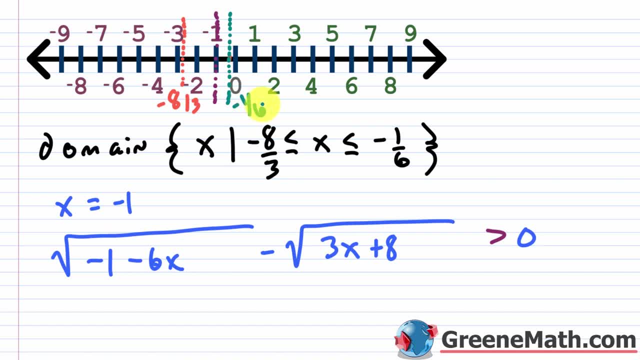 And I'll say that this is negative one, six, like that. Now, what you'd actually want to do is think about this in terms of the four regions. So you have region A and I'm not including any of these values here. So the negative eight thirds, the negative one or the negative one six, I'm gonna think. 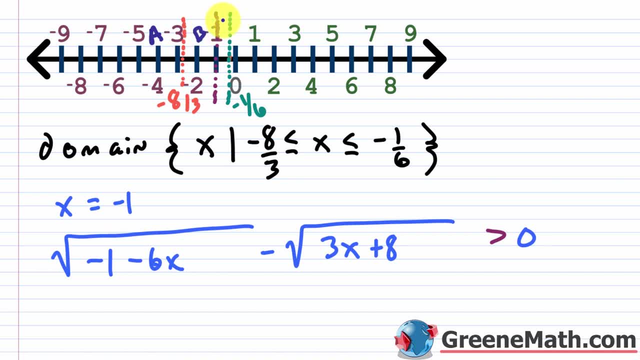 about those separately. So you have region A, you have region B. let's say this is region C, if I can fit that in there, And this is region D. Okay, So region A would be anything that's less than negative eight thirds. 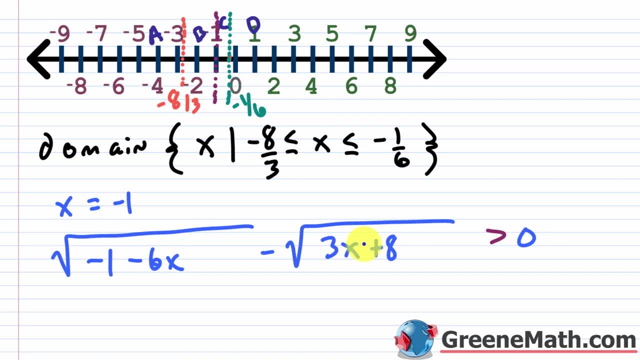 We already know that that violates the domain. So negative eight thirds itself is okay, So we'll talk more about that in a moment. But anything less than negative eight thirds, that will violate the domain. So that's automatic reject. So I'm going to say that region A, region A, or actually let me just put A here: make. 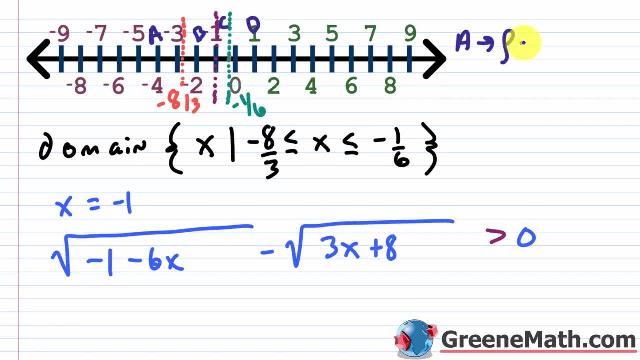 this a little bit shorter. I'll say that: A- this is going to be false, Or you could put that I'm going to reject it Now. region B: that's going to be between negative eight thirds and negative one. Okay. 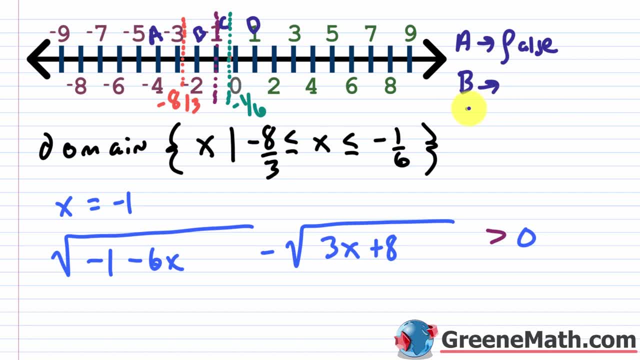 So region B: we have to test that. So that's, we don't know at this point. Region C: that's going to be between negative one and negative one six. So we have to test that, right, We don't know. 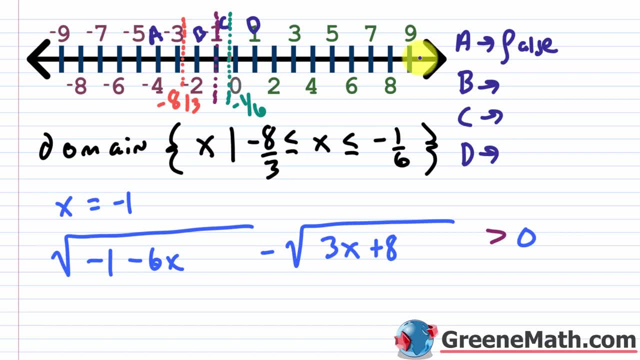 And then for region D, we're going to reject that, because that's anything that's going to be greater than negative one six. Again, negative one six itself is okay- right, X could be that- but it can't be greater than negative one six. 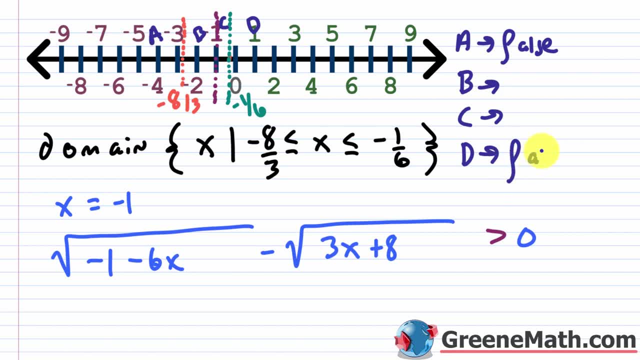 So we have to automatically reject that. That's outside of the domain. So we would say that this is false automatically. So let's test something from region B and then, just for completeness, let's test something from region C as well. So in region B you could use something like, let's say, negative two. 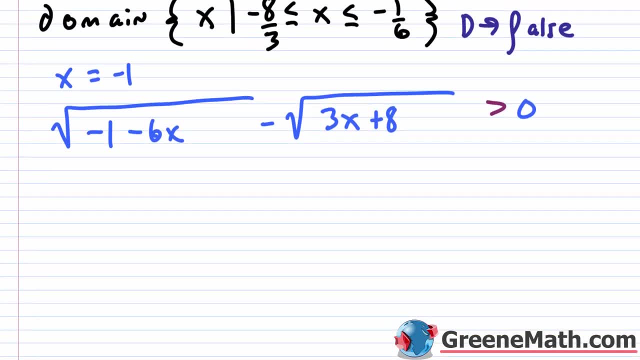 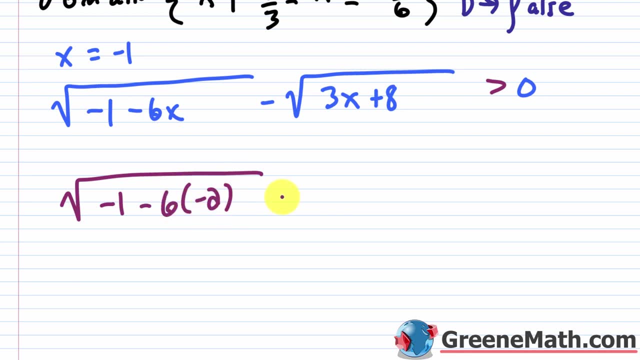 You see that values in there. I think that'd be easy to work with. Let's just come down here. We'll come back up in a moment. So you'd have the square root of negative one minus six times negative two, then minus. 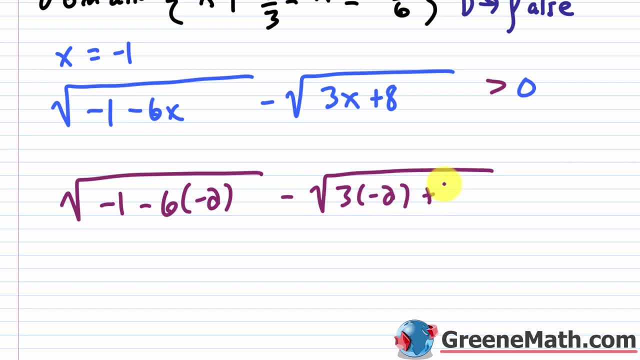 the square root. You have three times negative two and plus eight. Is this greater than zero? So this right here would be positive 12.. And so negative one plus 12 would be 11.. So this is the square root of 11.. 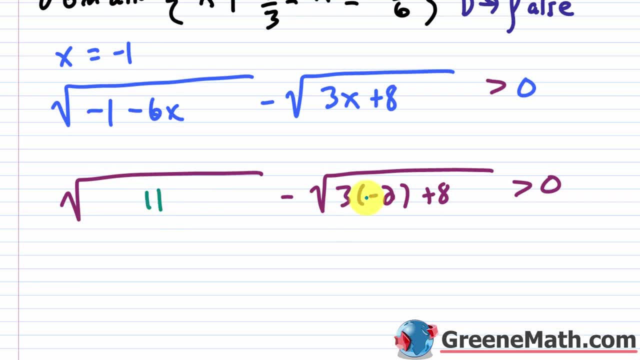 And then over here you have three times negative two. That's negative six, and negative six plus eight is going to be two. So this is the square root of 11 minus the square root of two. Without using a calculator, I think you can see that this is going to be greater than. 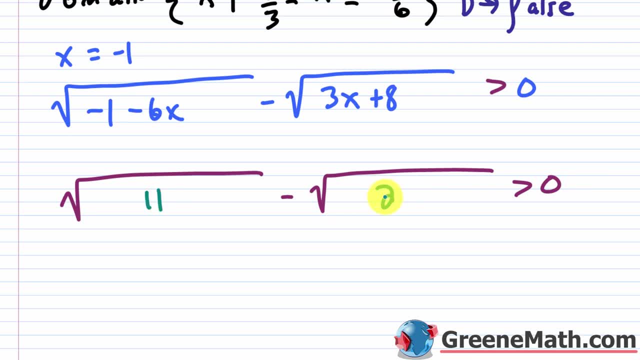 zero, right? The square root of 11 is larger than the square root of two, And so if you subtract the square root of 11 minus the square root of two, you will get a positive value, right? So this is obviously greater than zero. 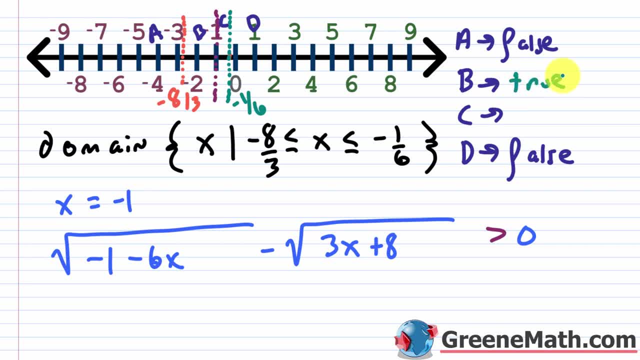 So, coming back up here, I'm just going to mark that this is true, right? So anything in region B is going to work. Now, for completeness, let's check something in region C, and this is a tight window, So I'm just going to pick something like negative 0.5 or negative one half and just show you. 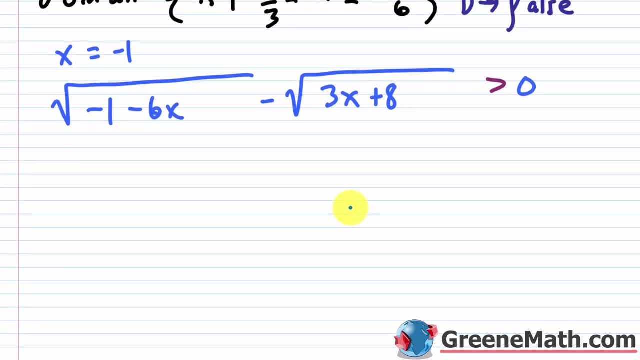 that it doesn't work. I'm just going to write here right now that it's false, but I'll just prove that to you, All right. so let's set this up. I'm going to go the square root of negative one minus six times negative one, half then. 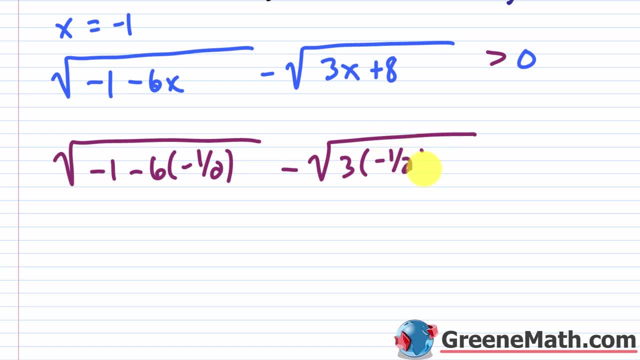 minus the square root. So negative six times negative. one half is three, and then negative one plus three would be positive two Over here. three times negative. a half is negative three halves. So this is negative three halves. Now, without going through and getting a common denominator, you can already see that this. 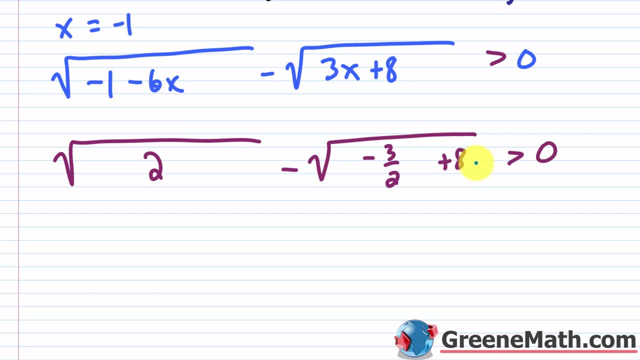 is a false statement. This is negative 1.5.. If I add that to eight I'm going to get 6.5.. So this right here would be larger than this right here. So basically, you're going to have a. 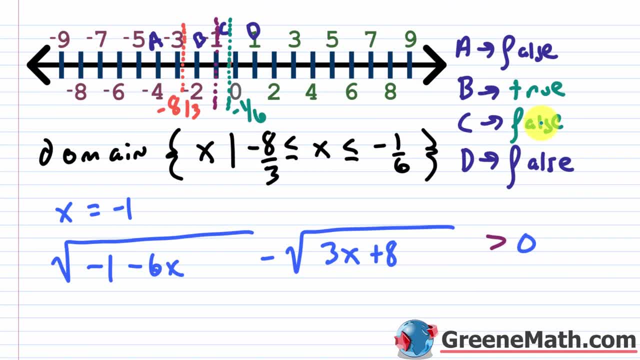 negative, and that's never going to be greater than zero. All right, coming back up here, we verified that things in region C will not work. So now what I want to do is think about region B and think about the endpoints, whether they 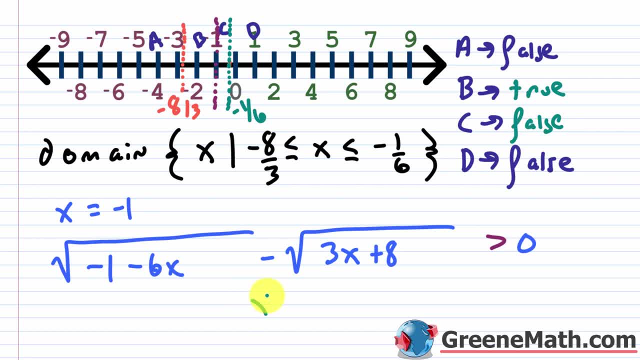 will work or not. Okay, so for region B we have: x is greater than negative eight thirds and it's going to be less than this negative one. So let's think about each of these. Would negative eight thirds work? Yes, negative eight thirds is in the domain and it is less than negative one, right? 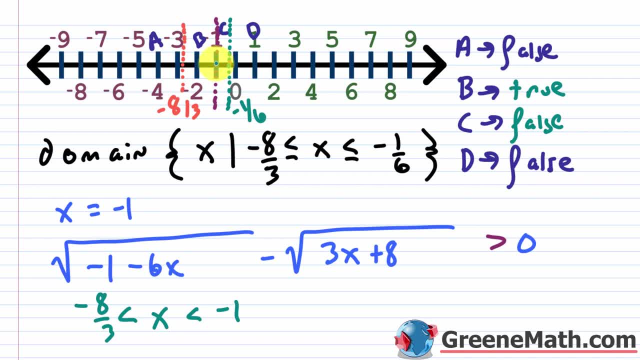 Things that are less than negative one work or satisfy the inequality. So that means that negative eight thirds would work. But again, if you go less than negative eight thirds you're outside of the domain, So you have to exclude those values. But negative eight thirds itself would work. 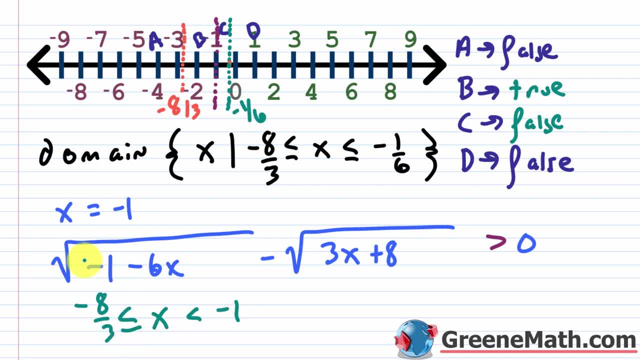 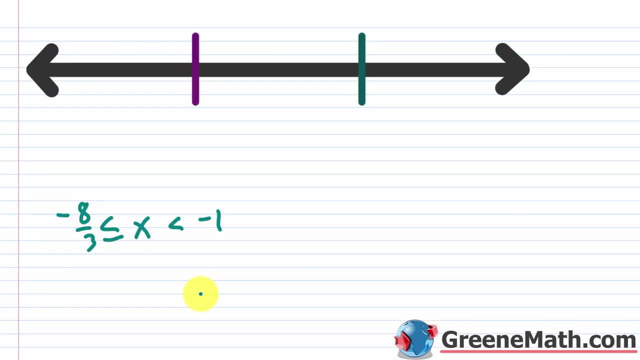 So I'm going to make this less than or equal to here. Then for negative one it's not going to work because this right here we know would be zero, and zero is not greater than zero, So this is going to be excluded. So when we write our solution, we would basically say that x is greater than or equal to negative. 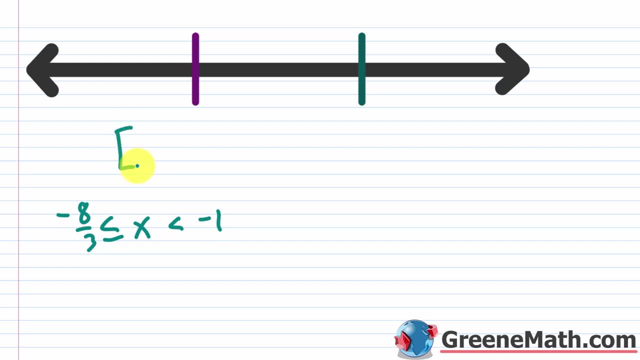 eight thirds and less than negative one. So we would say a bracket Here. So negative eight thirds and then comma. you have your negative one and then use a parenthesis there because it's not included. So that's going to be your interval notation. 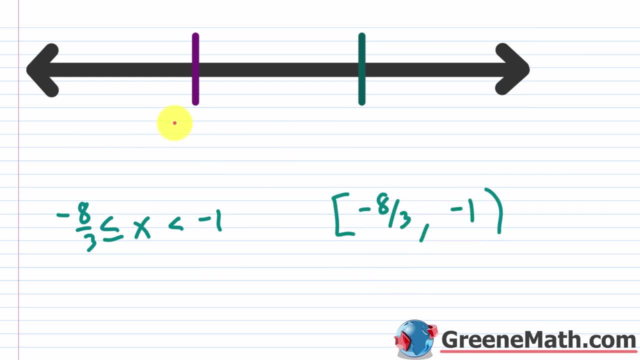 Let's just put that over there And then, graphically, if you want to put that in, you could put this as negative eight thirds, you could put this as negative one, And then essentially, you're going to put a bracket here because it's included, or again. 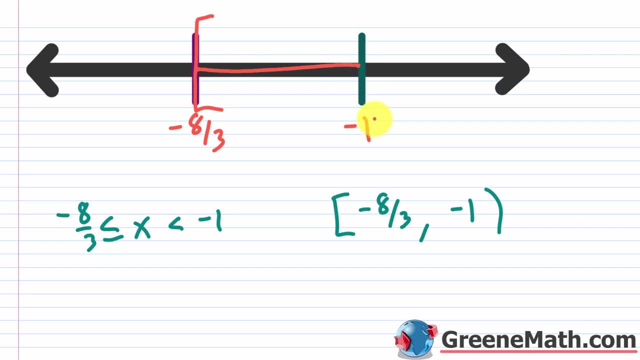 some books will use a filled in circle. then you're going to shade all this up to, but excluding negative one. So we'll use a parenthesis there. Or again, some books would use an open circle. Again, it's really up to you what you do. 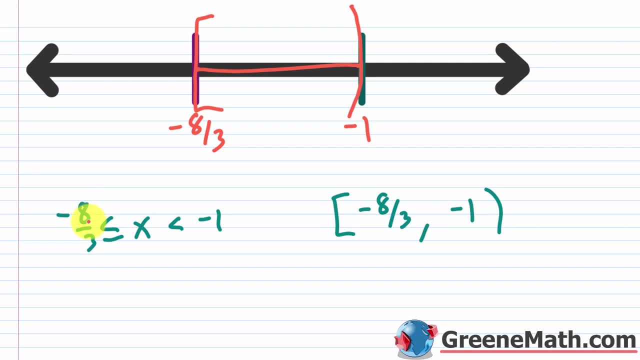 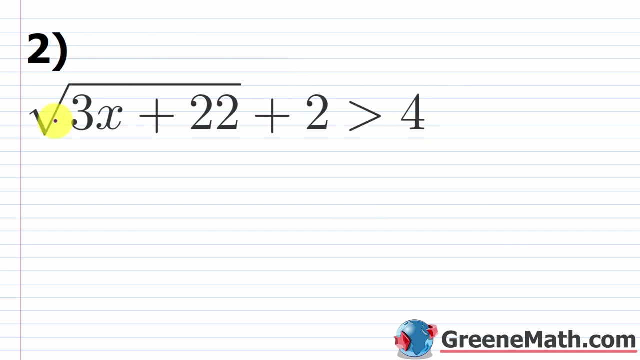 But this would be graphically. this is your x is greater than or equal to negative eight thirds and less than negative one. And then this is your interval notation. All right, let's take a look at problem number two now. So here we have the square root of three x plus 22,. then plus two. this is going to be: 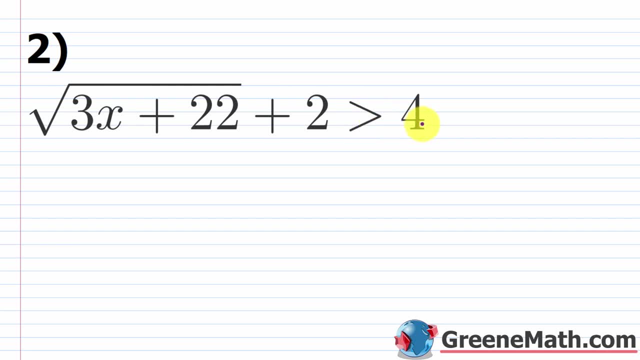 greater than four. So the idea here again is: I'm going to figure out what is the domain. So take your radicand, which is three x plus 22, and set it as greater than or equal to zero. So we're going to say three x plus 22.. 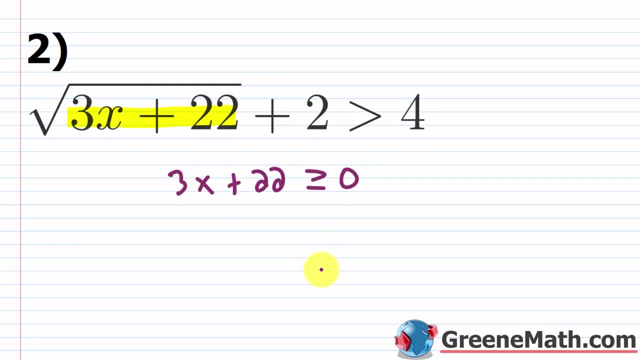 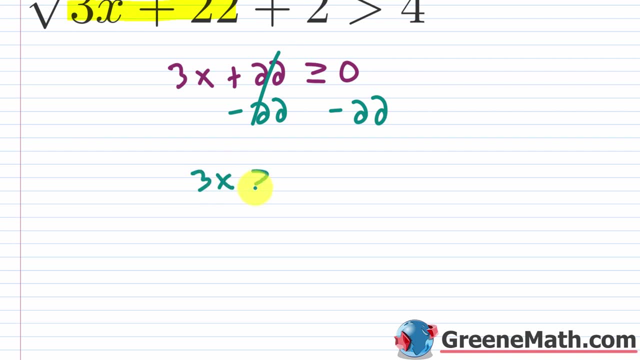 Is greater than or equal to zero. Okay, Is greater than or equal to zero. pretty easy to solve this inequality: what I'll do is subtract 22 away from each side. let's cancel this away. we'll say three x is greater than. 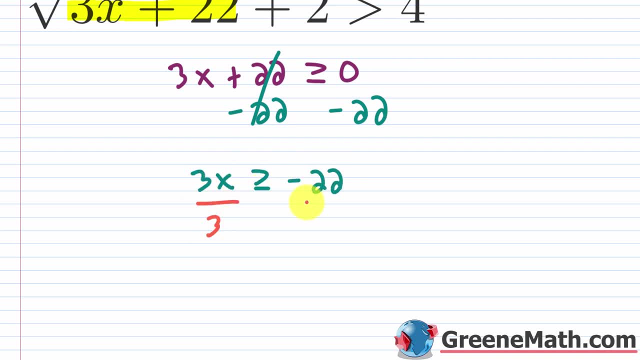 or equal to negative 22.. And then from here I'm going to divide both sides of the inequality by three, And so we'll cancel this three. with this three you have: x is greater than or equal to this negative 22 over three. 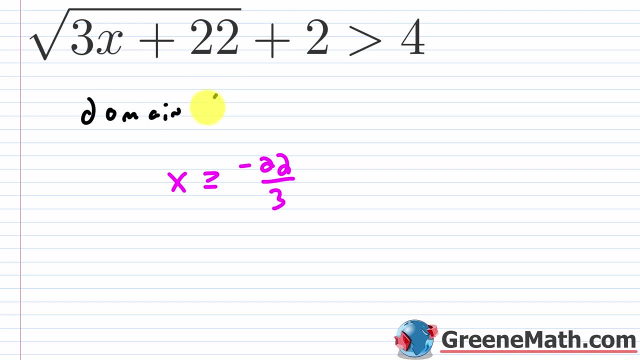 So again, I'm just going to write that my domain is the set of all x, such that x is going to be greater than or equal to this negative 22.. And then, basically, from here, I'm just going to replace this inequality symbol with an. 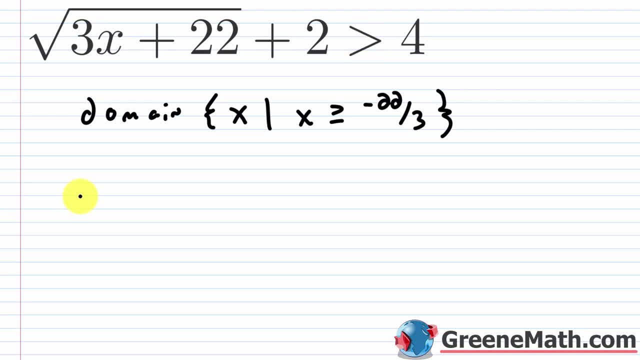 equality symbol. And then I'm going to solve that resulting equation. So I'm going to say the square root of three x plus 22,. and then plus two, we'll say that's equal to four. Okay, so what I want to do in this situation is isolate my radical 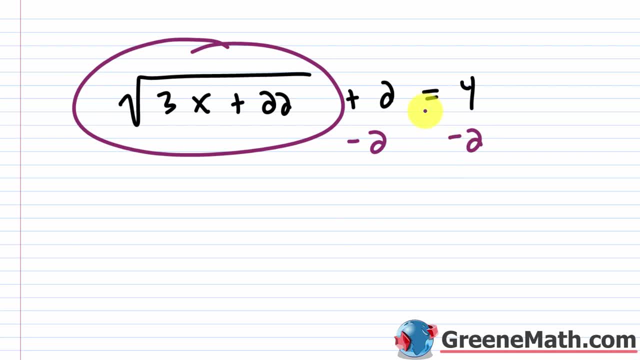 So this guy. and to do that I need to subtract two away from each side. this would cancel. you'd have the square root of three x plus 22.. Okay, so now I'm going to do the same thing over here. 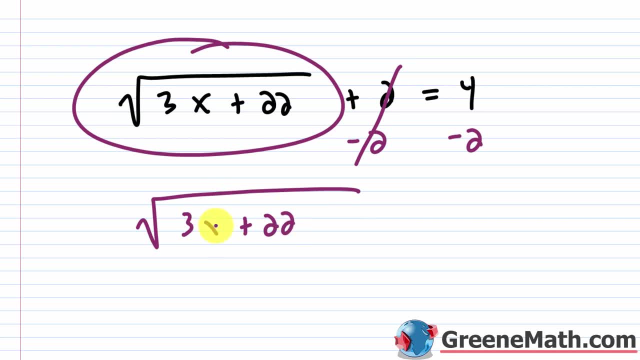 Three x plus 22,. let's make this x a little bit better here. We'll say: this is equal to four minus two is two, And then we'll square both sides of the equation just so we can get rid of this radical here. 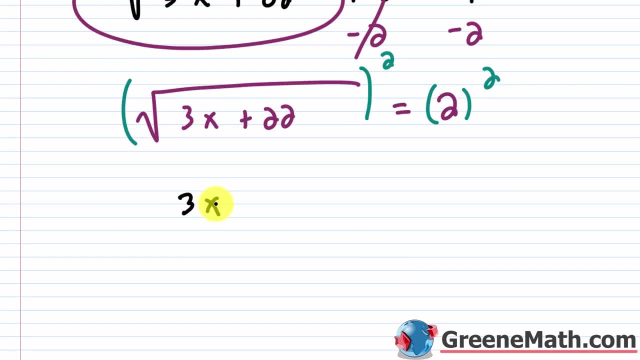 And so on the left side, I'll just have my radicand, which is three x plus 22.. This equals, on the right side, two squared is going to be four, And then what I want to do at this point is subtract 22 away from each side of the equation. 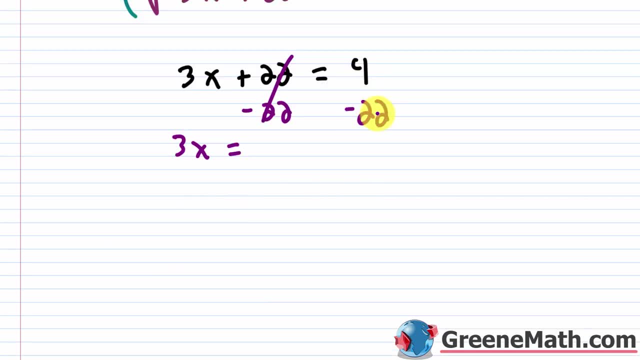 We'll cancel this away. We'll say: three x is equal to four minus 22.. Okay, Three x plus 22 is going to be negative 18.. And then, as a final step, I'll divide both sides of the equation by three. 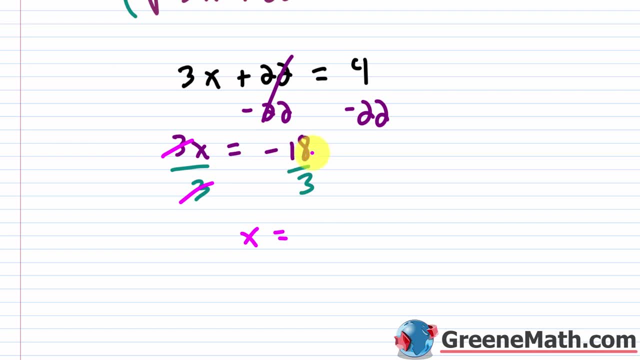 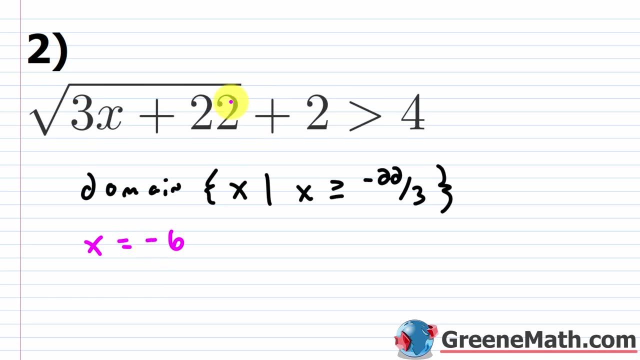 So now let's cancel this with this and say: x is equal to negative 18 divided by three is going to be negative six. So now we have our domain and we have our boundary. So what we'll do? I'm just going to rewrite this as the square root of three x plus 22.. 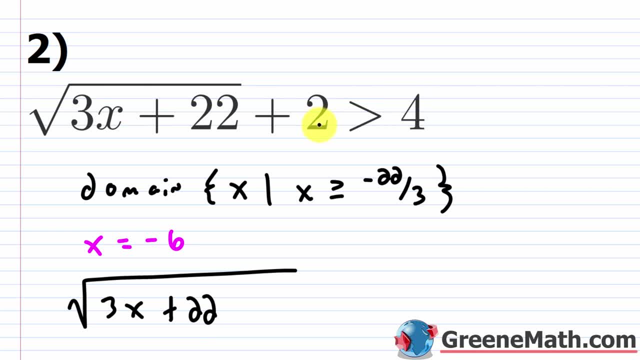 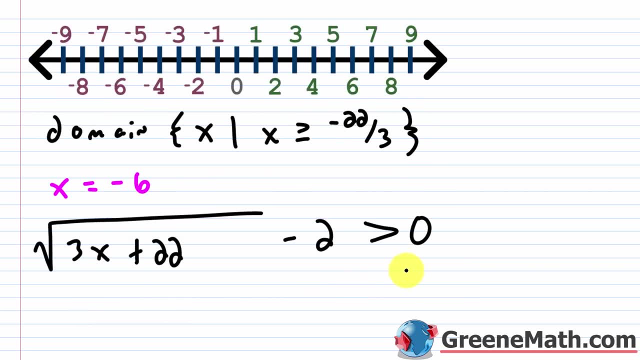 What I'm going to do is subtract four away from each side of the inequality. So two minus four would be negative two. So then minus two, And this is greater than zero. For me this is a little bit easier to work with. 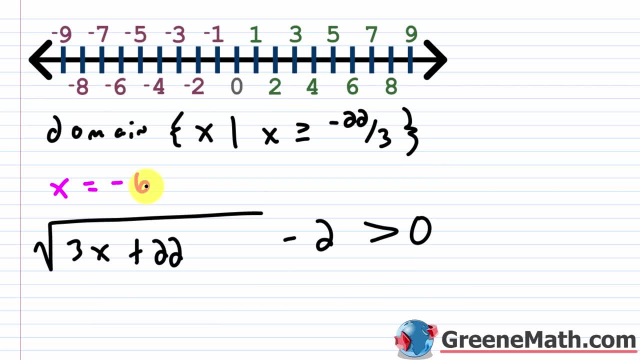 And let's come back over here and set up our intervals. So again, x equals negative six. That was the boundary that we found. Let's find that. So that's going to be negative six. Put a little dashed line there. Then the other critical value is negative 22 over three. 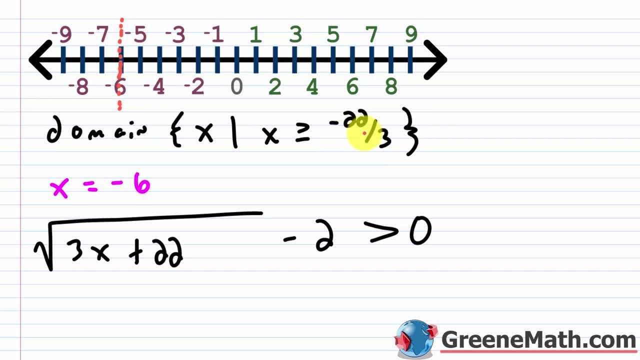 Now negative 21 over three is negative seven. So this is a little bit to the left of negative seven. So let's just say that it's going to be about right here. I know that's not exact, but let's just say that's where it is. 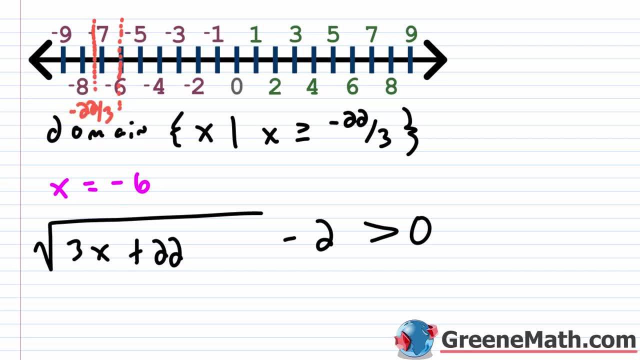 So this is negative 22 over three. let's say: Okay, So now you have these regions, So let's call this one A, let's call this one B and let's call this one C. So A would be anything that's less than negative 22 over three. 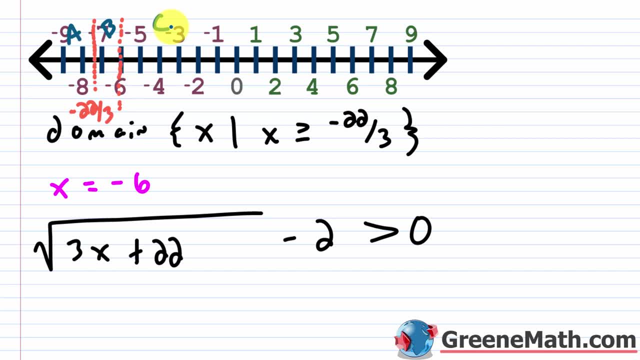 B would be between negative 22 over three and negative six, And then C would be anything greater than negative six And again those critical values, the negative 22 over three and the negative six. I will consider those separately In region A. since this violates the domain, it's automatic reject. 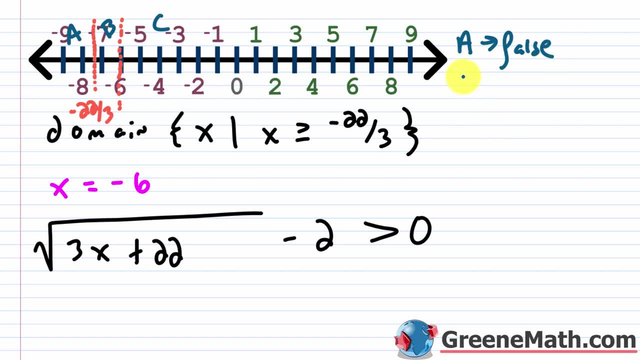 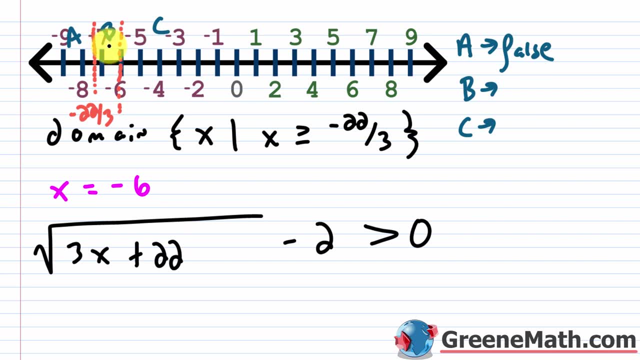 We'll just say this is false. Nothing in there is going to work For region B and for region C. we need to test Now to test something in B. it looks like negative seven is available, So let's work with that. 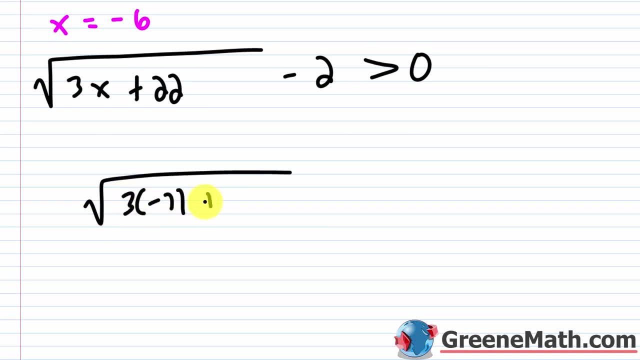 So we'll say the square root of three times negative seven plus 22.. Let's make this a little bit better here. Then minus two is greater than zero. So three times negative seven is negative 21.. So this right here is negative 21,. then plus 22,, which is positive one. 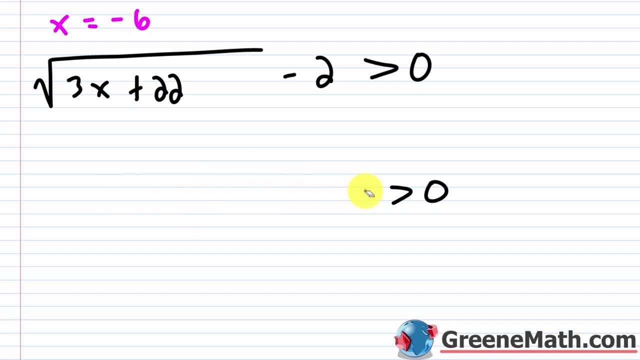 And if we take the square root of one, we get one, And one minus two is negative one. So this right here is a false statement. So we know that region B that's not going to work. So we have to reject those values. 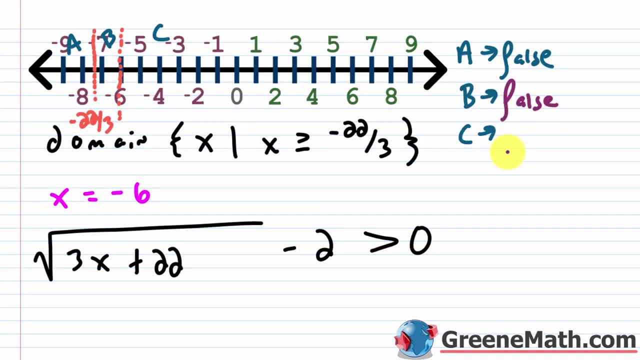 So, coming up here, I'm just going to put false here. Now C is going to work. So I'm just going to put a true for right now and then I'll prove that to you. So for C, I would just pick zero. 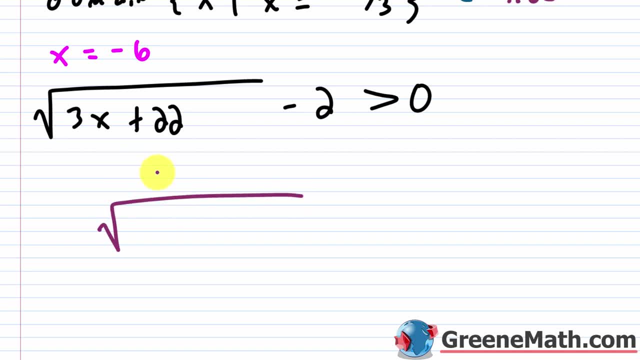 It's nice and easy to work with. So let's say we'd have the square root of three times zero, which is zero, So the square root of basically 22,. then minus two is greater than zero. Now for the square root of 22,. it's about 4.7.. 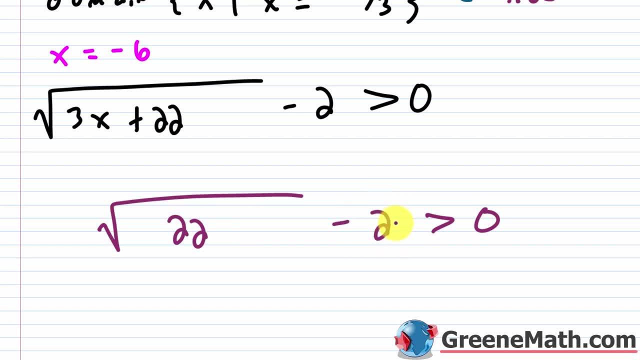 So you can see that this is larger than this two. That's being subtracted away, So this is going to be a positive value. So it will be greater than zero. So anything in region C will work right, So that will be true. 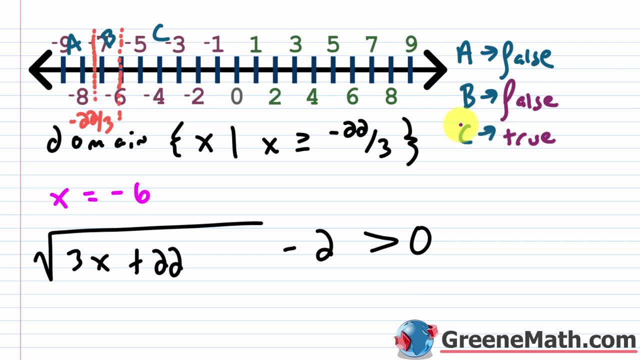 Now coming back up here, since we know that things in region C would work, we would start with our solution by saying that X is greater than negative six. Now, would negative six itself work? Well, think about it: Negative six, if I plug that in here, is going to give me zero on the left-hand side, right. 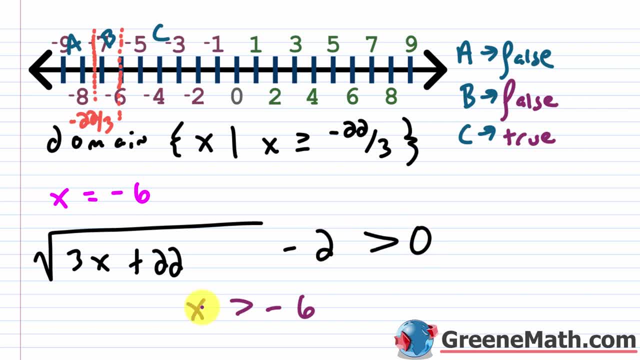 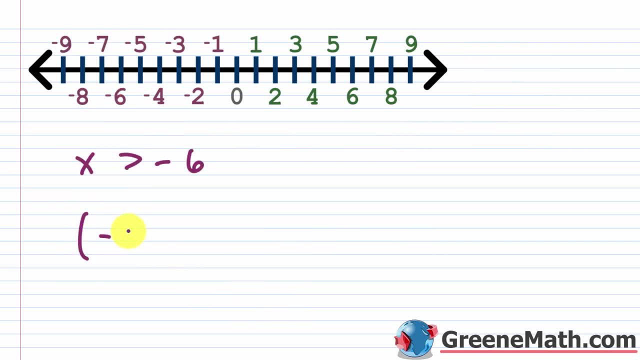 So you'd have: zero is greater than zero, which is a false statement. So negative six would work. It would not work. So this would be your solution And if you wanted to do interval notation, you could just say: you put a parenthesis. 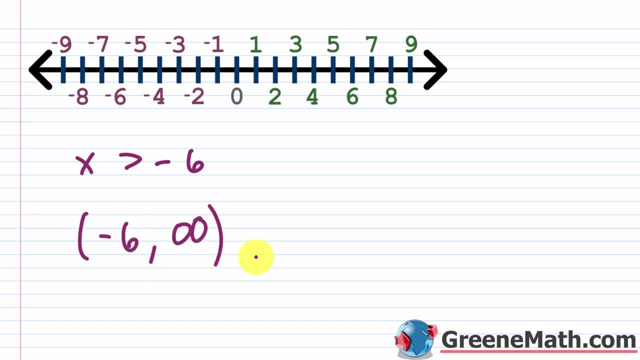 next to negative six, and this is going to go out to positive infinity. And then graphically we would find negative six- And again you could put a parenthesis there or you can do the open circle if you like that- And then we're going to go and shade everything out to positive infinity. 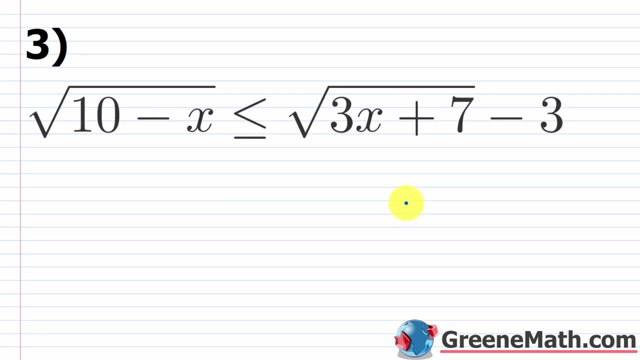 So let's make sure we shade in this arrow. All right, let's take a look at problem number three now. So we have the square root of 10 minus X, And this is less than or equal to. we have the square root of 3X plus seven, and then 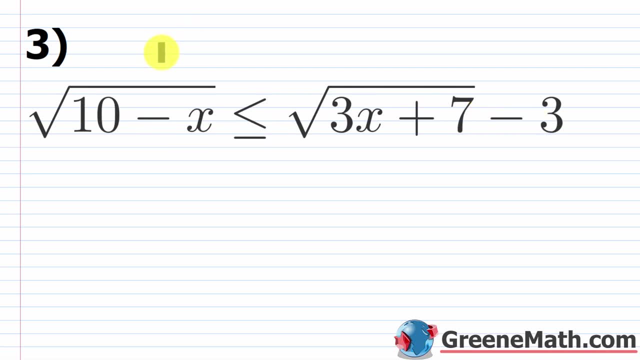 minus three. So the first thing I'm going to do is find my domain. So I'm just going to take this radicand here, which is 10 minus X, and I'll say that that is greater than or equal to zero. 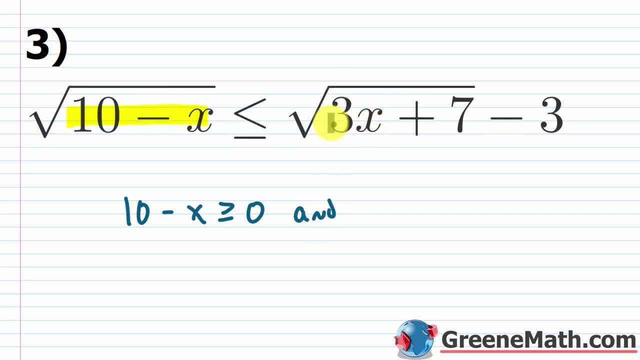 Then I'm going to use my keyword and I'm going to take this radicand here, which is 3X plus seven, So 3X plus seven, And again it has to be greater than or equal to zero. So let's solve this compound inequality real quick. 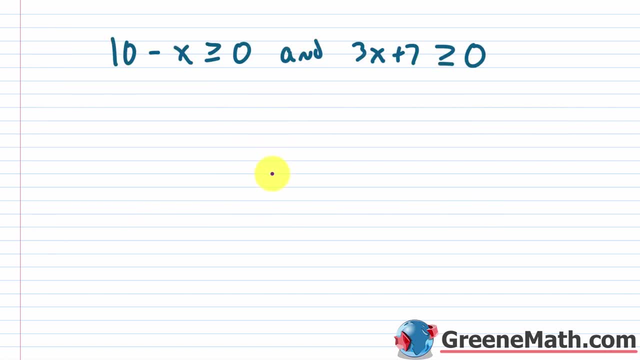 So on the left what we can do is actually just add X, So both sides of the inequality. I think that's the fastest way. So we'll say 10 is greater than or equal to X, or you could flip that around and say that: 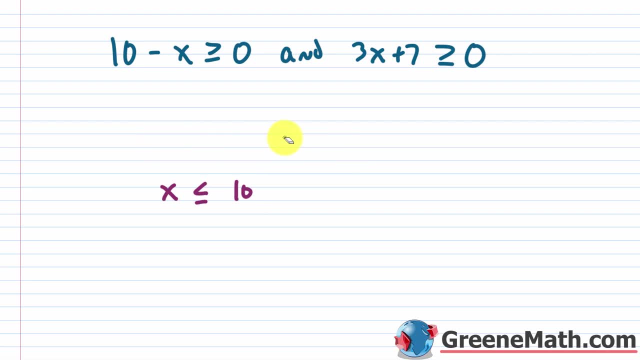 X is less than or equal to 10.. And then for the other guy, let me just write: AND in here We will subtract seven away from each side. cancel this, You'll have that 3X is greater than or equal to negative seven. 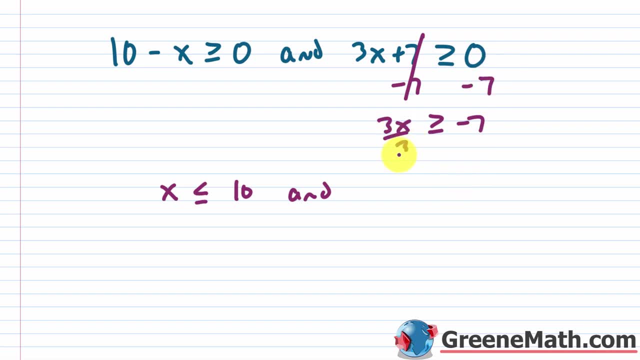 Let me make this a little bit more clean. And then we will divide both sides of the inequality by three. cancel this, So we'll say X is greater than or equal to negative seven. Okay, let's consider this real quick. And so, for the domain, let me write this out. 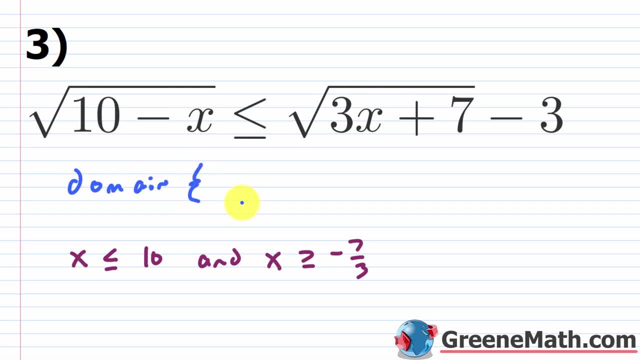 So for our domain we will say that it's the set of all X, such that X has to be greater than or equal to this negative seven thirds, and it has to be less than or equal to positive 10.. Okay, so now let's solve this related equation. 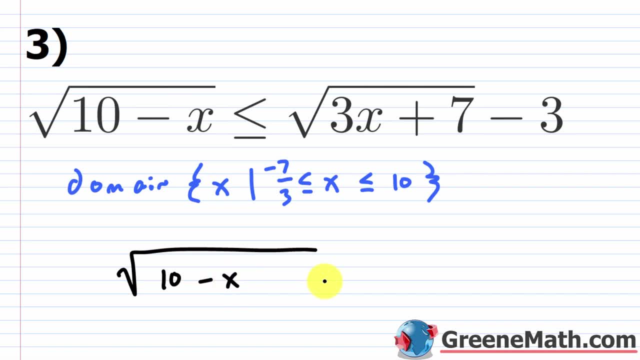 So we'll say that we have the square root of 10 minus X. We'll say this is equal to the square root of 3X plus seven, and then we have minus three. Okay, so I have this radical on the left isolated. 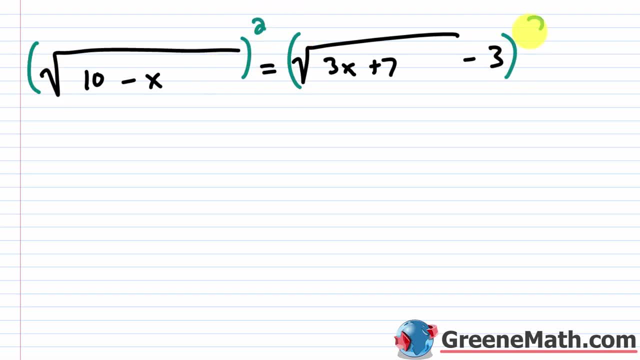 So you can immediately square both sides. But unfortunately that's not going to clear all the square roots involved. So this one squared. we know we just get the radicand. So this is 10 minus X on the left side. Then this equals on the right side again. you have to use your formula. 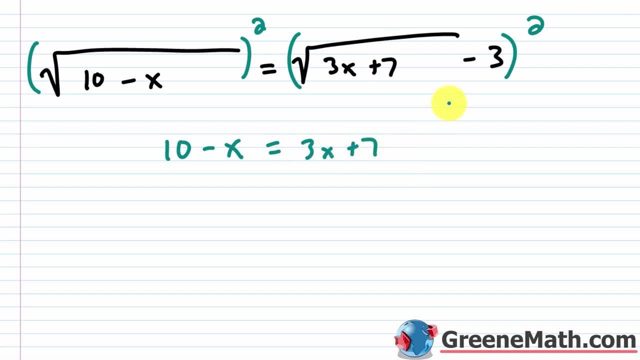 So square this guy, you get 3X plus seven. Then you have a minus, So you bring that and then it's two times this guy times this guy. So two times three is six. then times your square root of 3X plus seven. 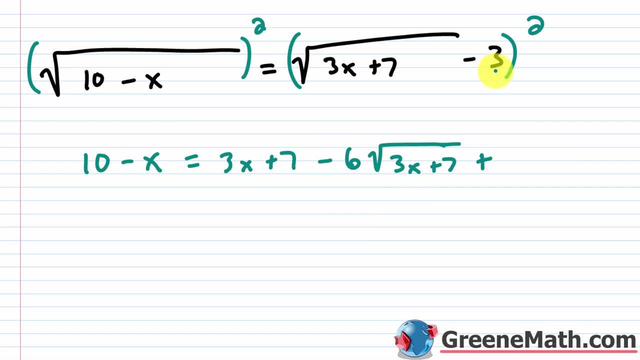 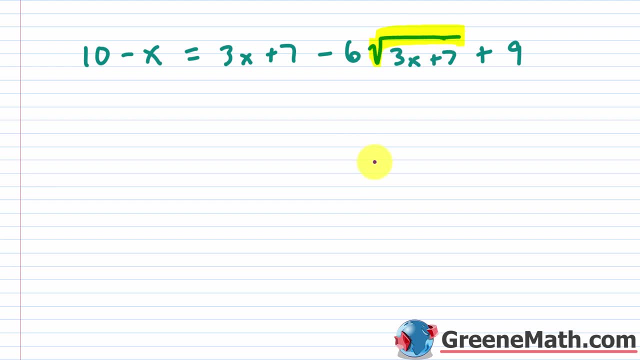 Let me actually slide this down here. Then plus your three, being squared, would be nine. Okay, we need to isolate this radical, So this guy right here, And so to do that, I'm first going to consider that seven plus nine is 16.. 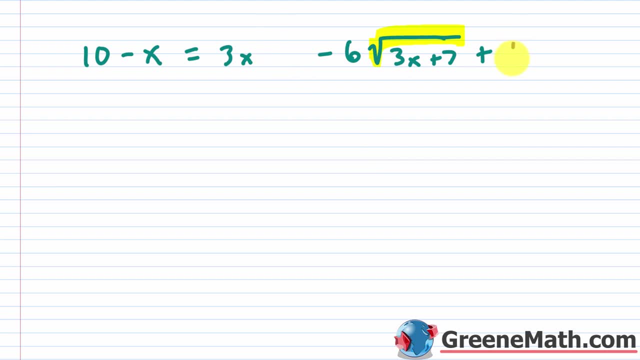 So let's just erase this from here and here, And actually I'll just put it at the end. I'll subtract it away from each side of the equation like this: And so this is going to cancel, And then, additionally, I can also subtract 3X away from each side of the equation. 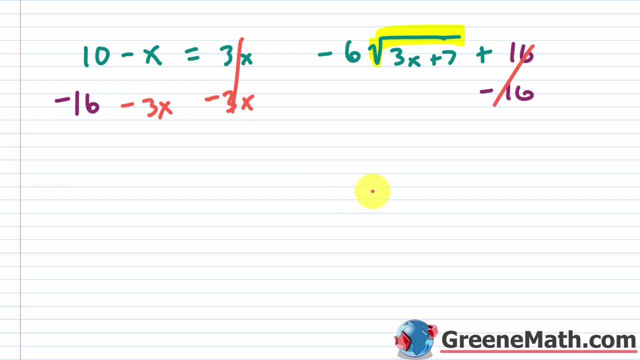 Let's make this a little bit cleaner here. We'll cancel this, And so my left hand side now will be 10 minus 16, which is negative six. So we have negative six, And then negative X minus 3X is negative four, X. 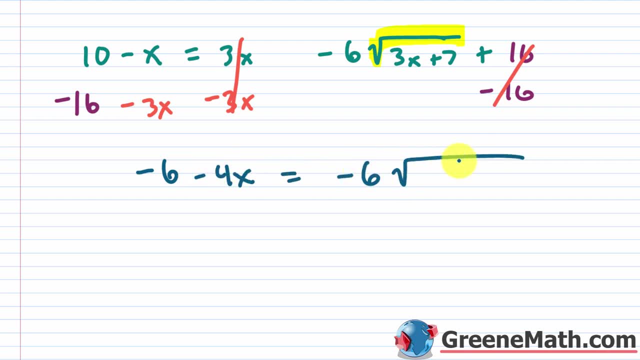 And this equals you have negative six times the square root of 3X plus seven. So, just like I talked about when we were discussing how to solve Radical equations, you could divide everything here by negative six, but then you'd have fractions over here. 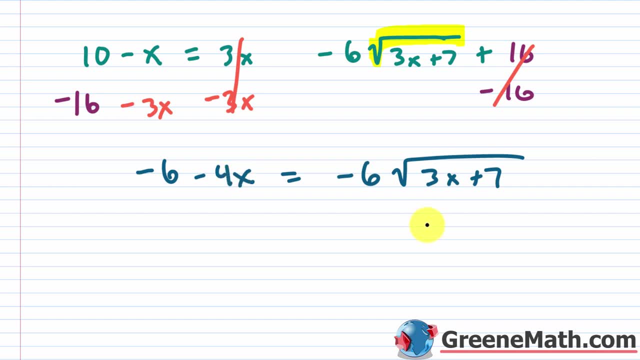 So it's really personal preference What I would do to make things easier. I would first reorder this and say: this is negative four X minus six. I move this out of here and basically drag this up. So what I would do is actually just divide everything by negative two and see where. 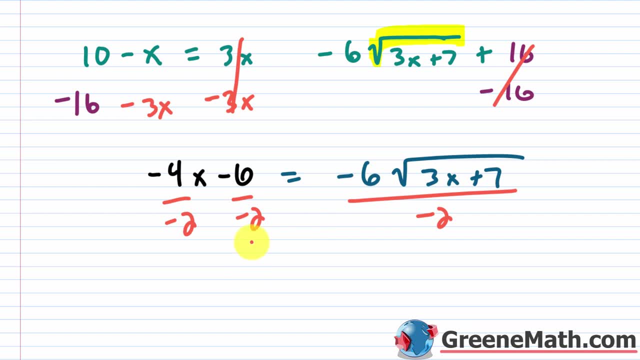 that gets me So basically negative. four divided by negative two is going to be two. So this would be two X. negative over negative is positive. Six divided by two is three. This equals negative over negative is positive. Six divided by two is three. 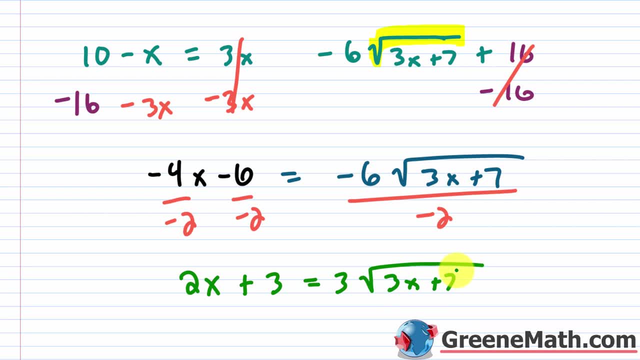 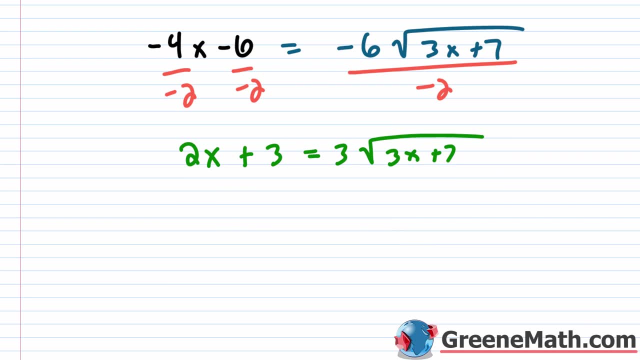 So this is three times the square root of 3X plus seven. Now you still have a number here, but at least you don't have to work with some nasty fractions, So I think this is preferable, at least for me. So what I'm going to do now is just square both sides and let's see where that gets us. 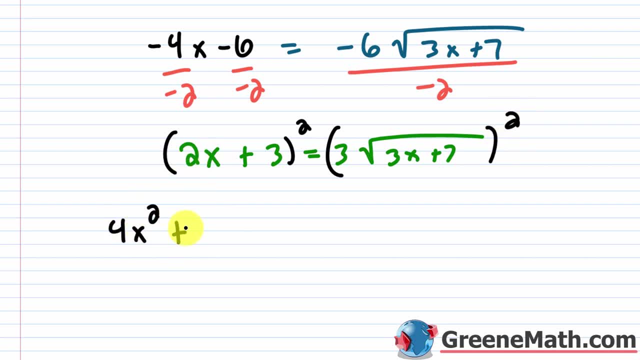 So for this guy, the first guy squared is four X squared. then plus two times this guy times this guy. So two times two is four, times three is 12.. Then times X Plus three squared is nine. This equals. when you square this guy, you have to be really careful. 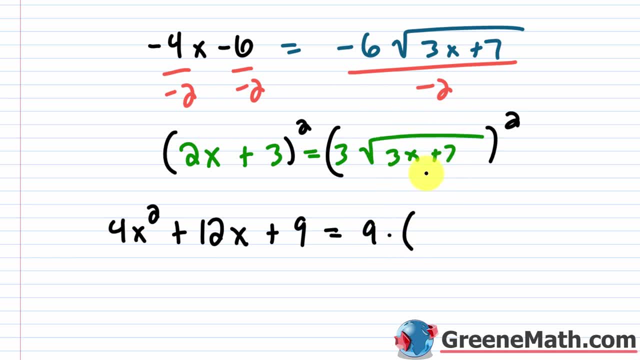 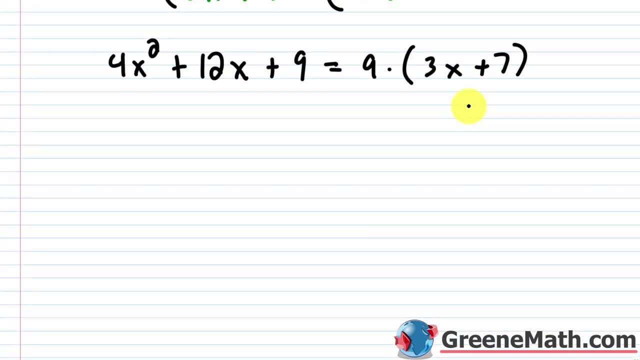 It's three squared, which is nine multiplied by this guy being squared. So you have to wrap this in parentheses. you would get three X plus seven inside, And then you just need to use your distributive property here. So let's write: four X squared plus 12, X plus nine is equal to 27 X plus 63.. 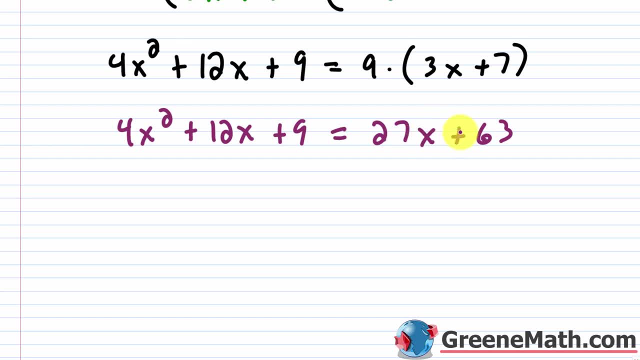 And all I did here was multiply nine times three X to get 27 X. then, plus you have nine times seven, that's 63. So that's all I did. So now we have a quadratic that we need to solve, And for this I would put it in standard form. 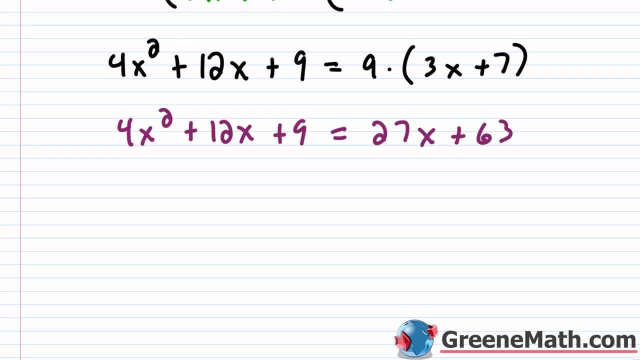 See if it's something you can factor. If you can't, then just use the quadratic formula. So I would subtract 27 X away from each side. Let's cancel that. Let's subtract 63 away from each side. Let's cancel that and put this as zero. 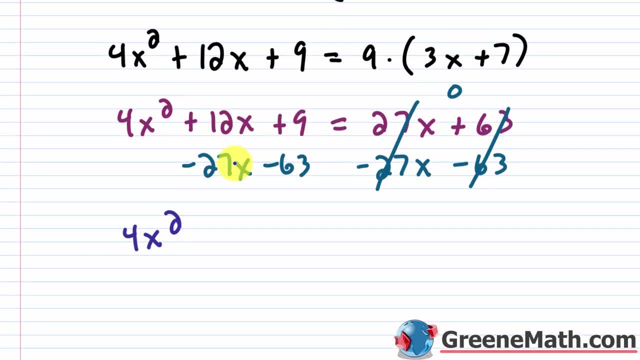 So on the left you'll have four X squared and then 12 X minus 27 X. That's going to be negative 15 X, and then nine minus 63.. That's going to be negative 54.. So minus 54.. 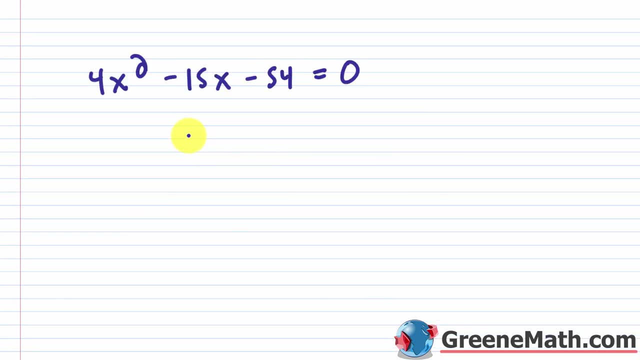 So this is something you can factor, but it's actually not that easy to factor, So you could use a quadratic formula if you have to. again, it's really up to you. I'm just going to factor it real quick because I already know how it works out. 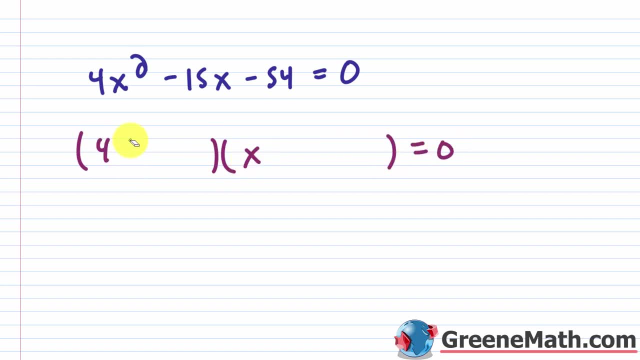 So I'm going to put a four X here and an X here. Now, remember, with four it's either four times one or two times two. So if this didn't work, you'd have to check two times two. Okay, Now with 54, you've got one in 54,, which that's probably not going to work. 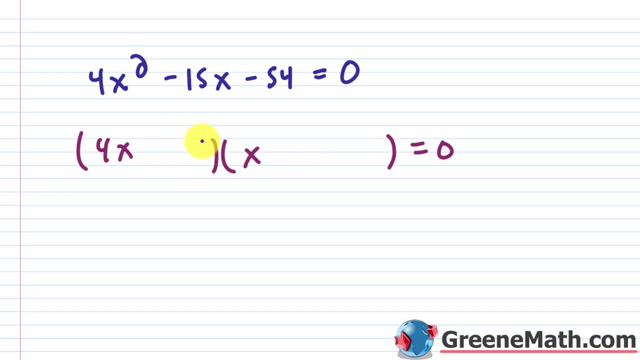 You couldn't put the 54 here because you'd have a common factor of two which you could put the 54 here and the one here. But four times 54, that's 216 and you're subtracting away one because this is a minus here. 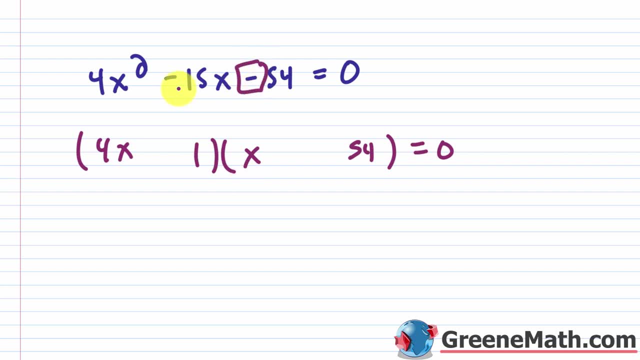 Again, everything is in terms of absolute value, So that's not going to get you to negative 15 or positive 15, again in terms of absolute value. Think about the next one. It's two and 27.. You can't put the two here, but you could put it here and you can put the 27 here. 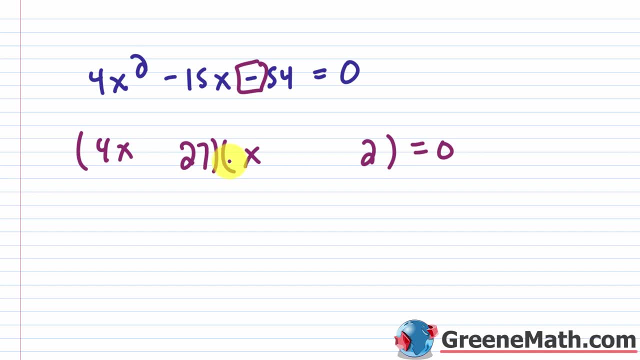 Now, four times two is eight, and then you've got 27,. 27 minus eight, That's 19, and you're trying to get to 15.. So that's out Now. 54 is also divisible by three, So you've got three and 18.. 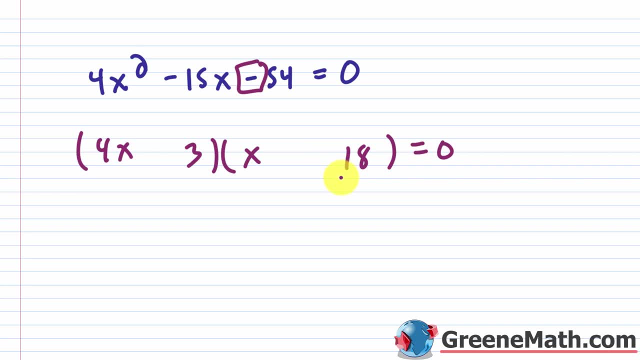 So you can't put the 18 here, but you could put the three here and the 18 here. Four times 18 is 72, and then 72 minus three would be 69. So that's not what we need. And then what else can we do? 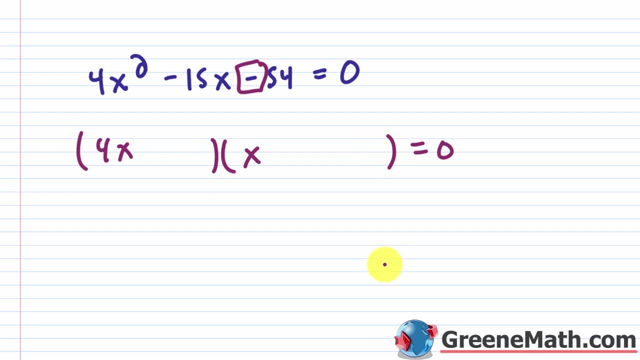 So it's not divisible by four or five, but you could do six times nine. Now you cannot put the six here because you'd have a common factor of two, but you could put the nine here and the six here. Now it turns out this is what you're going to need. 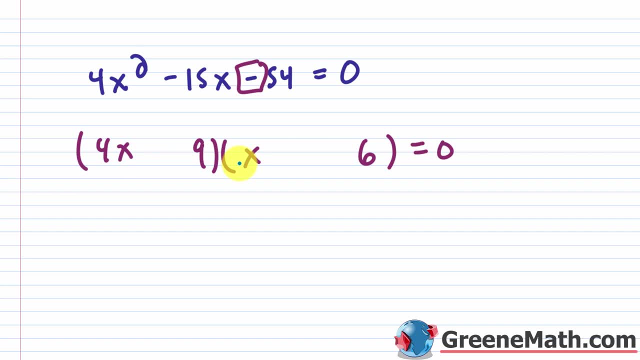 Four times six is 24 and nine times one is nine. 24 minus nine is 15, but you have to make the signs work. So this needs to be negative and this needs to be positive. So that will give me a negative 24 X and this would give me a plus nine X. 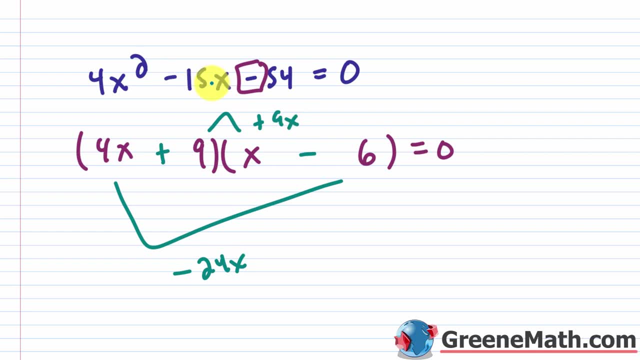 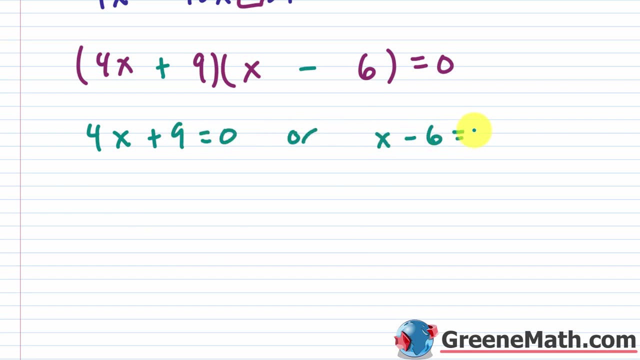 So negative 24 X plus nine X is negative 15 X. So this is what we want. Okay, So let's say that four X plus nine is equal to zero, or let's say that X minus six is equal to zero, And what I'll do here is subtract nine away from each side. 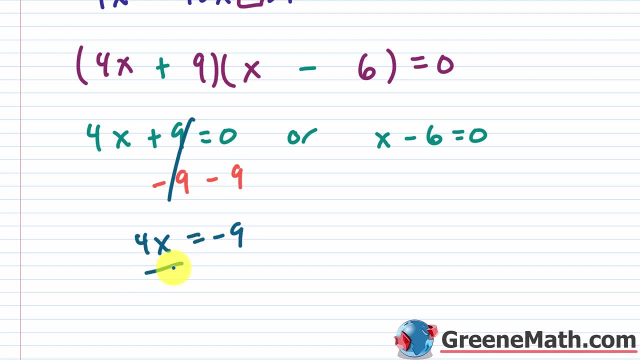 We'll cancel this away and say four, X is equal to negative nine. Let's divide both sides of the equation by four and let's cancel this and say that X is equal to negative nine fourths. Then, over here, let's add six to both sides of the equation. 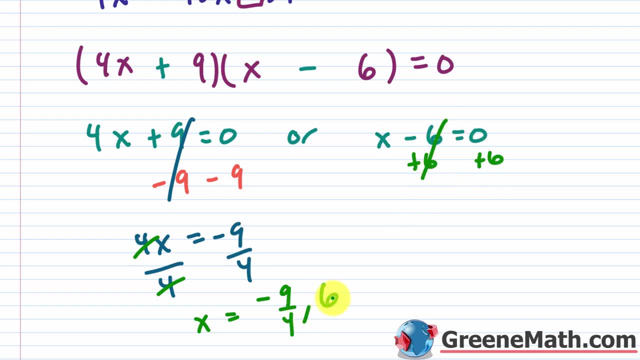 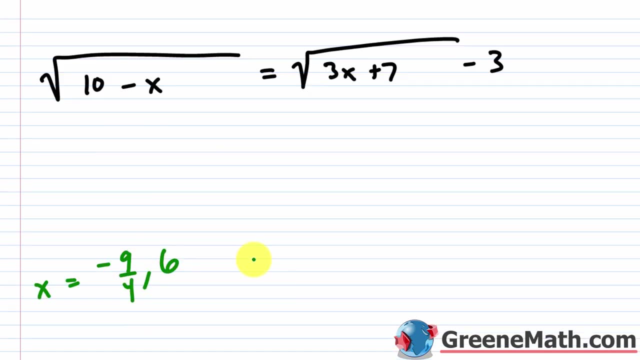 We'll cancel this. So also, we get X equaling six. Now again, these are proposed solutions. We did square both sides of an equation, so we need to check for extraneous solutions. All right, So let's check each one of these. 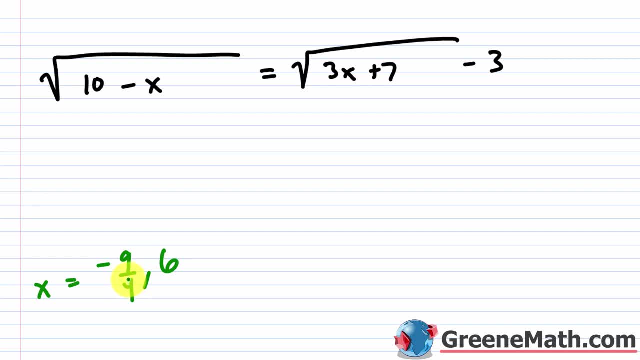 So I'm going to tell you in advance: negative nine fourths is not going to work. Instead of going through and trying to get common denominators, you can just use this as a decimal. So negative nine divided by four, that's going to be negative 2.25.. 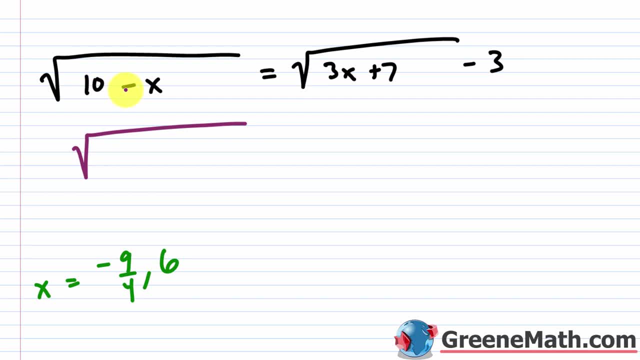 So you'd have the square root of 10 minus a negative 9.25.. Okay, All right, So that's a negative 2.25.. So that's like plus 2.25.. So this would be 12.25 and we're saying this is equal to. we have the square root of three. 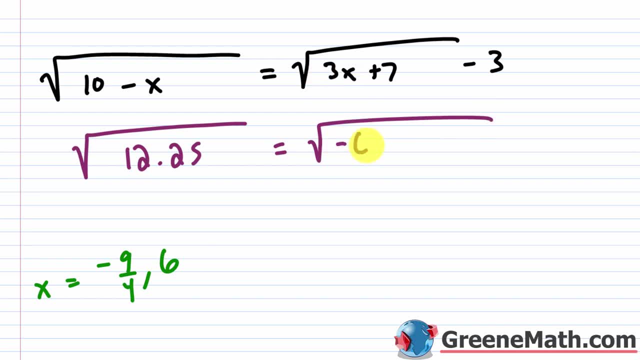 times negative 2.25.. That's going to be negative 6.75 and you're adding that to seven, That's going to give me 0.25, or you can think about that as a fourth. Now the square root of a fourth is going to be a half. 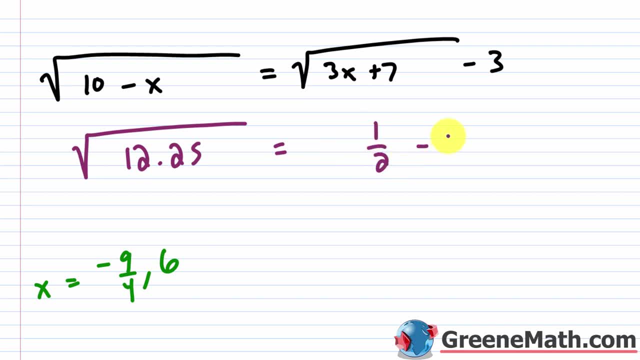 So basically this is 0.5, or you could say it's a half then minus three. We don't really need to go any further here, Because we can see that this side is going to be positive and this side is going to be negative. 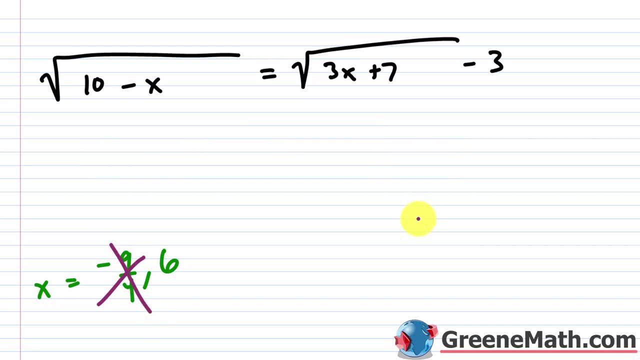 So we know that this is going to be rejected, So this does not work. Okay, The other one's really easy to check. So you have 10 minus six, That's four. The square root of four would be two Over here. three times six is 18, 18 plus seven is 25.. 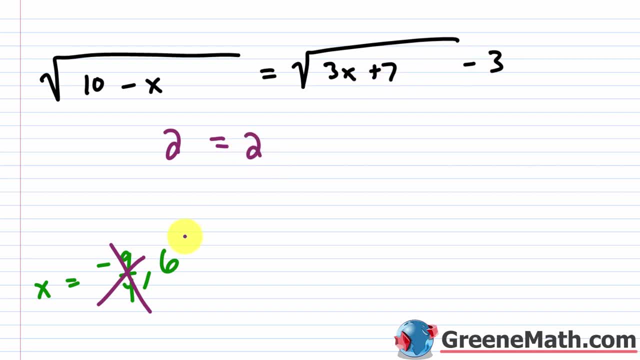 The square root of 25 is five, and then five minus three would be two as well. So this one works as a solution. So six is what we want. So, coming back up here, I'm just going to say X is equal to six. 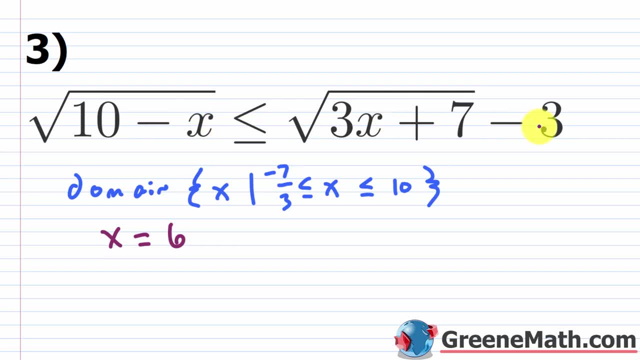 We have all the information we need. I'm going to keep this inequality in this form here. Just bringing everything over to one side in this case doesn't make it any faster for me. Maybe it does for you. It's really personal preference. 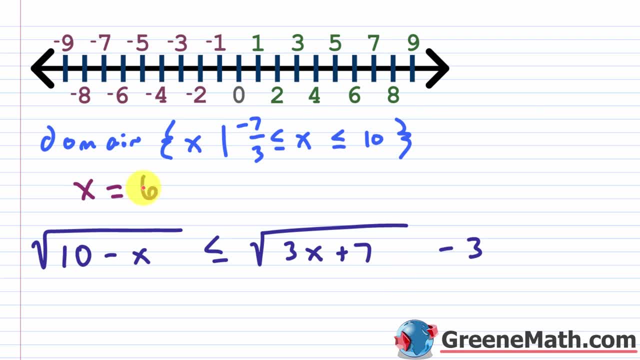 All right, Let's come to the number line now and set up our little intervals. So I'm going to start with six, so that's going to be my boundary here, So I'll make a little vertical line and then also I'm going to think about negative seven. 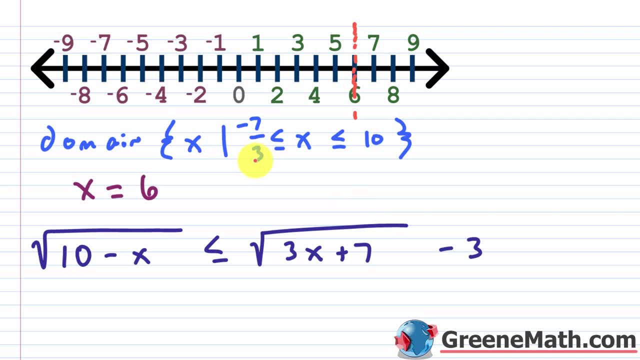 thirds. So if you don't know what that is, again if you don't have a calculator handy, the negative six over three is negative two. So this is basically negative two and a third. So let's just say it's going to be about right here. 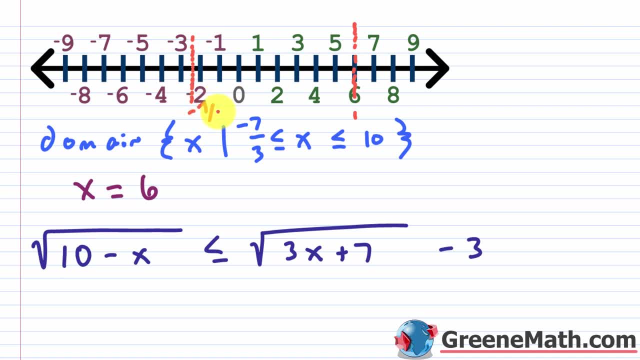 Approximately. It doesn't have to be perfect. We'll say this is negative seven over three, or you can put negative two and a third. whatever you want to do Then for 10, let's put that about right there. Let's make a little vertical line there as well. 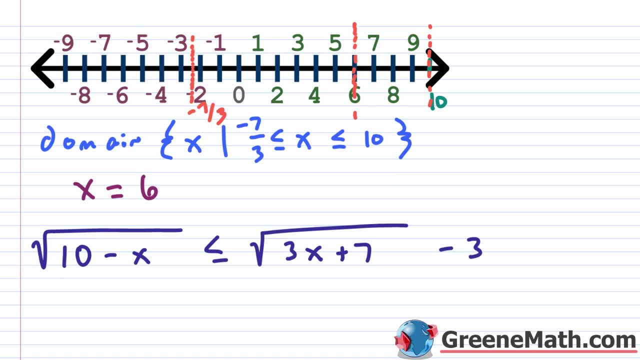 I'm just going to set up my little regions. So let's say that this guy is A, so that's anything that's less than negative seven thirds. Let's say that this is B, so that's between negative seven thirds and six. 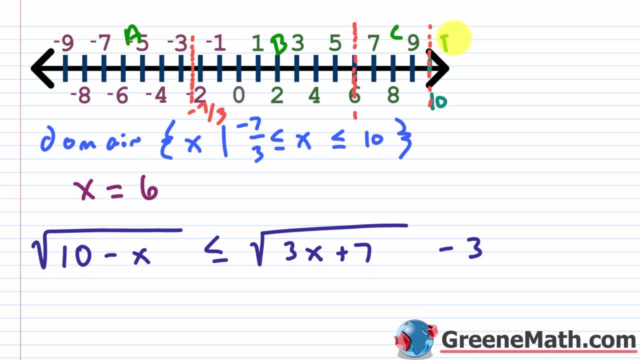 Let's say this is C, so that's between six and 10, and let's say this is D, so that's greater than 10.. So we know for A and D they're automatic rejects right. So they violate the domain. 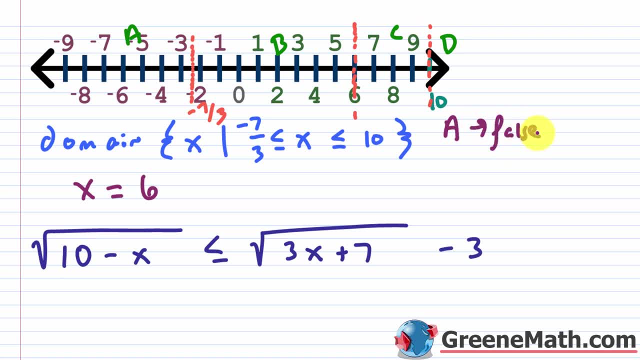 So if I set this up and say A is going to be false and then I'll have B- I've got to check that, C- I've got to check that, And D- we know this is going to be false. 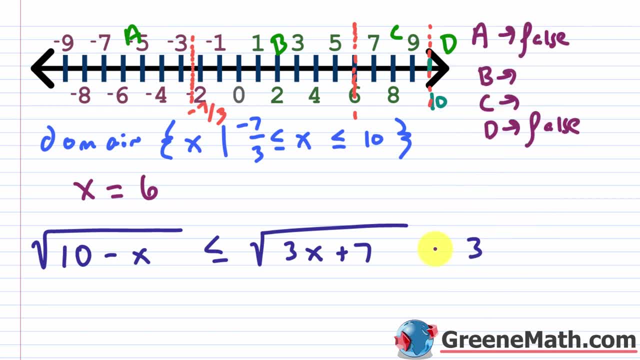 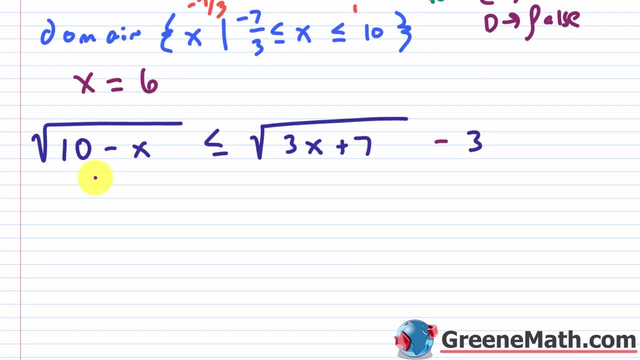 Let me try to slide this up here and I drug my minus sign, So let me put that back in there. So we want to start in region B, So I would pick zero. see what that does. So you would basically have the square root of 10 minus zero. 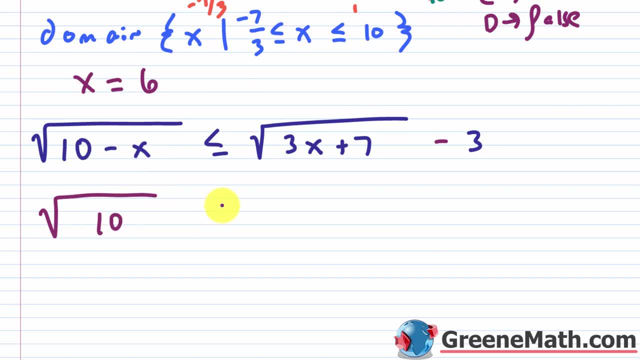 So this is: the square root of 10 is less than or equal to. here, If you plug in a zero, you'd have the square root of basically seven and then minus three. So this is something I would use a calculator for. I'm just going to tell you in advance it doesn't work. 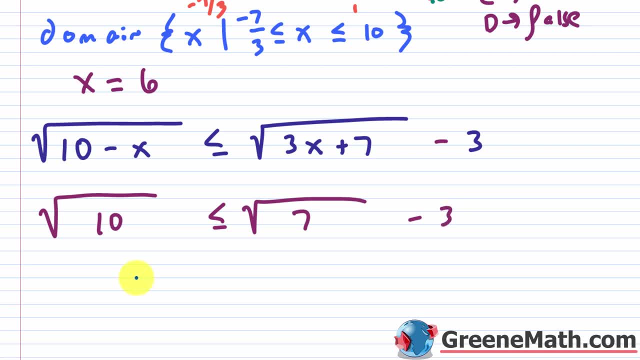 The square root of 10, let's just say that's about 3.16.. So this is an approximation. I'll just say it's about 3.16.. We're saying: is this less than or equal to punch in the square root of seven minus three? 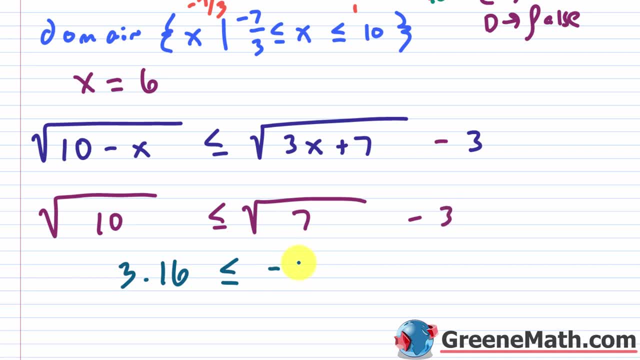 in your calculator. You're going to get a negative value. It's going to be negative, zero point. Let's just say it's 3.5.. We'll just stop there. You can tell because this is positive and this is negative. 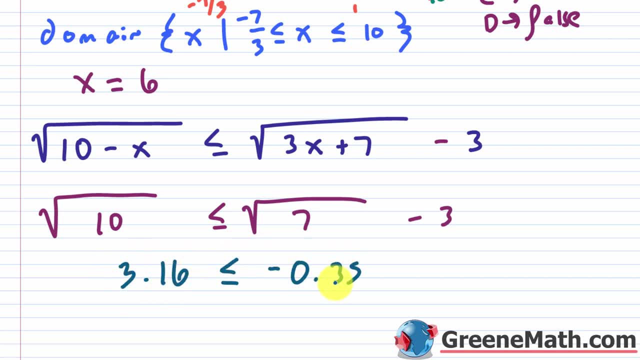 This is a false statement, right? This guy right here is not going to be less than this guy right here, because this is again a positive and this is a negative. A positive cannot be less than a negative and it can't be equal to a negative. 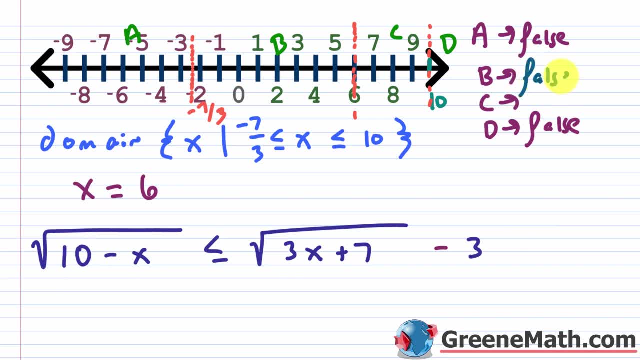 So this is false. So, coming back up, I'll just write that this one is false and then C is going to be true. I'll write that in now and then I'll prove it to you. Let me make that a little bit cleaner there so that it's legible. 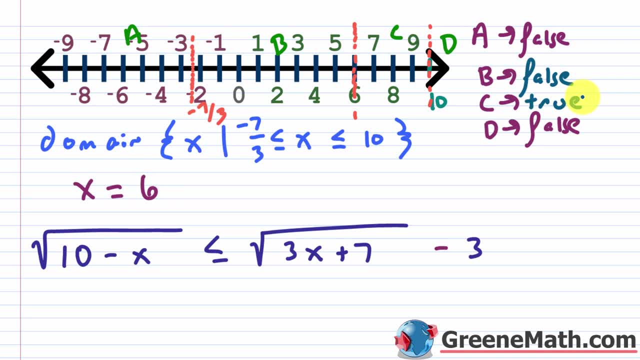 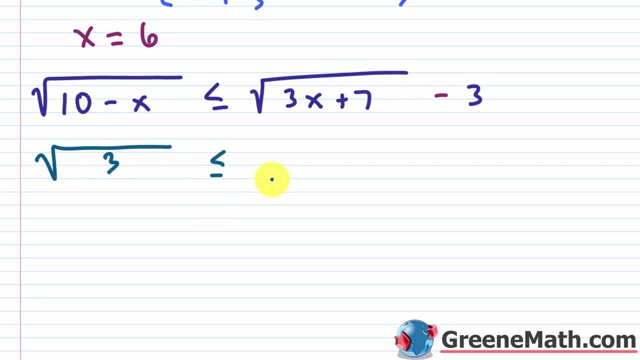 So for C we could pick something like seven, Seven or eight or whatever you want to do. let's just pick seven. So we would have the square root of 10 minus seven. That's going to be three. So the square root of three is less than or equal to. you're going to have the square 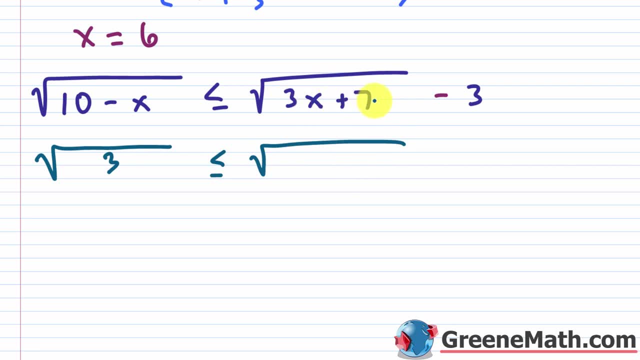 root of three times seven is 21,. 21 plus seven is going to be 28.. So you've got the square root of 28.. Now 28 is four times seven, So you could say this is two times square root of seven, if you wanted to. 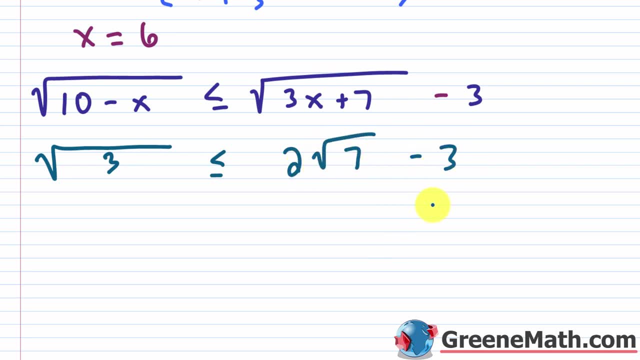 We're probably going to use a calculator, but just for completeness we'll put that in there. So then I have minus three. So punch in the square root of three in your calculator. You're going to get about 1.73.. 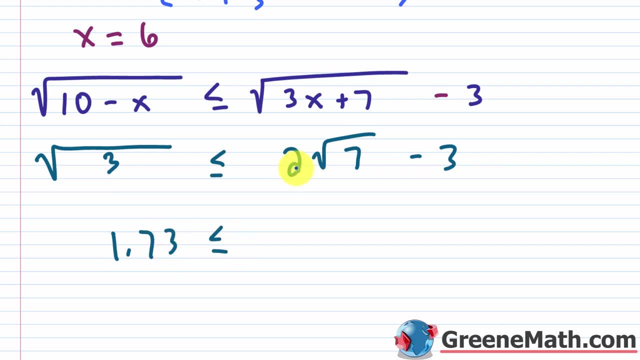 So 1.73,. we'll say this is less than or equal to two times square root of seven minus three. You're going to get about 2.29,. let's say So 2.29.. And again, these are approximations, but it's close enough to where we can see that this. 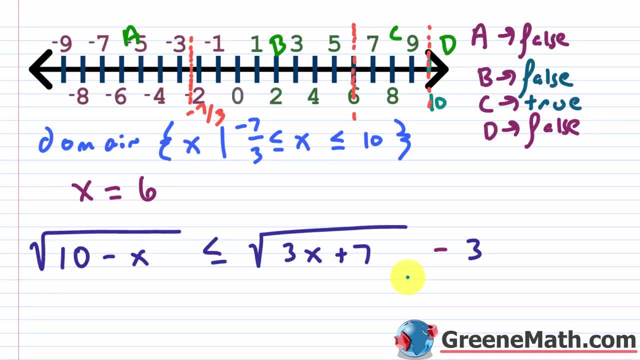 side is less than this side, So it's going to be a true statement. So now that we know that numbers in region C are going to work, we can set up our solution. Let's just start with region C. We'll say X is greater than six and less than 10.. 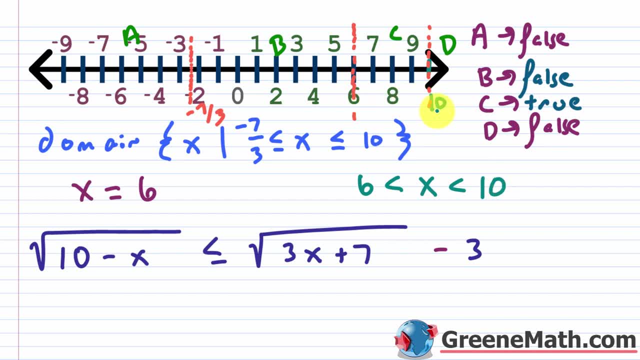 Now we want to consider six and 10.. Let's first think about six. We have over here this X equals six, Remember this was the solution for our related equation. Well, here we have this non-strict inequality. So if I plug in a six for X, I'm going to get the same value on the left as I get on. 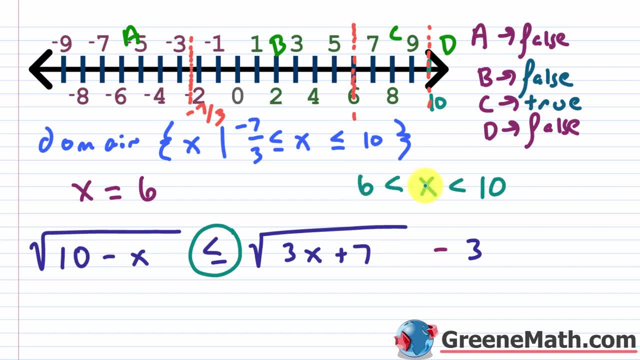 the right. So that means six would be included in the solution for this inequality. So let's go ahead and make this into a less than or equal to. Now let's think about 10.. Remember, on this side of six we're going to be in the solution region. 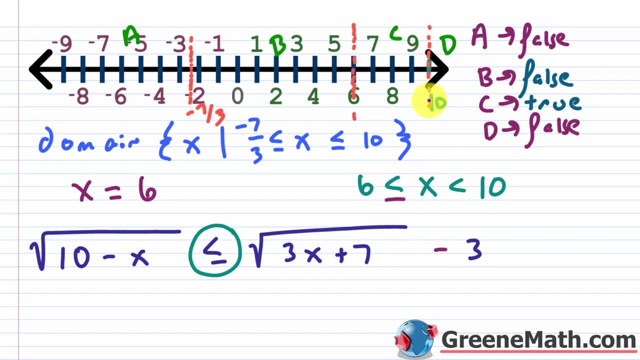 So anything greater than six. What stops us is that Anything greater than 10 is not going to work because it violates the domain. But 10 itself does not violate the domain, So it will be in the solution set. So I'm going to go ahead and say this is a less than or equal to. also. 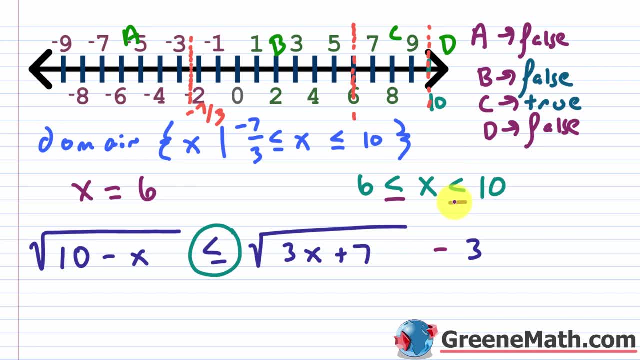 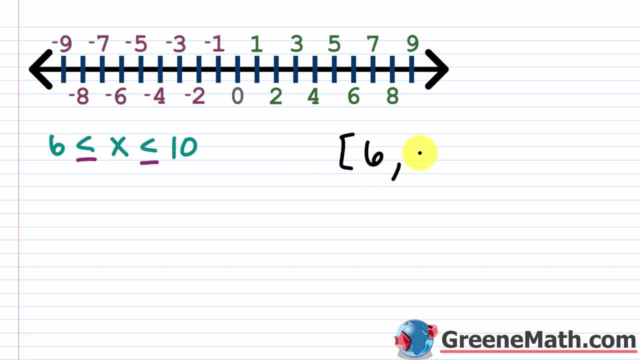 So here X would be greater than or equal to six and less than or equal to 10.. All right, So let's put this in interval notation. So I'll just say we'll have a bracket there and then a six, a comma. 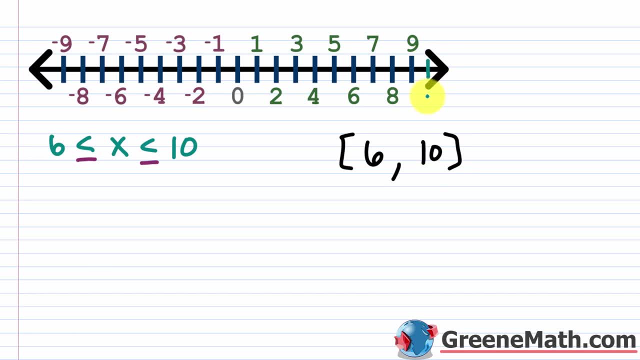 We'll put a 10 and then a bracket. Now, graphically, let me start by putting a little notch here for 10.. And then I'm going to use a bracket. I'm going to use a bracket here at six and I'm going to use a bracket here at 10.. 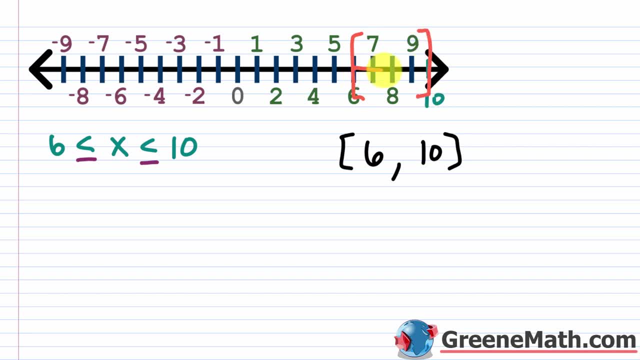 Again, if you want to use a filled in circle, that's up to you and that'll just shade everything in between there. So basically we're saying that X can be any number, that is six, and then going up to and including 10.. 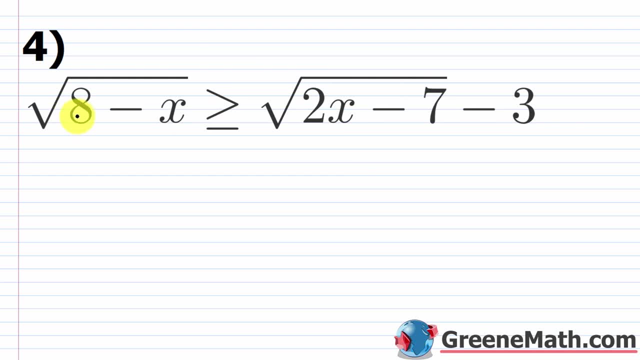 All right, Let's take a look at problem number four now. So we have the square root of eight minus X. This is greater than or equal to the square root of two X minus seven. Then we have minus three. All right, Let's start with the domain. 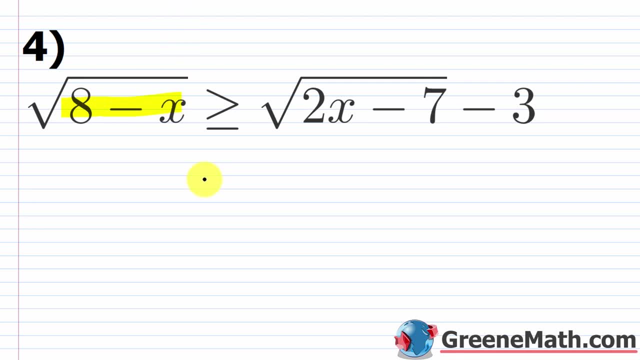 So I'm going to take this radicand here, which is eight minus X, Okay, And we'll say that this is greater than or equal to zero. Then I'm going to say, and I'm going to take my other radicand, which is two X minus seven. 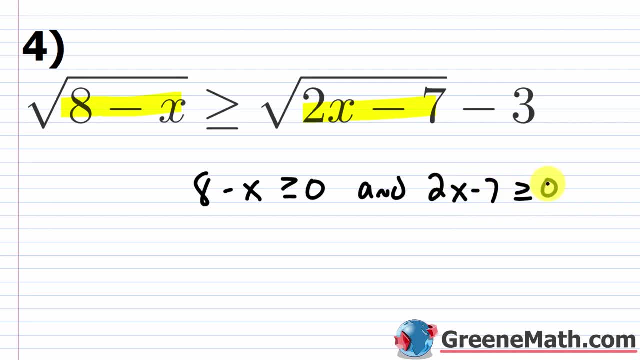 And again, we'll just say that that guy needs to be greater than or equal to zero as well. Okay, So solving this one is pretty simple. I would just add X to both sides of the inequality You would get. eight is greater than or equal to X. or you could flip that around and say: 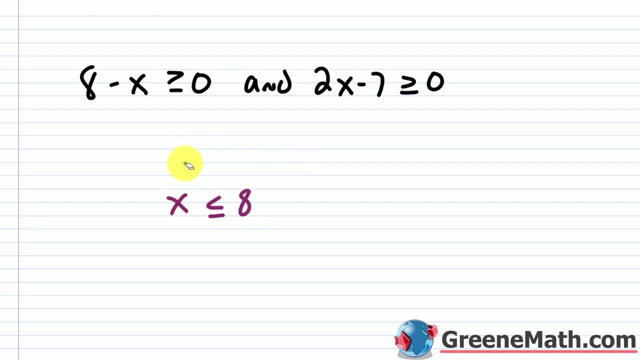 that X is less than or equal to eight. Okay, For this one over here, what I would do is add seven to both sides of the inequality. Let's cancel that away. We'll say that we have two. X is greater than or equal to seven. 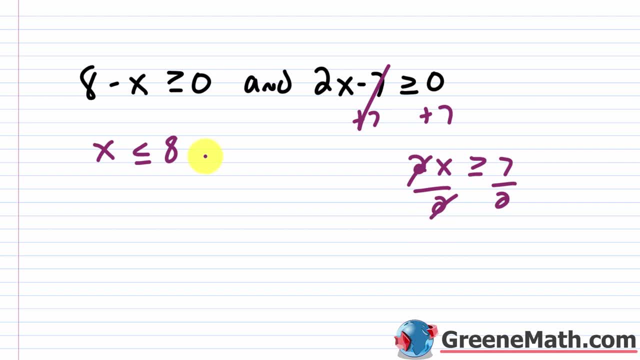 Let's divide both sides of the inequality by two, We'll cancel that, And so I'll write my keyword and here, and I'll say: X is greater than or equal to seven halves, or in decimal form you could put 3.5.. 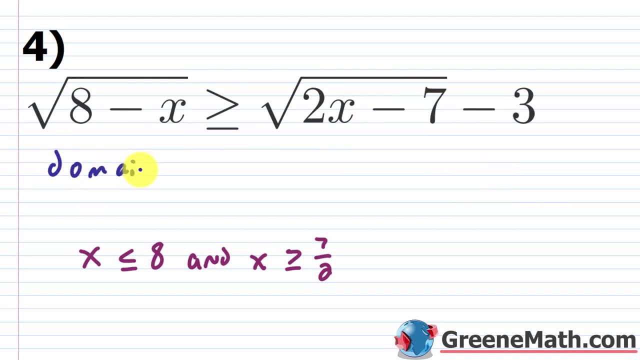 So let's write our domain. So we'll say that the domain here is going to be the set of all X, such that we're going to have. X is going to be greater than or equal to our seven halves, And it'll be less than or equal to eight. 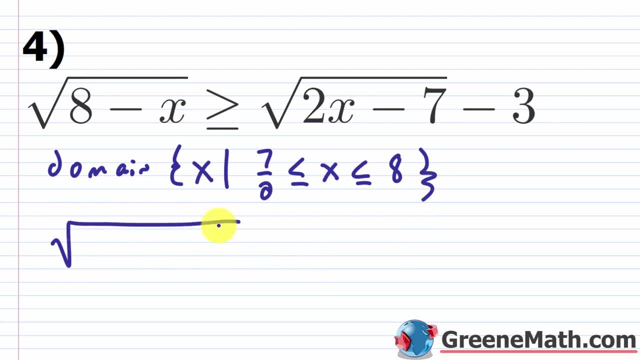 Okay, So let's solve the related equation. We'll say the square root of eight minus X now is equal to. we'll say the square root of two X minus seven, and then we'll have minus three. Okay, So I'm going to square both sides so I can get rid of the square root on the left. 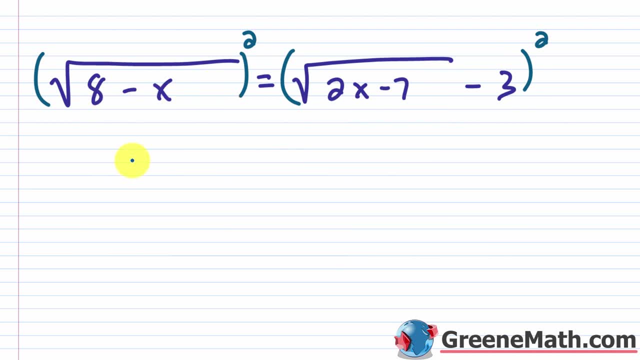 Unfortunately, I'll still have a square root on the right, but we'll deal with that in a moment. So I'll just have the radicand here. This is eight minus X and this is equal to here. I'm going to square this guy. 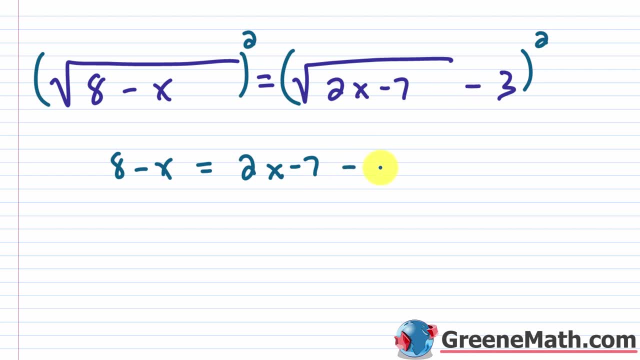 So that would be two X minus seven. Okay, Then you have the minus. You have two times this guy, times this guy two times three is six, and then times your square root of two X minus seven and then, squaring the last guy, if I square three. 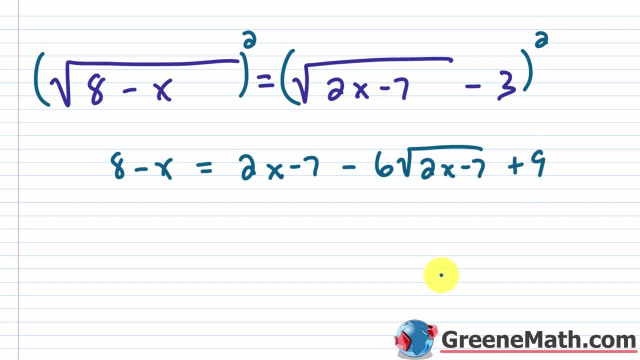 I get nine. So this is plus nine. Okay, So I can clean this up just a little bit Again. I'm trying to isolate this guy right here, So I can say that negative seven plus nine is positive two. Let me just erase that from here and just put this as a two. 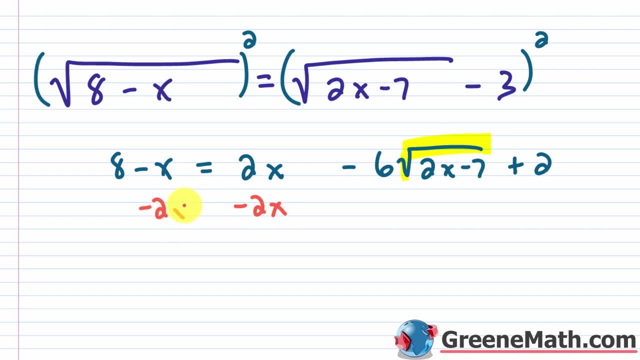 And then what I'm going to do is subtract two X away from each side, And then I'm going to also subtract two away from each side, And let's cancel this and let's cancel this. So let's say that we have eight minus two, that's six. 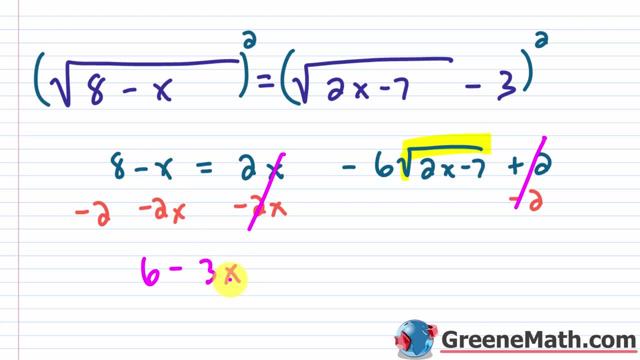 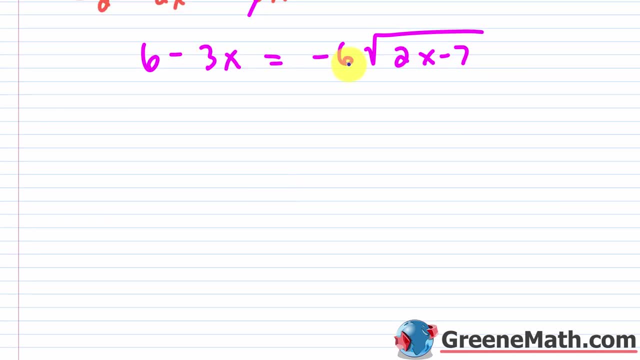 And then basically negative X minus two X would be negative three X and this equals negative six times the square root of two X minus seven. Now, like we've talked about before, you could divide everything by negative six to make this side simpler, but you're going to end up with a fraction over here and you probably 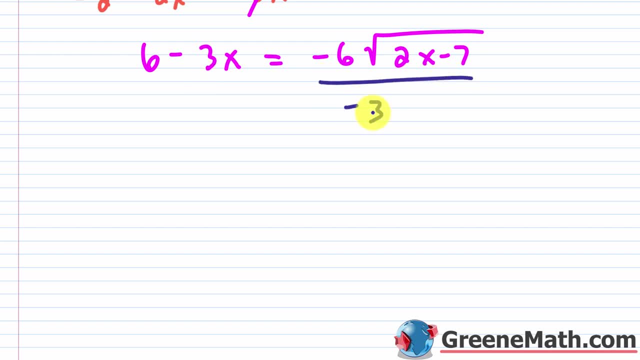 don't want to work with that, So I'm going to just divide everything by negative three. I think that's just going to make things a little bit easier for you. So six divided by negative three is negative two, then negative three divided by negative. 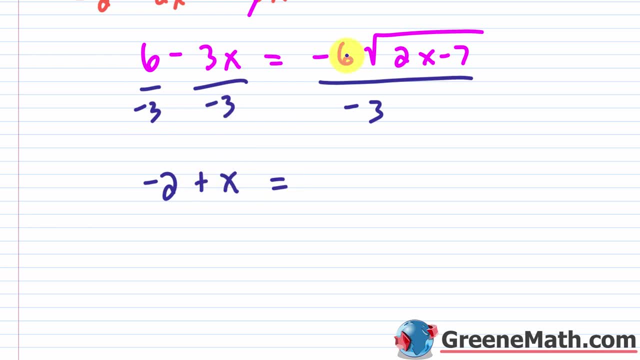 three is one. So this would just be plus X, And this would be equal to negative six over negative three is two, And then this is times, the square root of two: X minus seven. Now, over here, I would just flip this around and say it's X minus two. 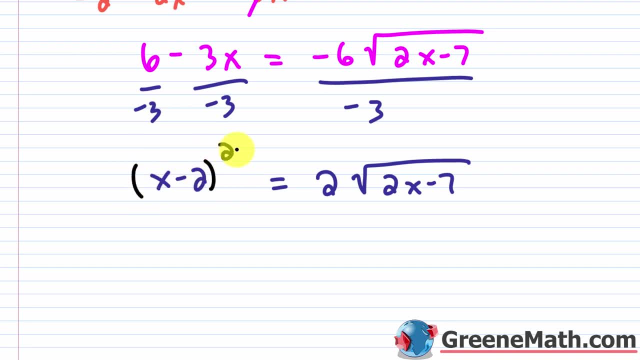 And then I would just square both sides. So square this side and then square this side. Over here just use your formula. So this is X squared minus two times X times two. So this is minus four X, Then plus two Square. 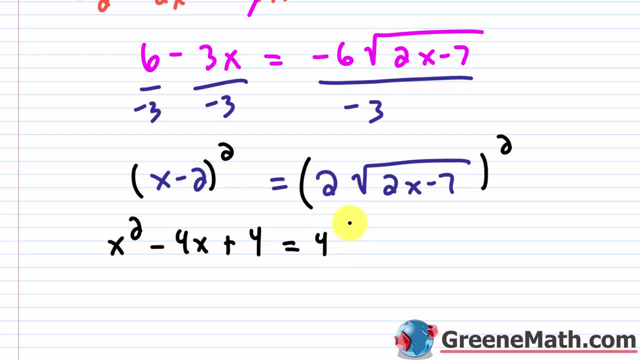 Square. Square is four And this equals square two. That's four. Then you're going to wrap this in parentheses. When you square this, remember you get two X minus seven, but you need to multiply four by each term there. So four times the quantity two X minus seven is what you're going to get there. 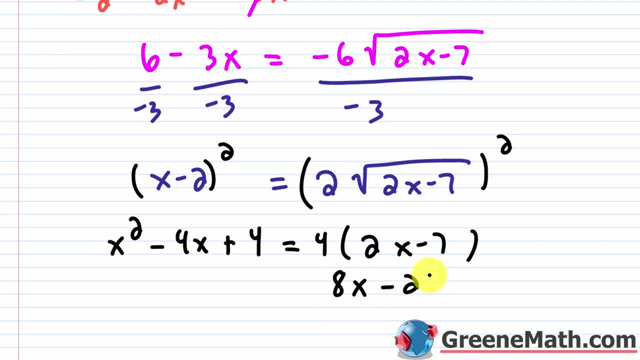 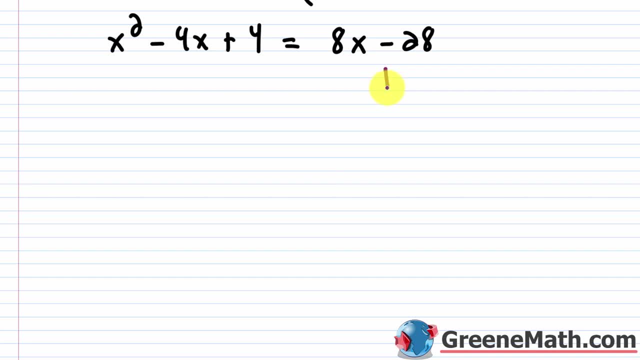 And if you go through and distribute, you would have eight X and then minus 28.. So let me erase this and just drag this up here. All right, So a pretty simple quadratic equation to solve. I'm just going to add 28 to both sides and then cancel this away. 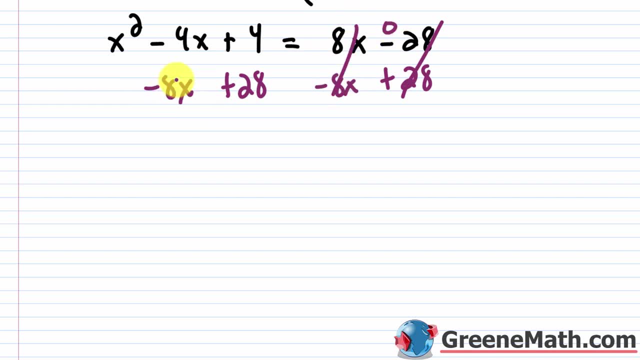 Subtract eight X away from each side. cancel this away. let's put this as zero. we'll have x squared and the negative 4x minus 8x is negative. 12x. 4 plus 28 is 32, so plus 32 and this equals zero. very easy to factor this and solve it. 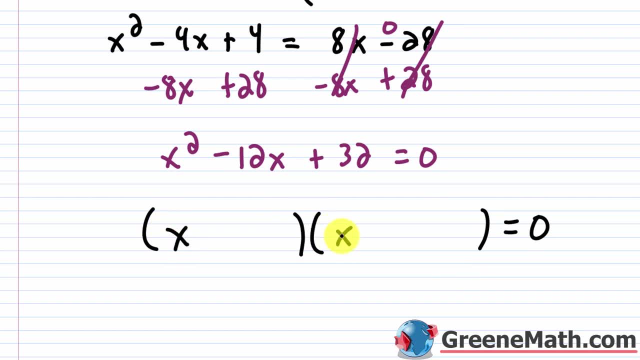 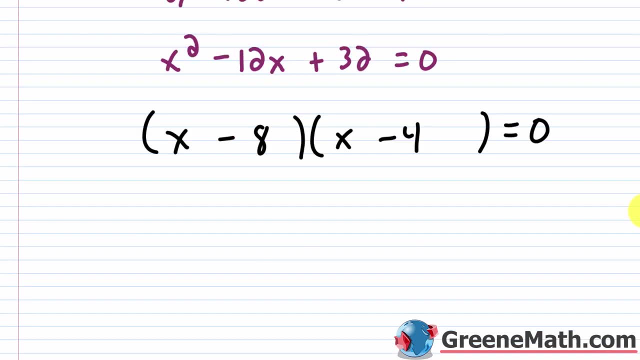 that way. so let's do that. so we'll put an x here and an x here, two integers that sum to negative 12 and have a product of positive 32. that's going to be negative 8 and negative 4. so here we would just say x minus 8 is equal to zero, or x minus 4 is equal to zero. let's add 8 to both sides of. 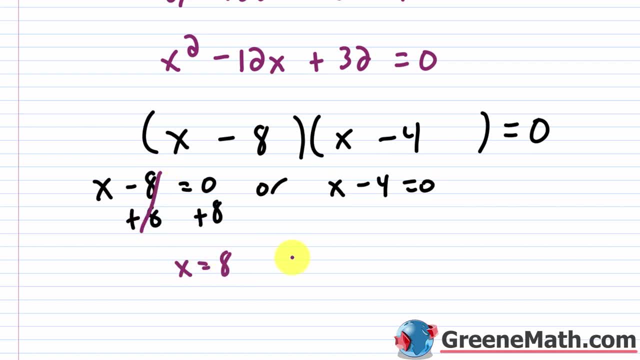 the equation. let's cancel this away and say x is equal to 8. let's add 4 to both sides of the equation. cancel this away. we'll say x could also be 4. but again, these are proposed solutions so we have to check them. all right. so, coming back, i'm just going to tell you in advance that 8 works. 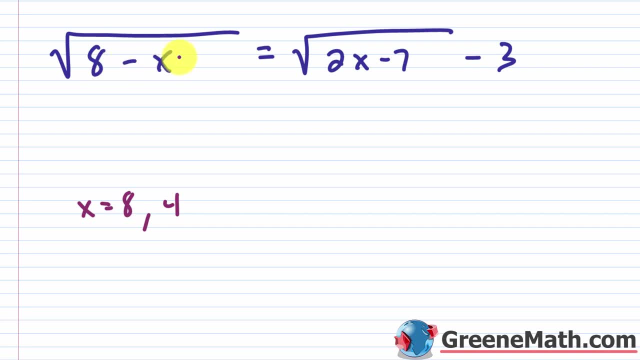 and 4 doesn't. if you plug in an 8 for x, you get 8 minus 8, which is 0. square to 0 is 0 and this equals 2 times 8 is 16. 16 minus 7 is 9. 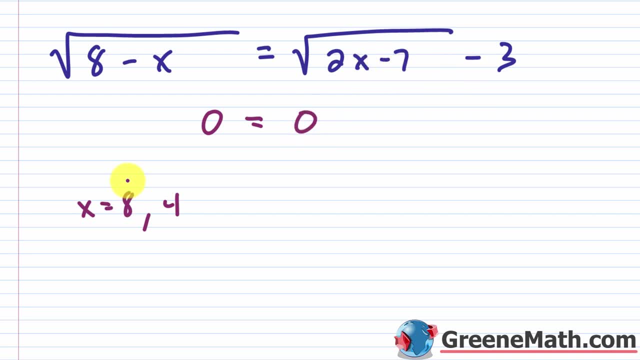 square root of 9 is 3. 3 minus 3 is 0, so this one works. 4 does not work. so here you have 8 minus 4, which is 4. square root of 4 is 2, and this should be equal to 2 times 4 is 8. 8 minus 7 is 1. the 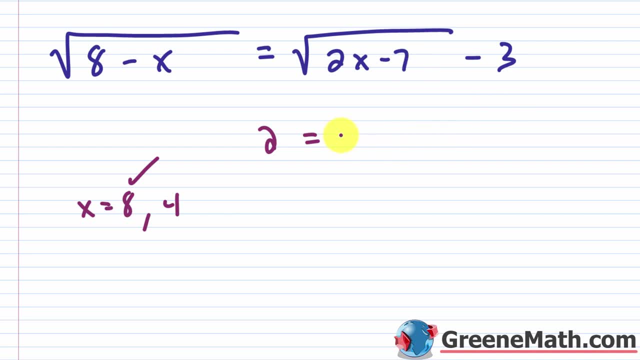 square root of 1 is 1, and then 1 minus 3 is negative 2. so this solution here of x equals 4 is extraneous, so we're going to reject that one. so we just want this: x equals 8. so coming back, 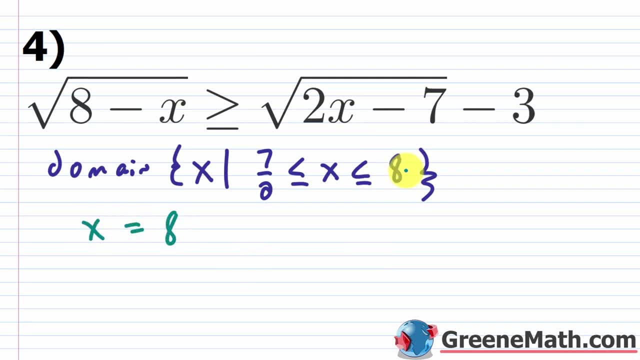 up here. i just want to put x equals 8. now you have an 8 here and an 8 here, so we're going to reject that one. so we just want this: x equals 8. so, coming back up here, i just want to put x equals 8. now you have an 8 here and an 8 here, so we're going to reject that one. so we're. 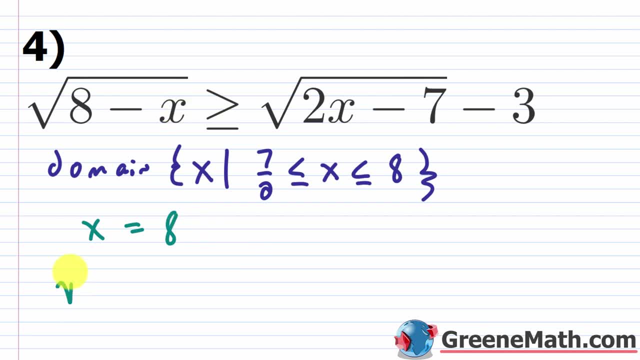 That's going to make things a little bit simpler. Let me copy this real quick. So we have the square root of 8 minus x is greater than or equal to. we have the square root of 2x minus 7, and then minus. 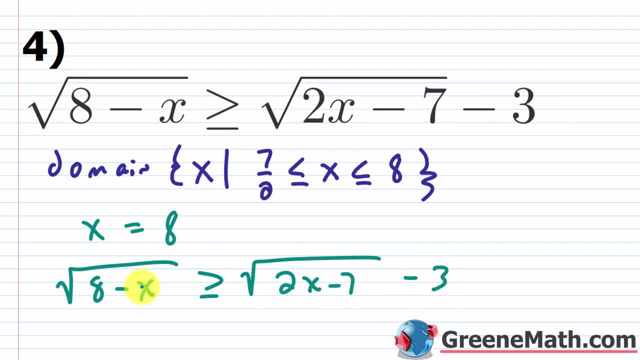 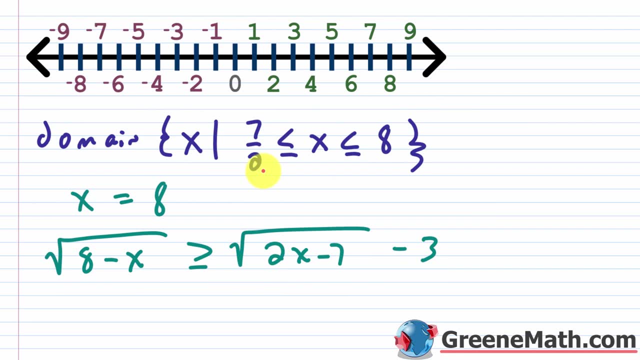 3.. Once again, I'm not going to write everything on one side. When it gets complex like this, I don't think it helps that much. You just pretty much have to use a calculator. Alright, so, coming to the number line, let's think about 7 halves, which in decimal form is 3.5.. So let's just say: 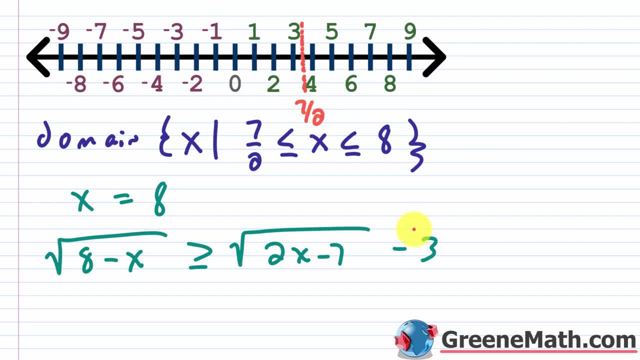 that's about right here. It's not perfect, but that's close enough. And then we have 8.. So let's put that there, And that's basically it. So we're going to have three intervals here. Let's call this A, let's call this B, let's call this C. Now for A and C, those are automatically going to be. 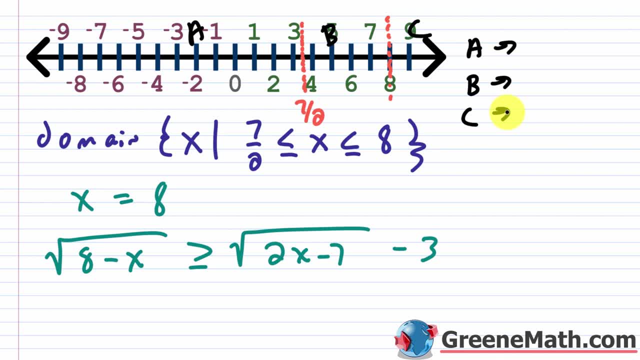 rejected because they violate the domain right. A is going to be anything that's less than 7 halves, So this is going to be false. Then for B, we have to check it. That's between 7 halves and 8.. Then for C, we're going to reject because that's anything greater than 8.. Again, that. 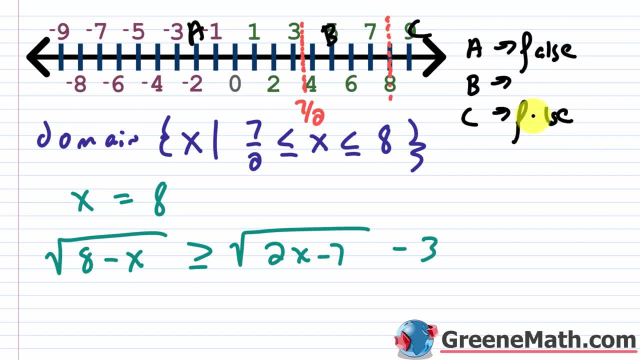 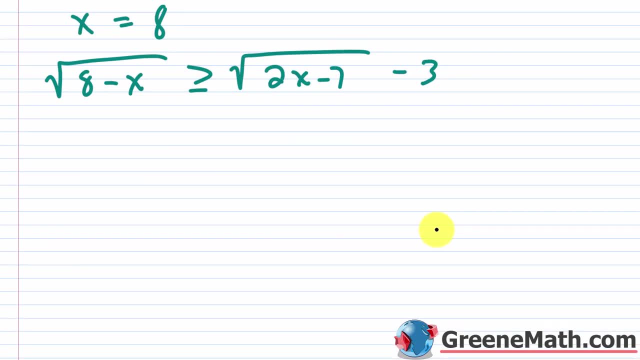 violates the domain, So this is automatically going to be false. So really, we just want to check something. in B You could just grab something like, let's say, 4.. I think that'd be pretty easy to work with. Now, you might remember from the equation when we 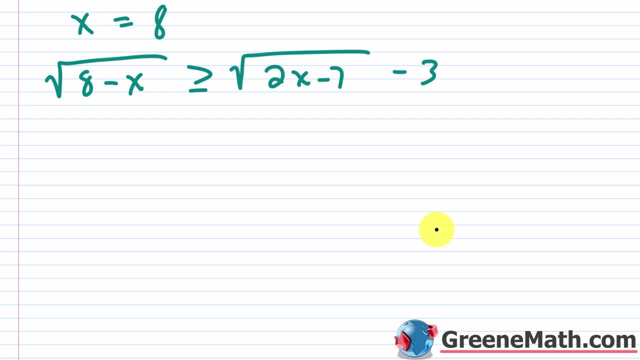 plugged in 4, we got 2 on one side and we got negative 2 on the other side. But let's just go through it again. So if I plug in a 4 there and I plug in a 4 there, we're going to get 8 minus 4,. 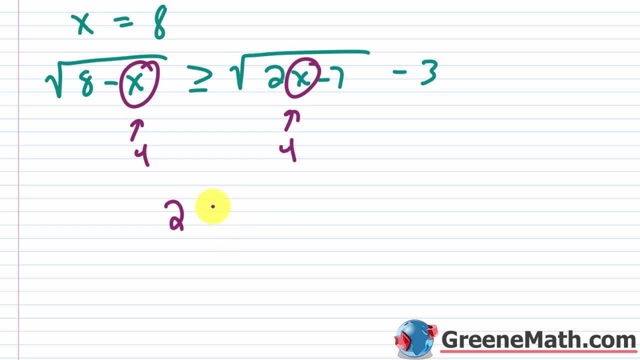 which is 4, square root of 4 is 2.. So that's the left-hand side. This is greater than or equal to, 2 times 4 is 8,. 8 minus 7 is 1, square root of 1 is 1.. So this is 1 minus 3, which is negative 2.. 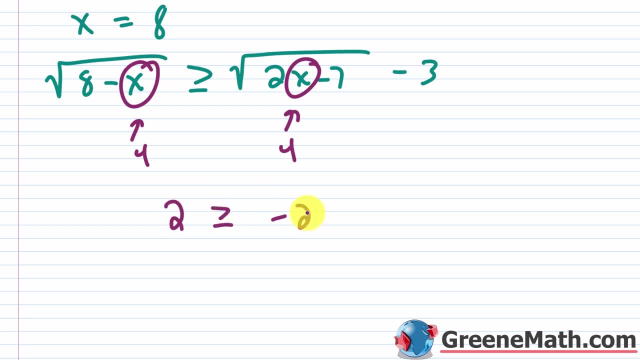 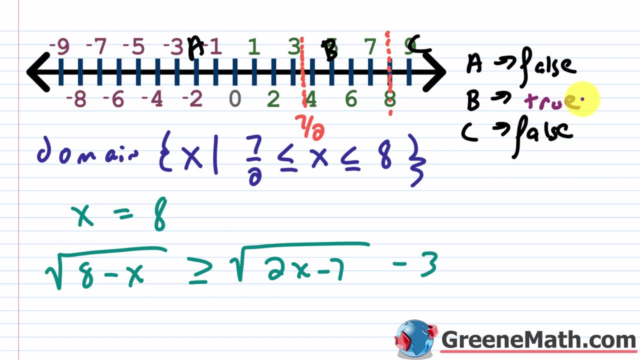 And this is a negative, And a positive is always greater than a negative. So this is definitely true. right 2 is greater than negative 2.. We can say that this is true for region B, So getting our solution is pretty easy. We just grab region B, So we'll say that x is greater. 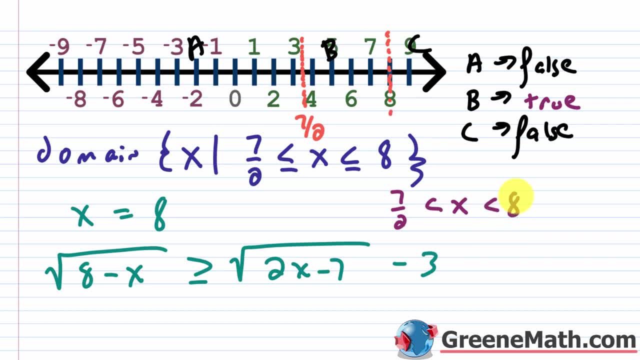 than 7 halves and less than 8.. And we're going to think about 7 halves and we're going to think about 8.. Now, first and foremost, does 7 halves work? Well, yeah, if I'm less than 8, I'm going. 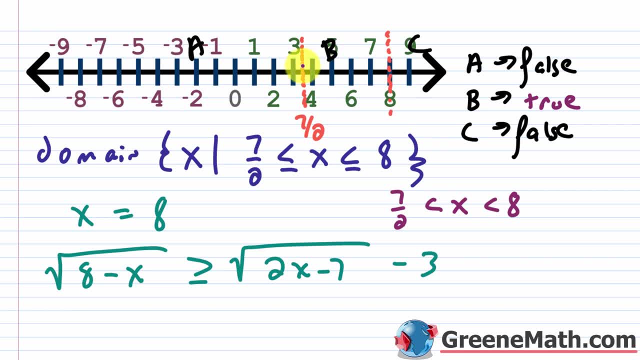 to work, But again, anything less than 7 halves. that violates the domain. So we're going to the domain, but 7 halves does not. So this is going to be included. So x here would be greater than or equal to 7 halves. So we want this right here to be less than or equal to. Now does 8. 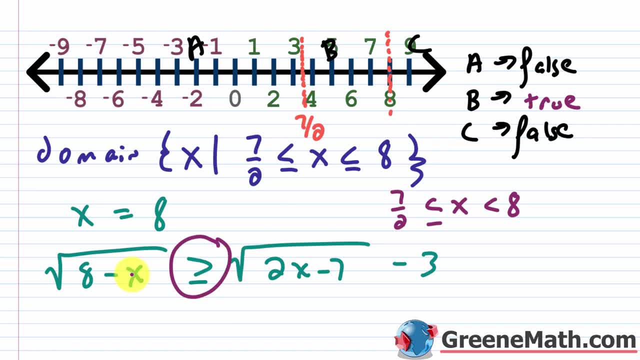 work Well. again, this is a non-strict inequality. So if I plugged in an 8, the left and the right sides would be equal, So this would work as well. So I want this to be a less than or equal to also. 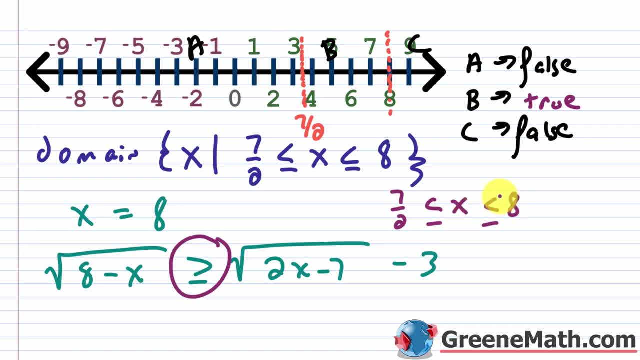 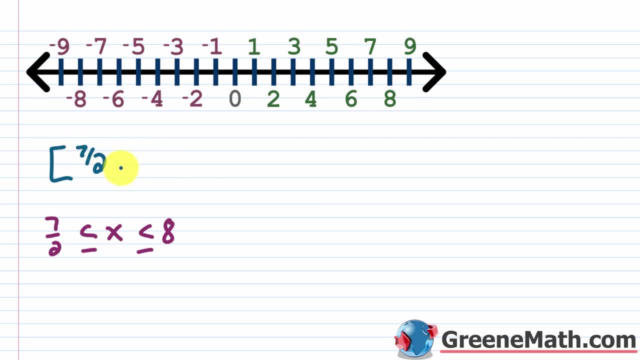 So here x would be greater than or equal to 7 halves and less than or equal to 8.. So, coming back here, I'll just write this in interval notation: So we'll put a bracket, 7 halves, comma 8, and then a bracket, And then let me put my notch in. 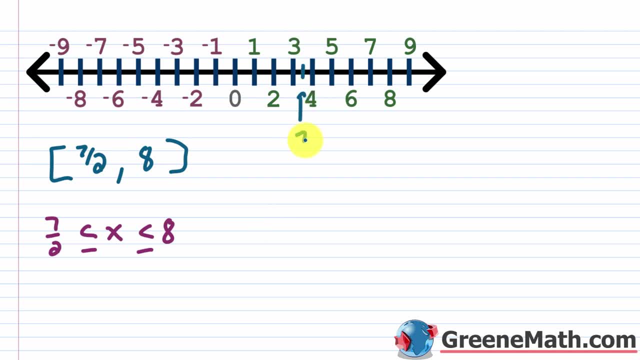 here for 7 halves again. So let's just say it's about right there. That's going to be 7 halves for us, And I'm just going to use a bracket. there Again, you can use a filled-in circle, And then I'm going to use a bracket at 8. And then just shade everything in between. 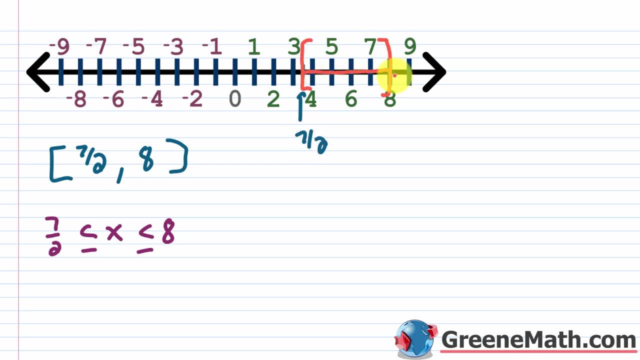 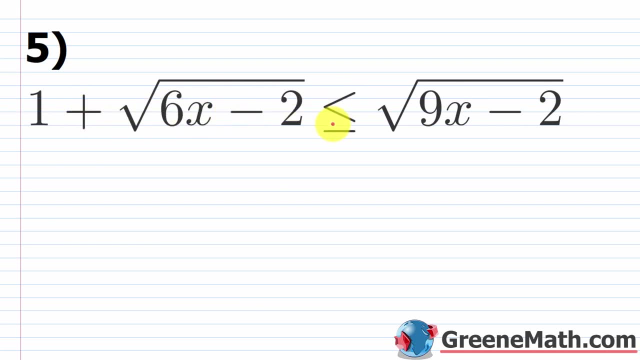 So from 7 halves x can be that going up to and including 8.. All right, let's take a look at problem number 5 now. So we have 1 plus. the square root of 6x minus 2 is less than or equal to. 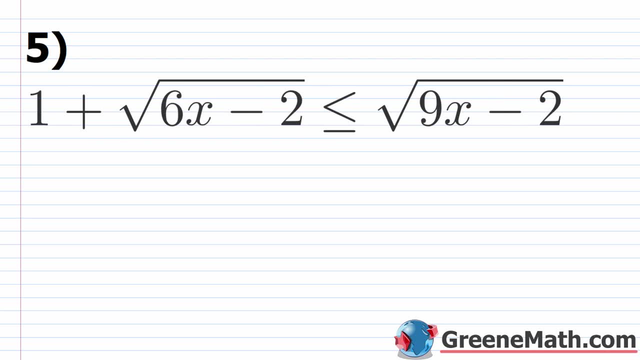 We have the square root of 9x minus 2.. And what I'm going to do is first find my domain. So I'm going to take this 6x minus 2, this radicand here And I'll say that that needs. 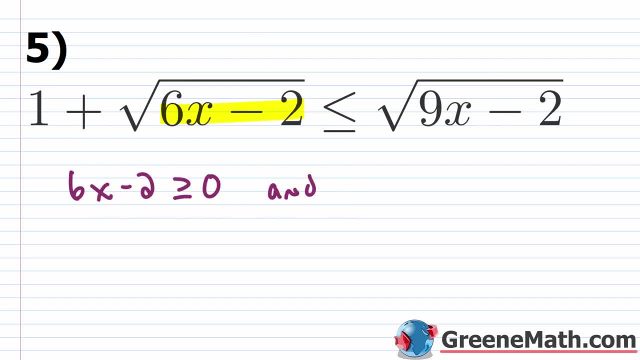 to be greater than or equal to 0.. Then I'll use my keyword and I'll work with my other, radicand, which is going to be this: 9x minus 2.. And again, this has to be greater than or equal to 0 as well. 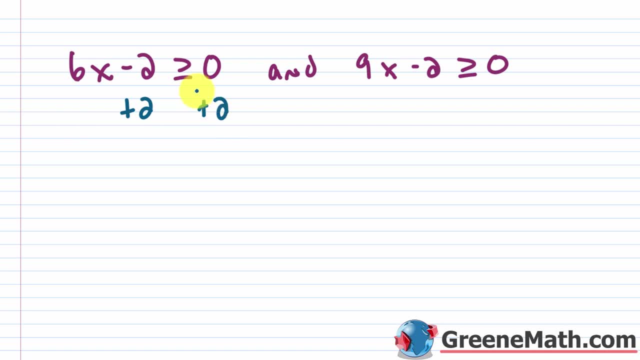 OK, on the left let's add 2 to both sides of this inequality. We'll cancel this and say 6x is greater than or equal to 2.. From here let's divide both sides of the inequality by 6.. 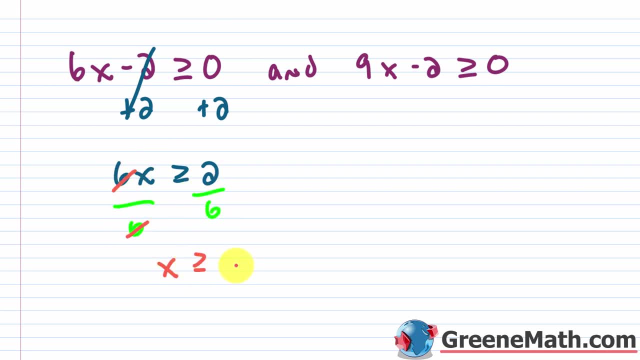 We'll cancel this away and say x is greater than or equal to 2 over 6 is basically going to be 1 third. And then let me write my keyword and here And over here, I'm just going to add 2 to. 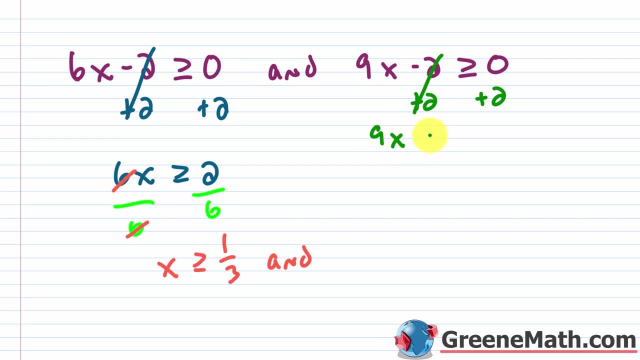 both sides of the inequality. We'll cancel this. We'll have 9x is greater than or equal to 2.. From here, we'll divide both sides of the inequality by 9.. We'll cancel this, So we'll have x is greater. 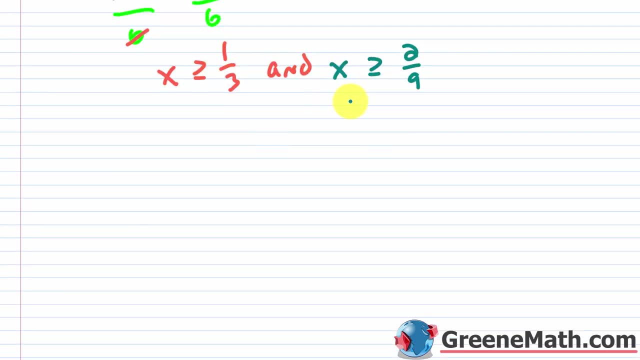 than or equal to 2 ninths. Now, this one is a little bit tricky, when you see it, if you're not used to working with compound inequalities. Basically, since you have a greater than or equal to, and then another greater than or equal to, you're going to take the more restrictive one. 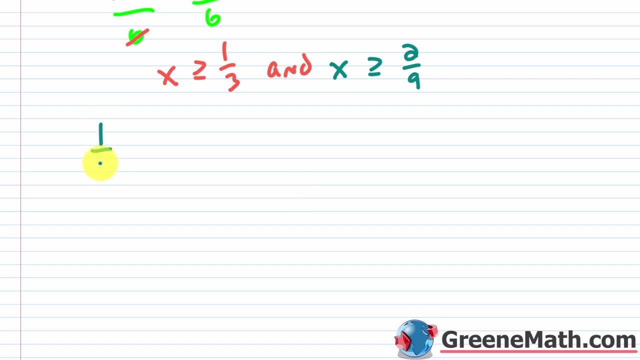 So how do we figure out which one's more restrictive? Well, think about 1, third as a decimal. Just punch that into your calculator. You're going to get 0.3, where the 3 repeats forever, right, You get 0.333.. That 3 is going to continue forever and ever and ever. Then for 2: 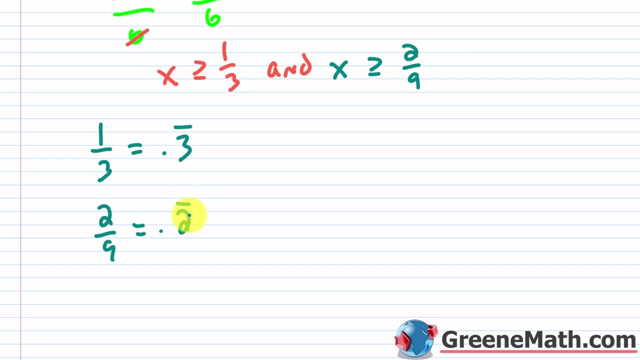 ninths, punch that into your calculator, You get 0.2, where the 2 continues forever. So 0.2222,, so on and so forth. Now, thinking about this again, which one's more restrictive? Well, 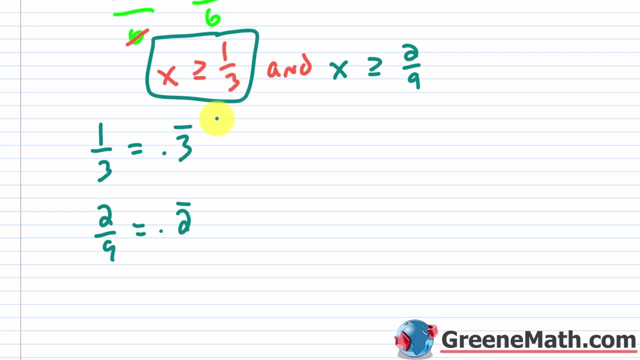 this one will be right Because this one is larger, so it's to the right of the other one. You can even look at this on a number line if you're confused by this, and just think about which one's more restrictive or which one includes fewer numbers. So let's say that this is. let's say 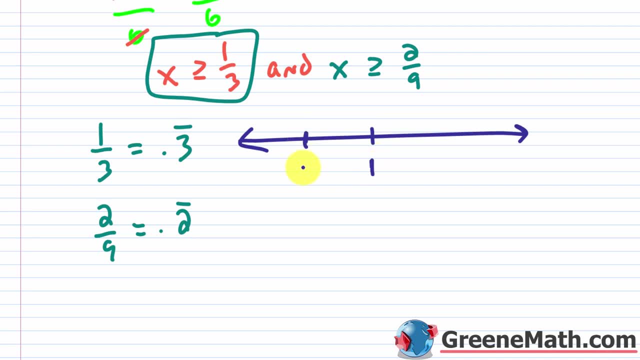 1, okay, Wherever you want to put it, it's fine. And let's say that this is 0 here. Well, if we have something like 1 third, let's just say that that's going to be somewhere about. let's say: 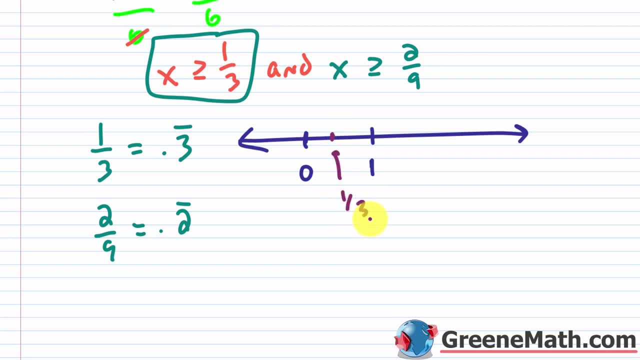 right there. So let's say this is 1, third, And then what's going to happen is 2 ninths is going to be to the left of that. So let's just say it's right here. Again, it doesn't matter if 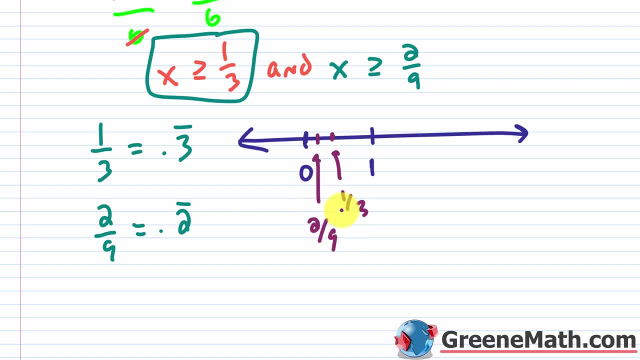 it's exact. Let's just say this is 2 ninths. You're just going to see that 2 ninths is to the left of 1 third, And so if we were considering this guy right here, right, that would include more numbers. 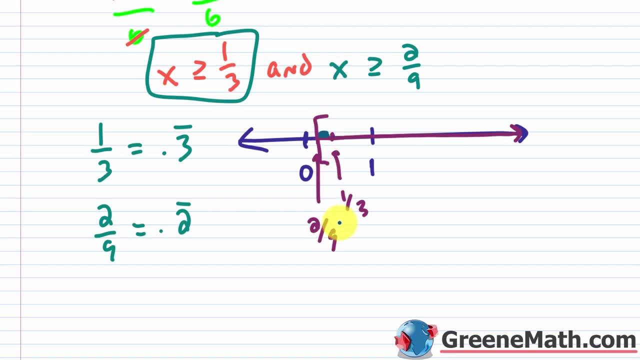 So this would include these numbers right here, right, which would not be included in the other one. So that's important to understand. So we want to go with the more restrictive one, because we have and because it has to work in both. So we want: x is greater than or equal to 1 third. 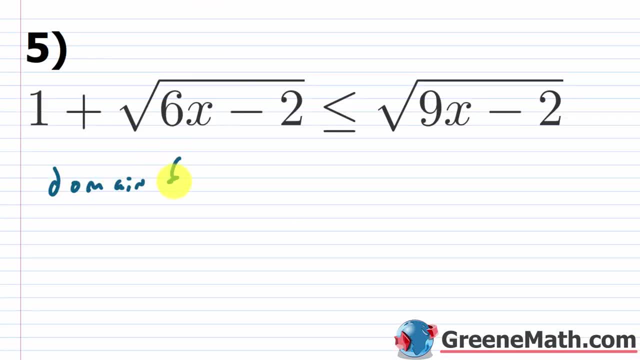 Let's come back up here and write our domain and say that it's going to be the set of all x, such that x is greater than or equal to 1 third. Okay, so now let's solve the related equation. So 1 plus the square root of 6x minus 2.. This is 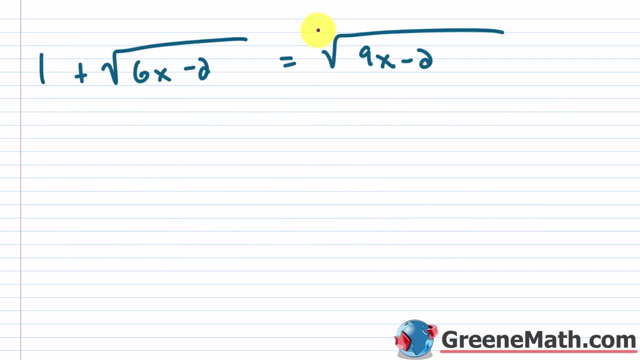 equal to the square root of 9x minus 2.. What I'll do here just immediately square both sides So I can get rid of this radical on the right. Unfortunately, I'll still have a square root on the left, So on the left it's our formula. So 1 squared is 1 plus 2 times 1 times this, So 2. 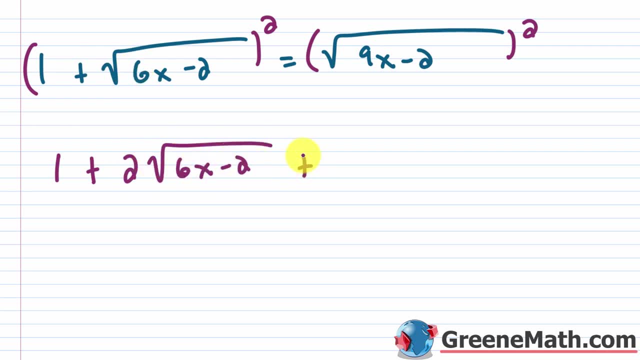 times square root of 1 squared is 1 plus 2 times 1 times this, So 2 times square root of 1, squared, root of 6x minus 2.. Then plus this last guy squared, which is 6x minus 2.. This equals, if I: 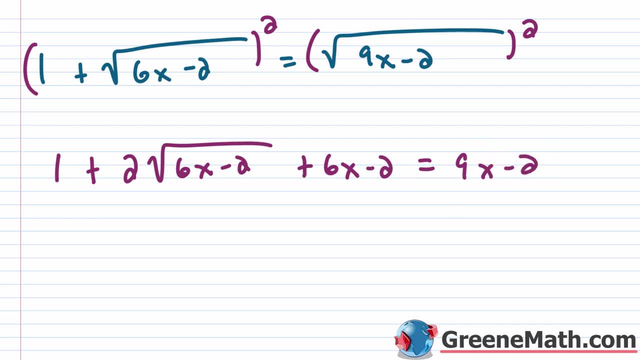 square this guy, I get the radicand, which is 9x minus 2.. So again, I need to isolate this guy right here. Pretty easy to do at this point, I think. So you see that you have negative 2 here. 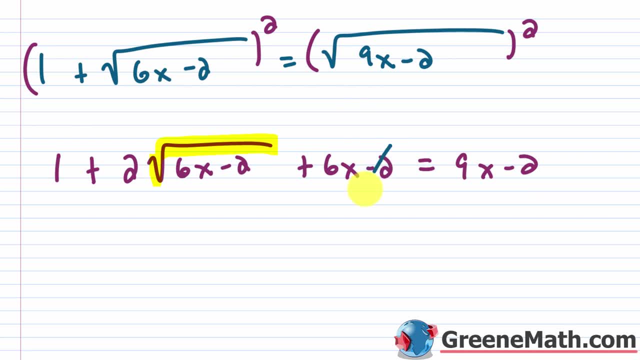 and negative 2 here. You could just get rid of it from each side. I think that's probably the easiest thing to do, And then you could just subtract one away from each side. Let's cancel that from there. And then let me subtract 6x away from each side. Cancel that from there, So you. 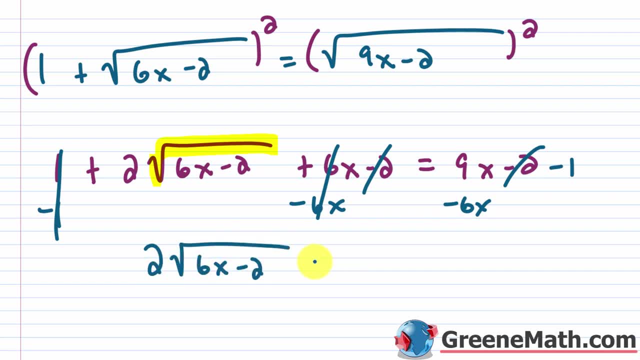 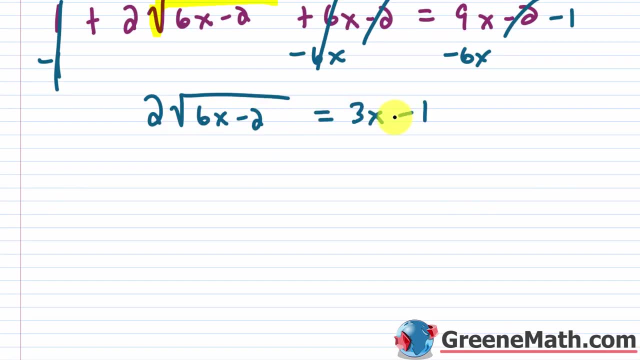 have 2 times the square root of 6x minus 2.. This equals 9x minus 6x is 3x, And then basically minus 1.. Now at this point you could divide both sides of the equation by 2, so that this is a little bit. 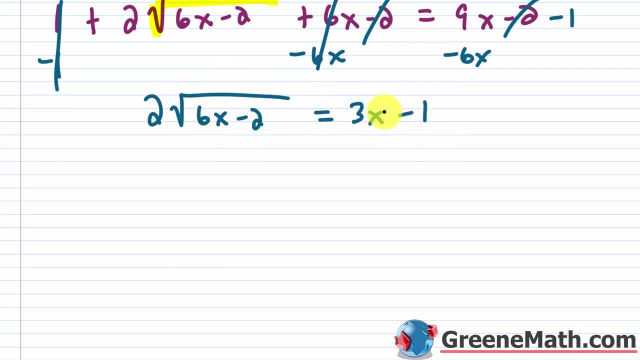 easier to work with, But you're going to make this one more complicated. So it's really a trade-off. Okay, which one do you want to struggle with? I'm just going to leave it as is And I'm going to square both sides And essentially I'm going to say that this is 4 times the quantity, 6x minus 2.. 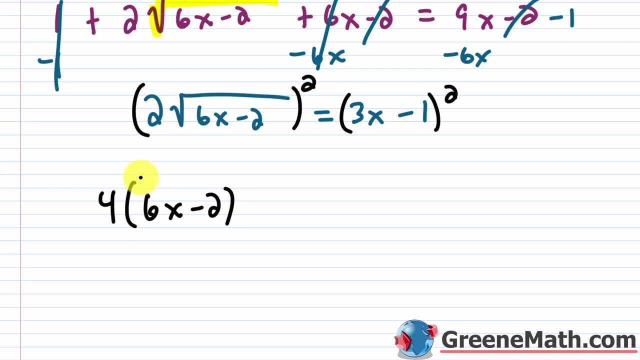 So again, I can't stress this enough: Make sure, when you do something like this, that you use parentheses here. The 4 needs to multiply by the 6x and the negative 2. Then this equals- I'm going to square 3x, That's 9x squared, And then minus 2 times 3x, times 1 is going to be 6x, And then plus. 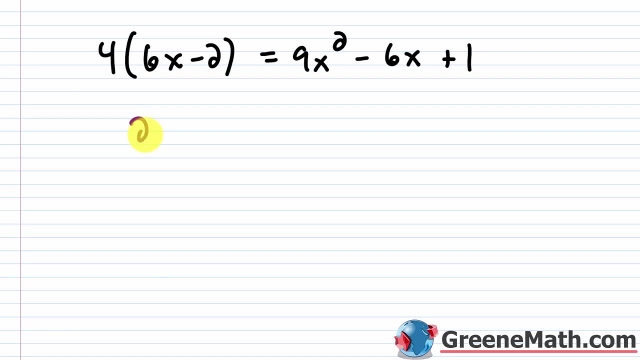 1 squared is 1.. Okay, just using my distributive property, 4 times 6x is 24x. Then minus 4 times 2 is 8.. This equals 9x squared minus 6x plus 1.. What I'll do from here is subtract 24x away from each. 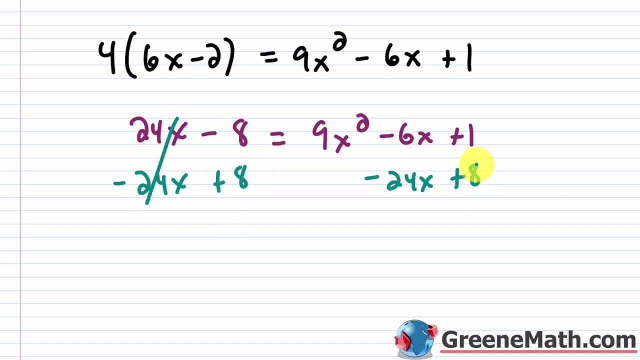 equation. We'll cancel this. I'm going to add 8 to both sides of the equation. We'll cancel this. Let's say this is 0 over here. I'm just going to flip this around and say it's 9x squared. 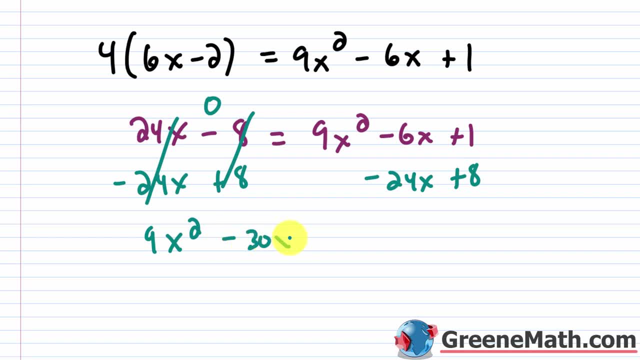 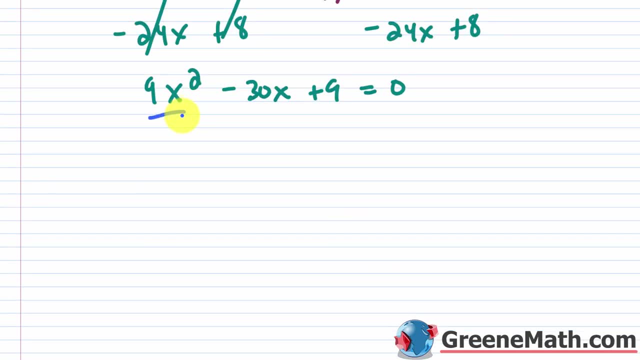 Then basically negative 6x minus 24x is negative 30x. Then we'll have 1 plus 8,, which is 9.. And this equals 0.. Okay, so definitely something I'm going to solve using factoring. You can divide. 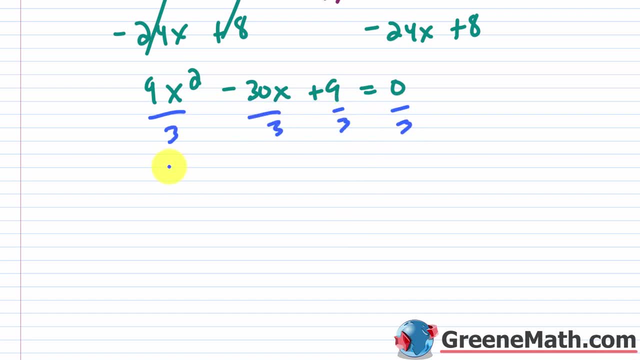 everything here by 3, if you want to make it a little bit easier to work with. So this is 3x squared, Then minus 10x, Then plus 3 is equal to 0. And so really easy to factor this: This is 3x and this is x, And then basically 3 is only 1 times 3. 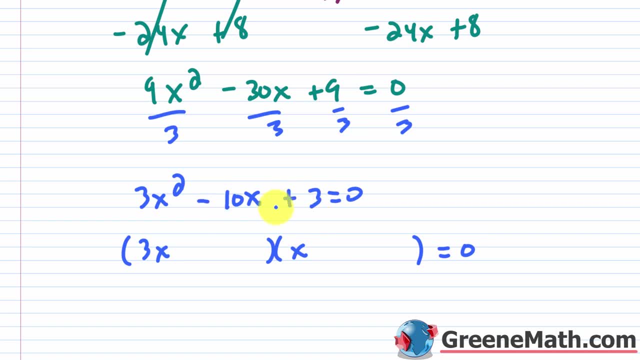 or negative 1 times negative 3.. Now this is a negative and this is a positive. So this is basically going to be a negative and a negative. Now the 3 can't go here because you'd have a common factor of 3.. So it has to be a negative 1 here and a negative 3 here. That's really the 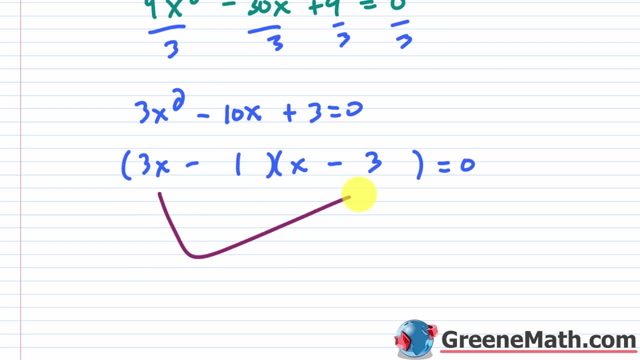 only possible choice, given all these conditions. Well, this would be negative 9x and this would be negative x. Negative 9x minus x would be negative 10x. So we are going to have a negative 9x minus x. 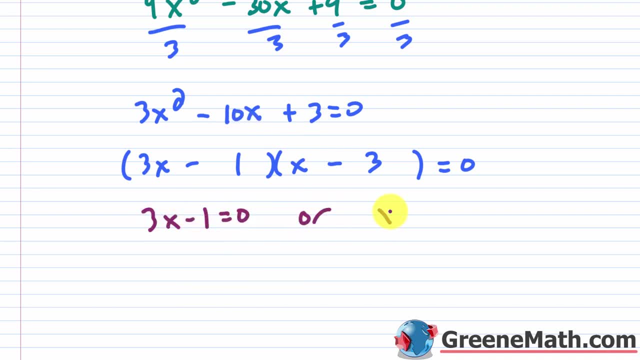 Good to go. Let's go: 3x minus 1 is equal to 0.. Or let's go: x minus 3 is equal to 0. And then I'll add 1 to both sides of the equation. Cancel this. We'll get: 3x is equal to 1.. Divide both sides by: 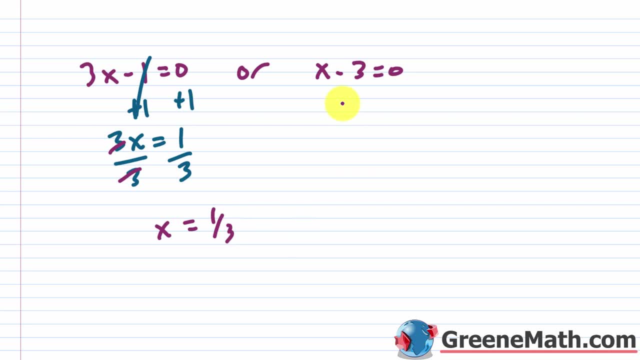 3. Let's cancel this away and say x is equal to 1 third. Then over here let's add 3 to both sides. Cancel this, So x could also be 3.. So again, these are proposed solutions. I'll just tell. 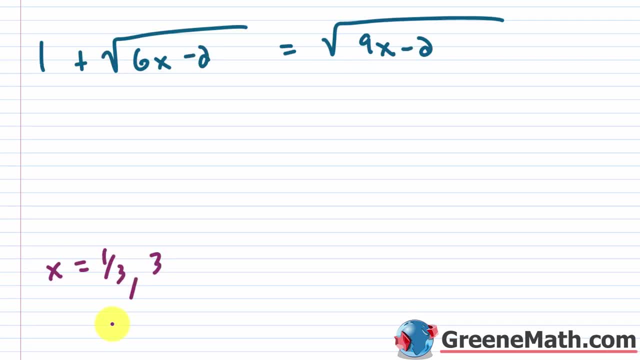 you in advance that they're both going to work. I can plug in a 1 third for x and see if that works, and a 3 for x and see if that works. So we have 1 plus the square root of x. So that's going to be. 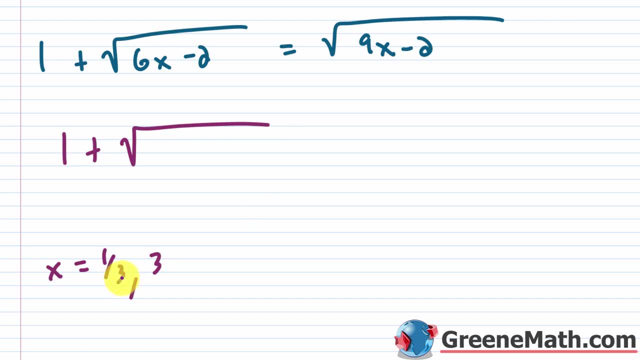 6 times a third would be 2.. 2 minus 2 is 0.. So this is the square root of 0,, which is 0.. So this is just 1.. That should be equal to the square root of 9 times the third is 3.. 3 minus 2 is 1.. 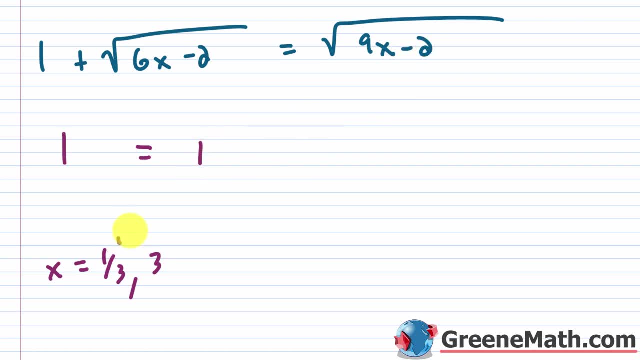 Square root of 1 is 1.. So again, you're going to get 1 equals 1 here. So this one works. Now in terms of 3, I think we could just eyeball this one. So 6 times 3 is 18.. 18 minus 2 is going to. 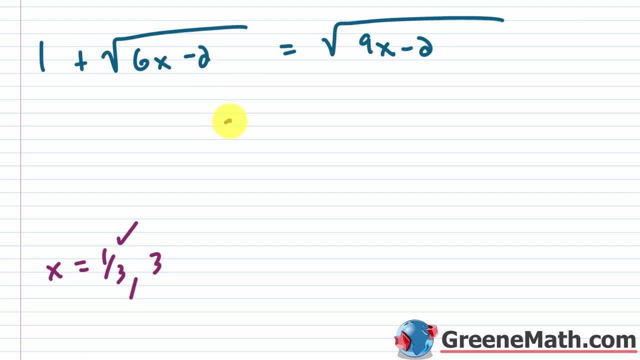 be 16.. The square root of 16 is 4.. So you have 1 plus 4, which is 5.. That equals over here: 9 times 3 is 27.. 27 minus 2 is 25.. The square root of 25 is 5.. So this one works as well. So both of these are. 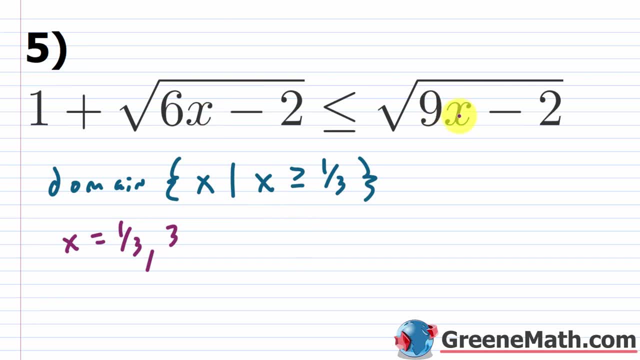 going to work. So let's come back up here. I'm just going to copy this in its current form. So 1 plus the square root of 6x minus 2, we'll say, is less than or equal to, we'll say, the square root. 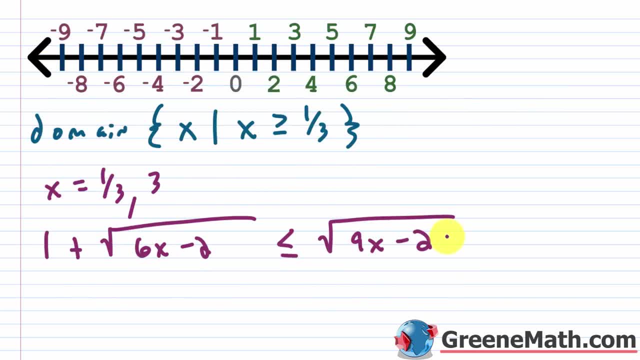 of 9x minus 2.. Okay, so, coming back up here, really we just need to think about 1, third and 3.. That's the only critical values we're going to have. Remember 1, third and 3, those are solutions. 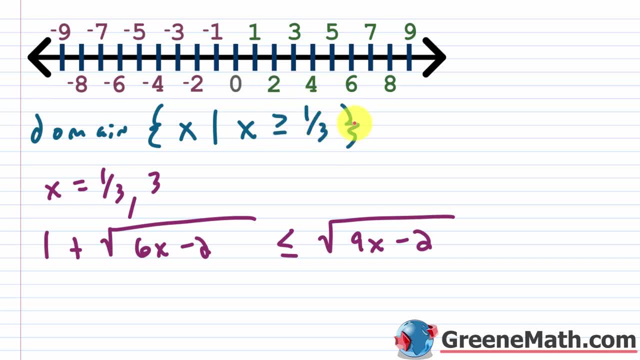 But then also with 1 third. if anything is less than 1 third, it can be 1 third or greater, But if it's less than that, we're going to reject it. So let's find 1 third. Let's just say it's about. 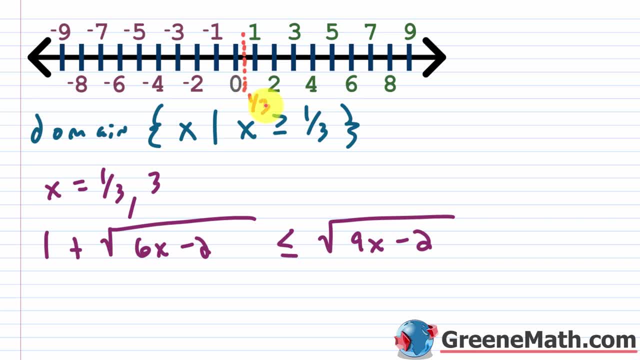 right here. I think that's probably close enough. Let's say that's 1 third, And then for 3, that's right here, And basically we can set up our regions, or you can say intervals or whatever you want to say. So this is A, this is B and this is C. So A is going to be anything, that's. 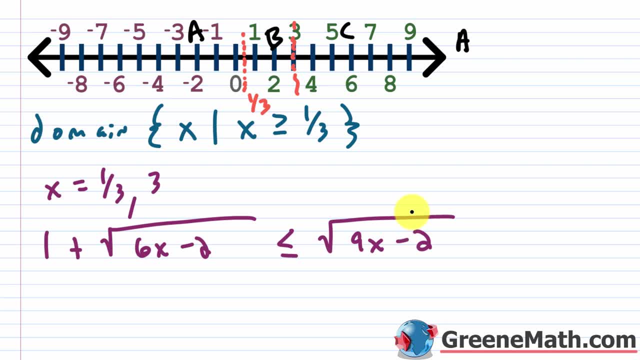 less than 1 third. So we already know that that violates the domain, because X has to be equal to 1 third or greater. So this is an automatic reject. We'll say this is false. Now B and C are open. We don't know. So for B we have to test. that's between 1 third and 3.. 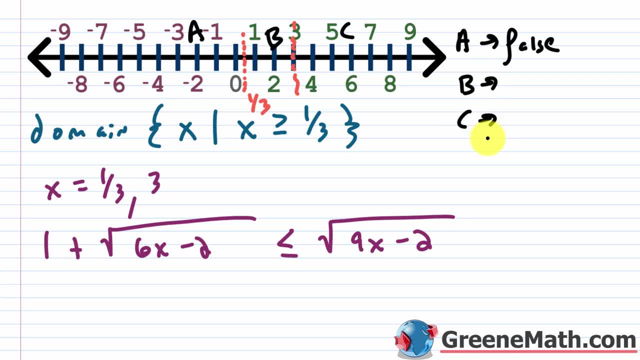 And then for C we have to test that's greater than 3.. So let's check that real quick. So let's think about something like maybe 2 or you could use 1, whatever you want to do, Let's just use 1.. I think that might be easier. Let's see if this works. So 1 plus the square. 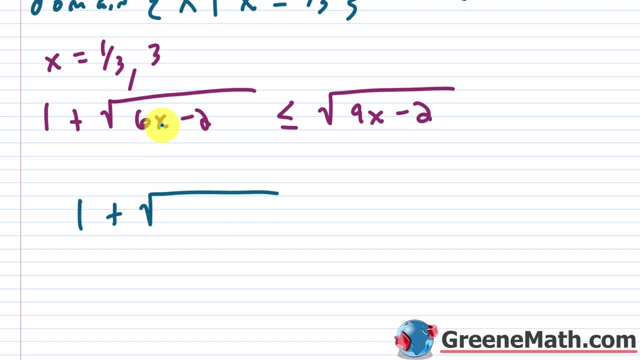 root of, you'd have 6 times 1,, which is 6.. And then minus 1,, which is 6.. And then minus 1,, which would be 4.. So the square root of 4 would be 2.. So this over here would be 1 plus 2 or 3.. 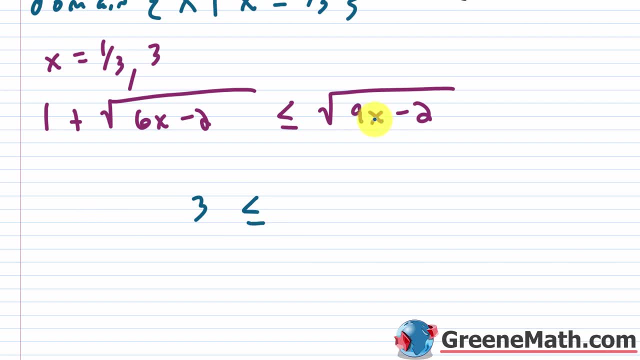 So let's put this as 3.. This is less than or equal to, 9 times 1 is 9.. Then minus 2 is 7.. So this would be the square root of 7.. Now, this is something you could just punch into your calculator. 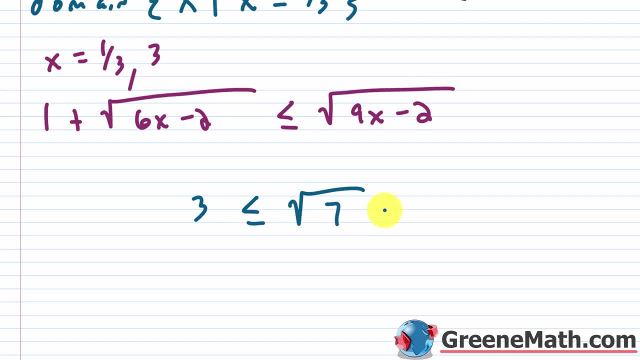 The square root of 7 is about 2.65.. So this is going to be false. This is not going to work. Let's come up here and say this is going to be false And I'll just say this is going to be true. 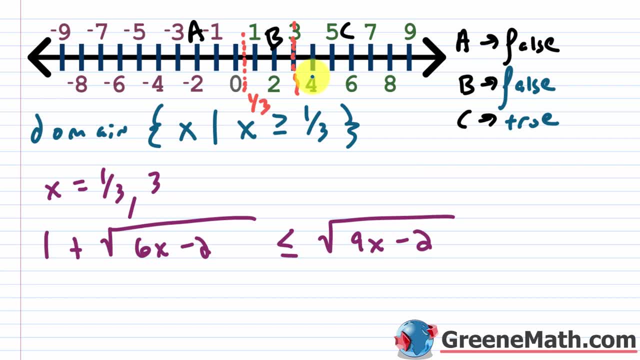 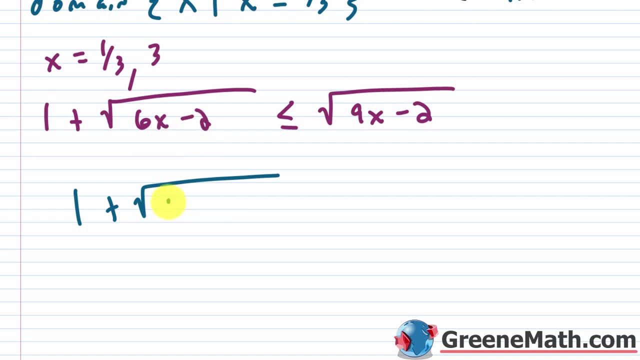 And I'll prove that to you. Something like: let's just say 4.. That won't be that bad. So let's say 1 plus the square root of 6 times 4 is 24.. 24 minus 2 is 22.. This should be less than or equal to the square root of. 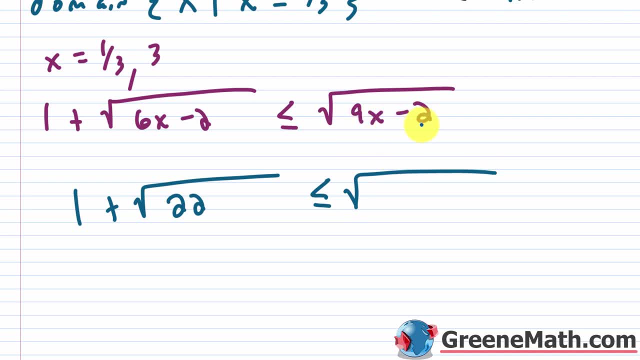 9 times 4 would be 36.. And then 36 minus 2 would be 34.. So again, this is just something you could punch into your calculator: 1 plus the square root of 22.. Let's just say that's about 5.69.. 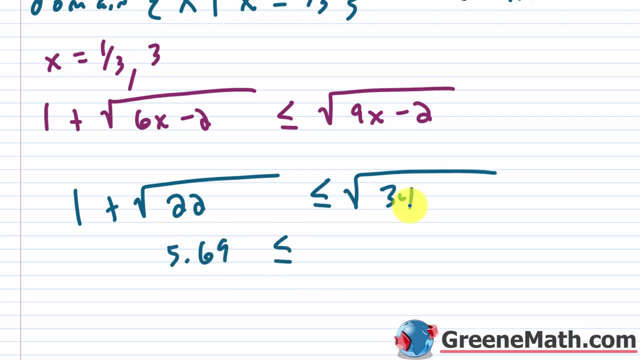 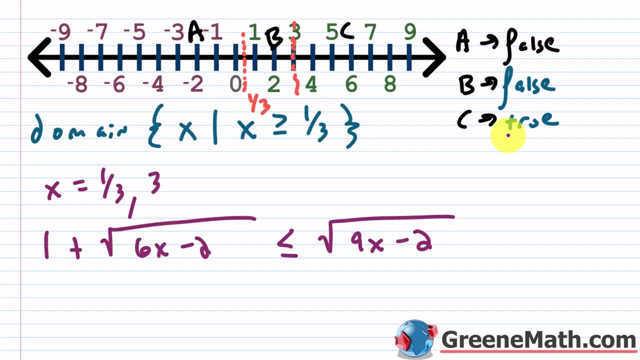 Again, it's an approximation. Is this less than or equal to the square root of 34?? That's about 5.69.. 5.83.. So this is a true statement. So let's think about our solution now. So we're going to start. 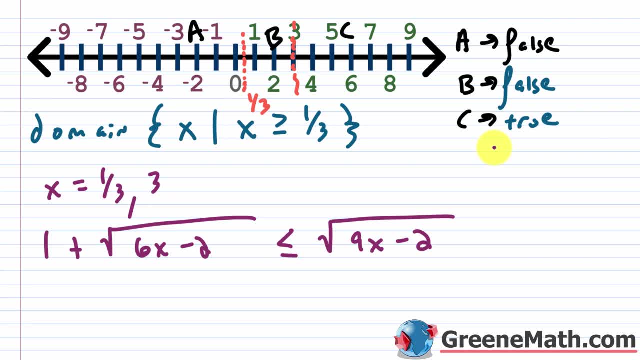 with region C. So for that it's anything that's greater than 3.. So x is greater than 3.. Now is 3 itself included. Remember, 3 is a valid solution to the related equation. So if I plug, 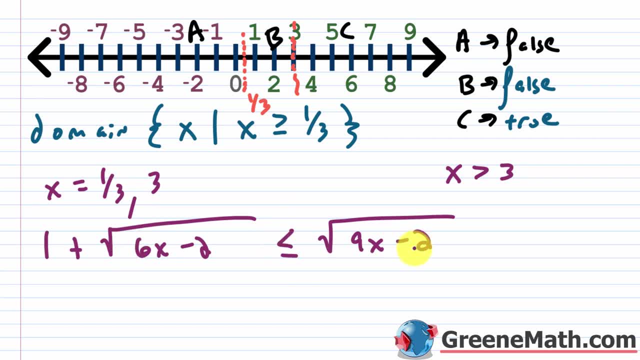 it in. I get the same value on the left as I get on the right. Now, keep in mind here: this is a non-strict inequality, So 3 will work. So we're going to say x is greater than or equal to 3.. 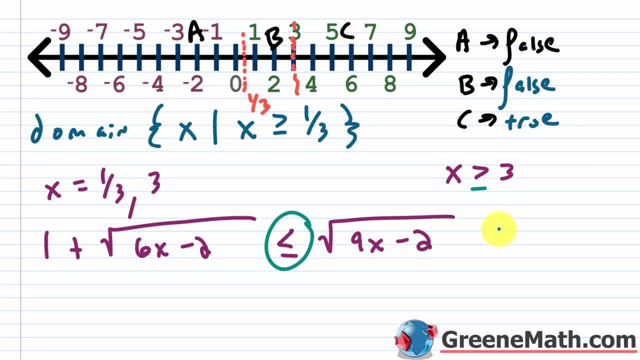 But there's another thing you have to do. Remember we said that 1 third would work as a solution as well, And this is a non-strict inequality, So we have to make sure that we include it. So these are the types of things. 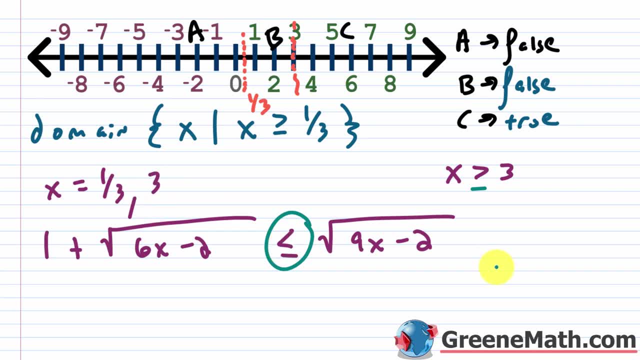 that you can miss pretty easily if you're not thinking about checking all these things. So I would put that x is greater than or equal to 3.. Then you would just put: or x could also be equal to 1 third, because that would satisfy this guy as well If I plug in a 1 third for x. 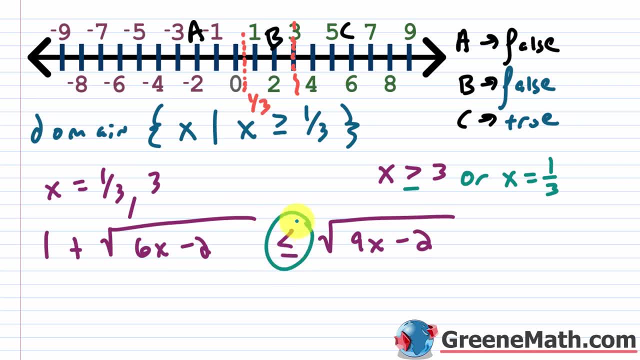 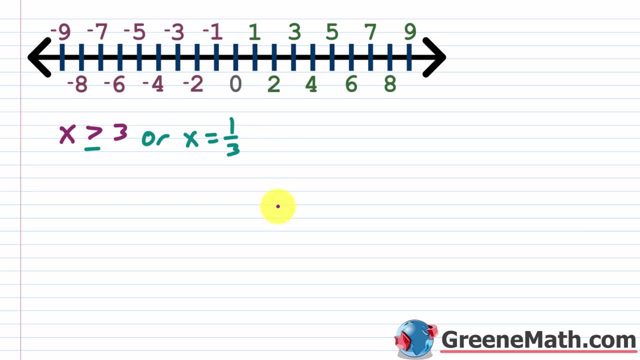 I would get the same value on the left as I get on the right, So this guy would be satisfied. Now, this is going to be strange and interval, But in case you do want to write it that way, what I would do is actually reorder this and say: 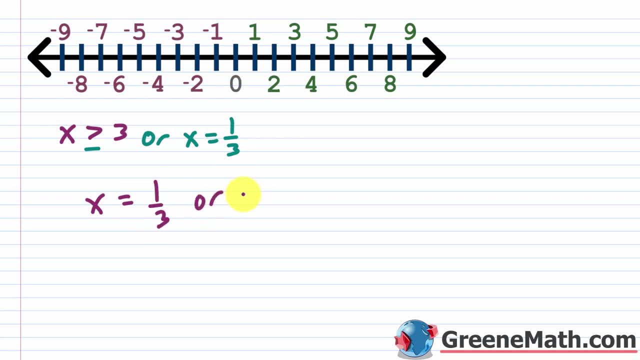 that x is equal to 1 third, And then I'll put: or x is greater than, or equal to 3.. So let me erase this and put this like this, And then an interval notation. What I'll do is basically put a bracket. 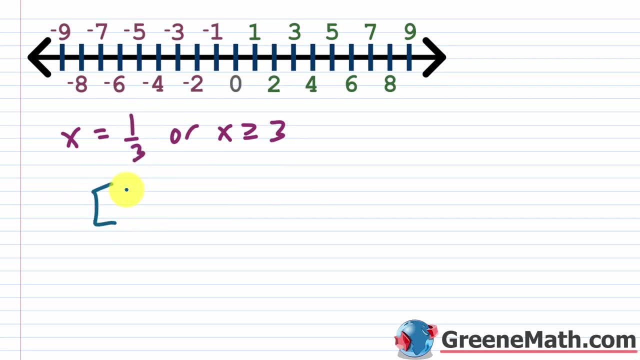 here It's the same number. So how do you write that as an interval? You just put 1 third here next to this bracket, a comma, and then 1 third here next to this bracket, And I know this looks really, really weird, but that's just how you do it. So I'm going to put 1 third here next to this.